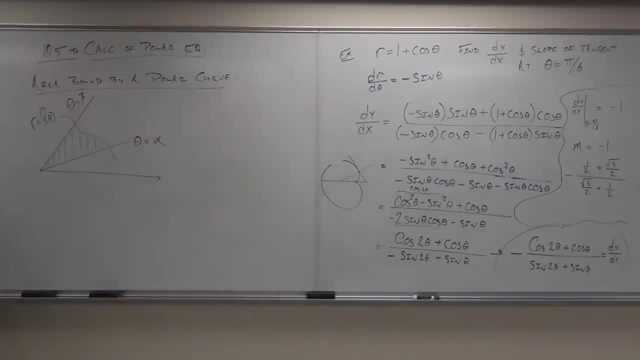 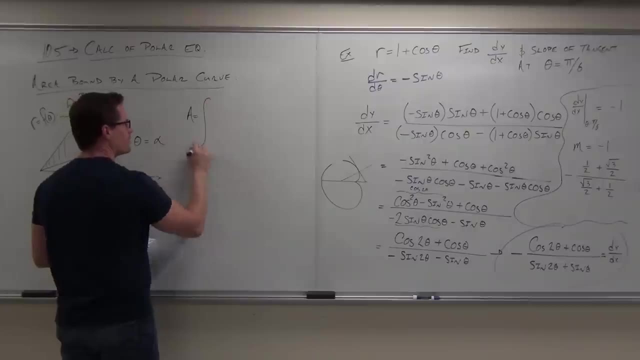 it's more like a sector. We're going to talk about that in a second. So here it is how we find the area. I'm just going to give it to you and you're going to see why. it's going to be very straightforward right now. Here it is. Now these functions are they based? 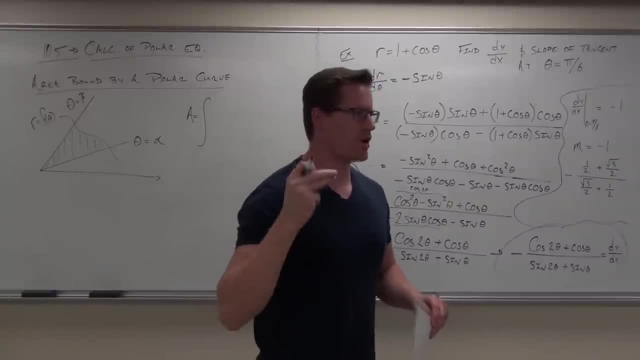 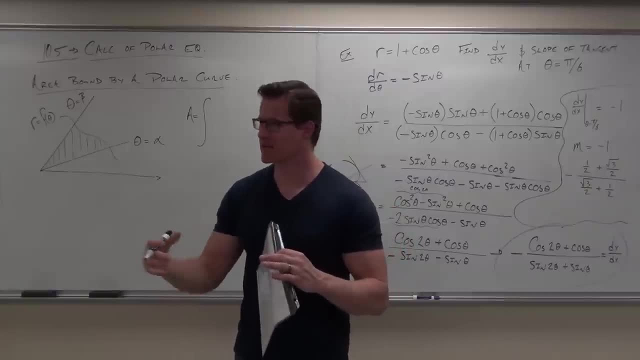 of stuff. We're going to talk about what slices we're adding up in just a second. I'm not going to prove it for you because I think I can just explain it well enough. If you remember anything about calculus 1, when you do integrals, the Riemann sums that you added. 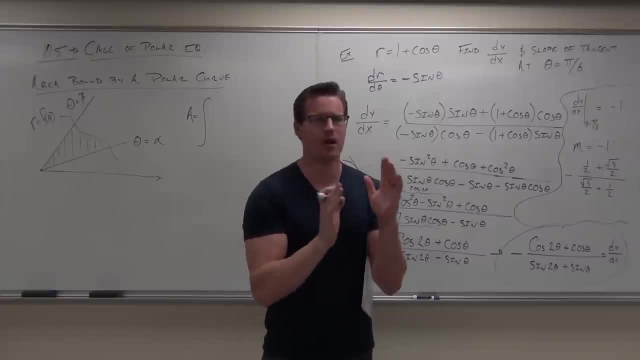 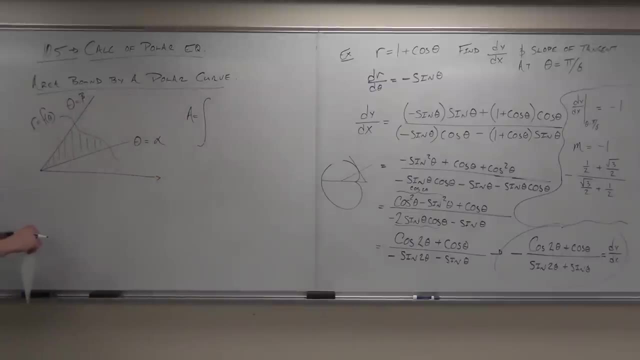 up. they were little slices, little rectangles. Remember that. Add up an infinite number of them. We're going to get the same idea. That's what integral does: It adds stuff up. So here's what we're going to add. We're going to say: well, where do we want to start If it's not? 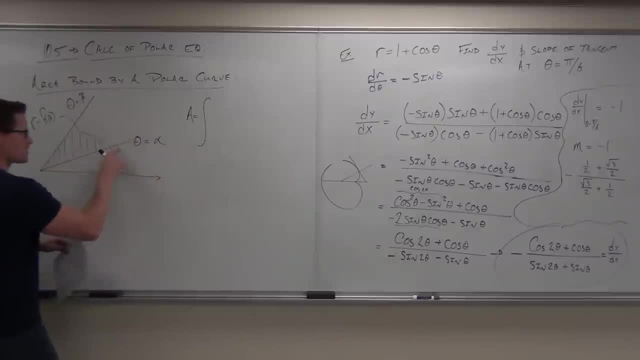 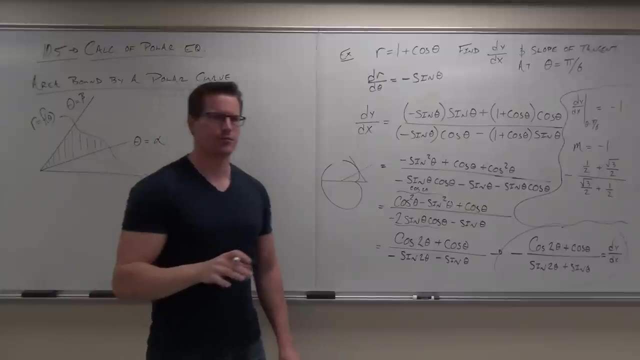 X and Y. we've got to start at some alpha, So we're going to start here, We're going to end at beta And we're going to have. here's what we're going to have. If you think about this, what we're really doing- 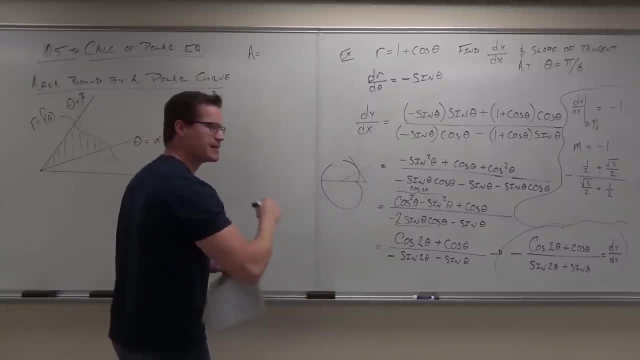 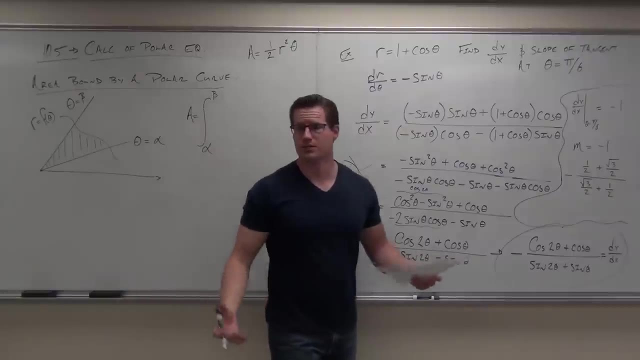 is, we're finding the area of a little teeny sector. The area of a sector is given by this. If you've seen that before, that's the area of a sector. It's 1 half r squared theta. You can look it up. 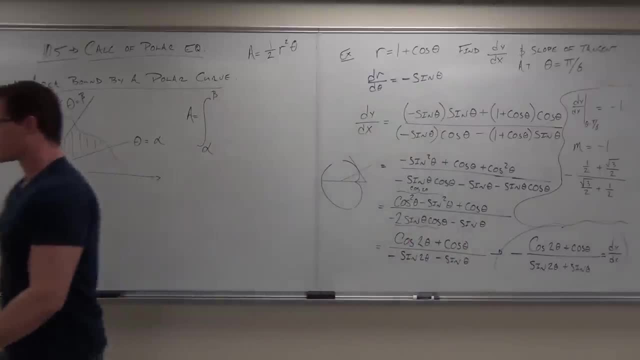 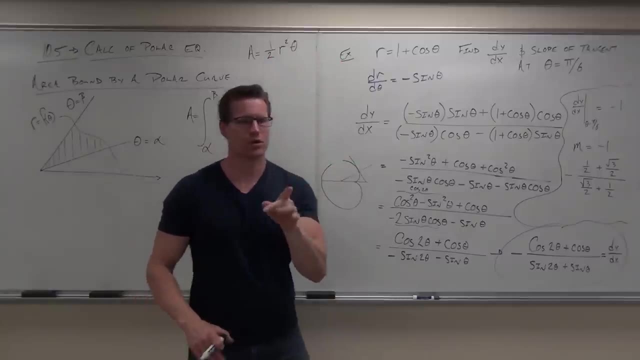 It's a formula. I'm not going to go through the proof of that formula. That's the area of a sector. It says: take half the radius squared and then multiply it by whatever angle you have. Well, here's what we're going to do. 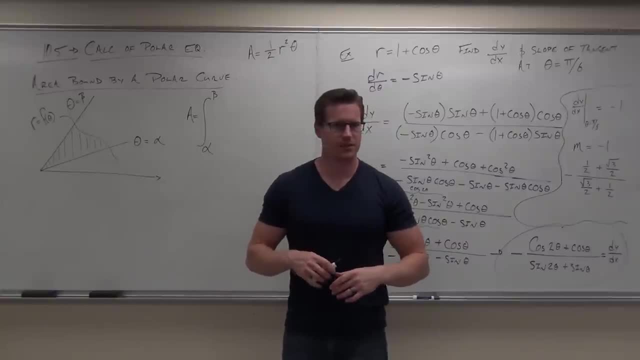 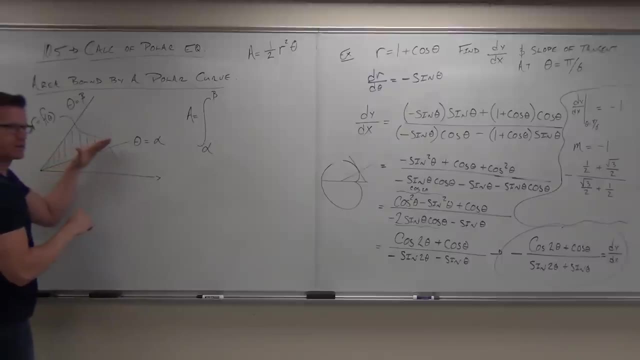 Are you listening Now? r is a function of theta, isn't it So for us? it says: what we're going to do is we're going to take a real teeny little sector of this thing, a teeny little one. 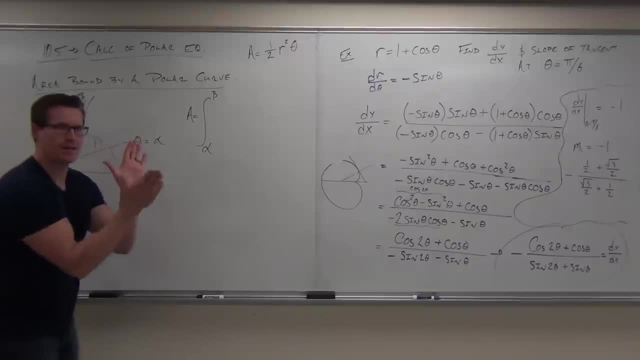 And then we're going to find the next one, and the next one, and the next one, and the next one. We're going to allow that distance, that angle, the distance of the angle between them, to go to 0. And if that's the case, we're going. 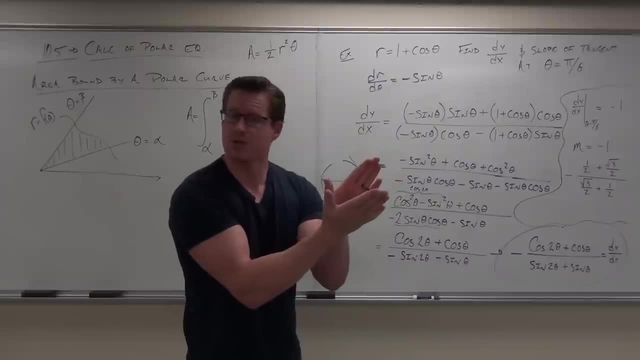 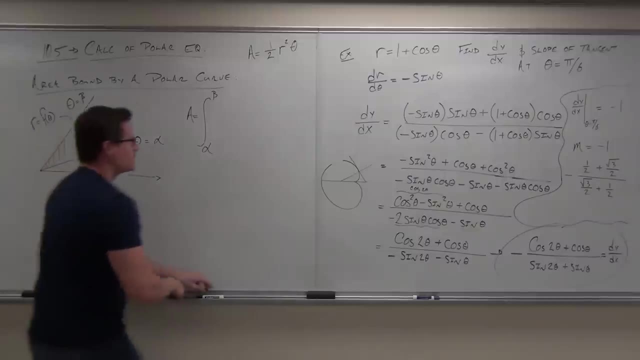 to have an infinite number of teeny little sectors that we're going to add up. So when we're saying we're starting alpha, you're going to have all these sectors starting alpha adding up to beta And we're going to say, all right, cool. 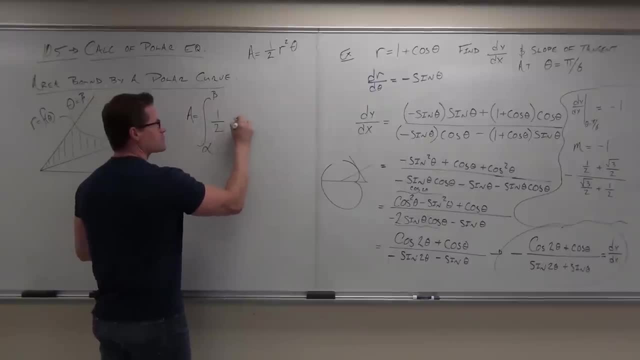 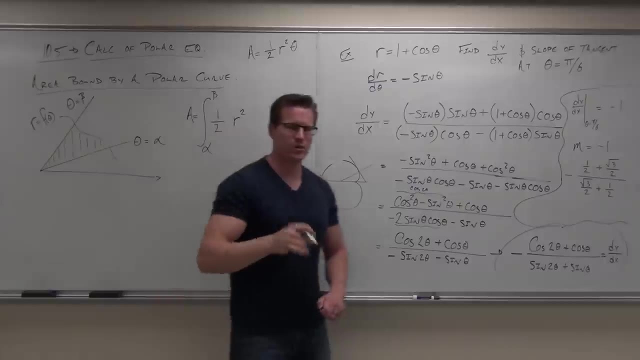 Well, we're going to have the 1 half. We're going to have a function. We're going to let r change based on theta. r is a function of theta, But then we're going to integrate with respect to theta And the reason why we integrate with respect to that variable. 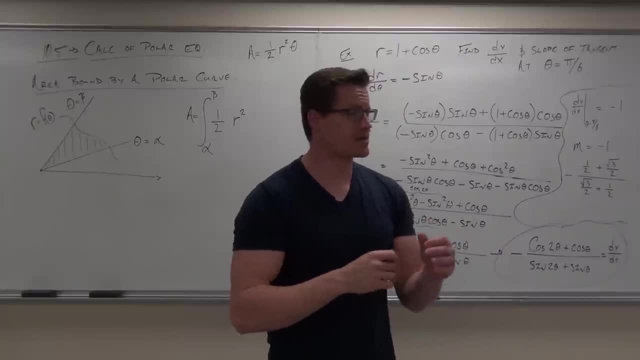 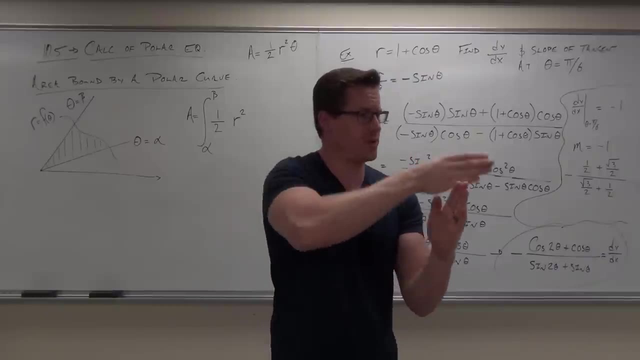 is because when you integrate that like a dx, that's saying that dx, the distance between the x values are like infinitesimally small, giving you an infinite number of rectangles. when you do a basic area For us, it says we're going to do d theta, saying 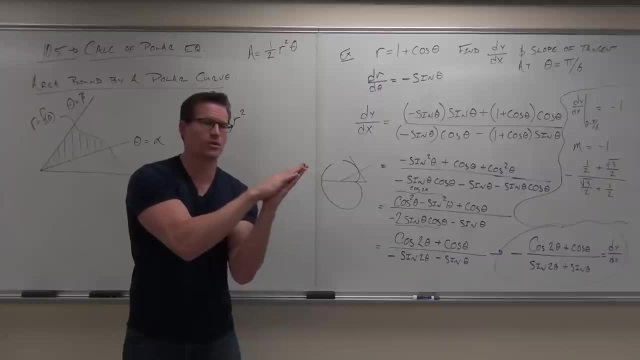 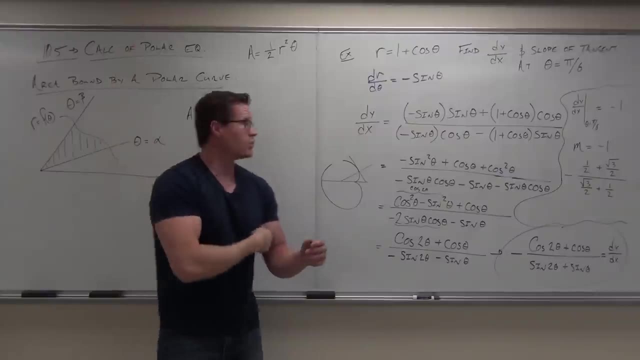 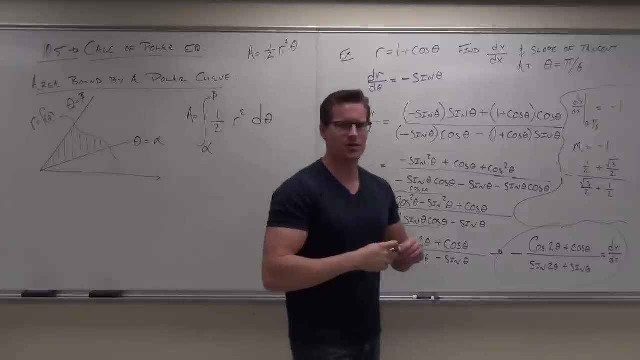 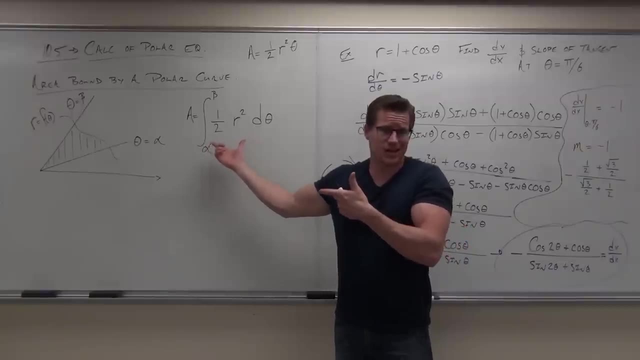 Chirp, chirp little crickets. Where's that coming from? Area of a sector. Do you guys see the area of a sector I'm trying to show you here? This is the area of a sector. You're just allowing the angle to change. 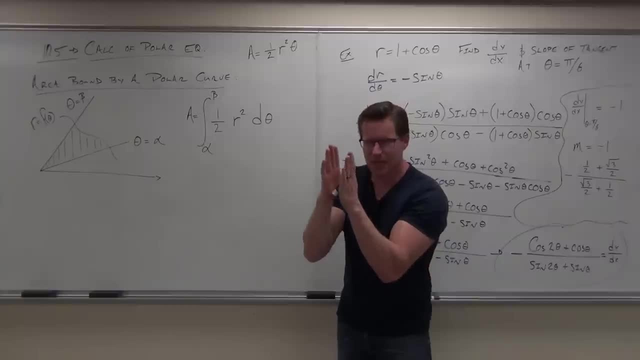 That's all you're doing here. Make sense. It's cutting this into really little teeny sectors, adding up the sectors from alpha to beta. So this is adding up. Remember the integral is like an s, It comes from a summation notation. 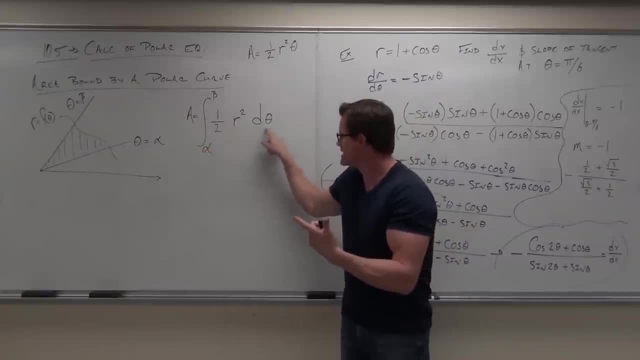 So the integral is: we're adding up all the teeny sectors. teeny sectors here See it: Yes, Teeny, teeny sectors, adding from alpha to beta. That's what it means. So let's do an example real quick to illustrate this. 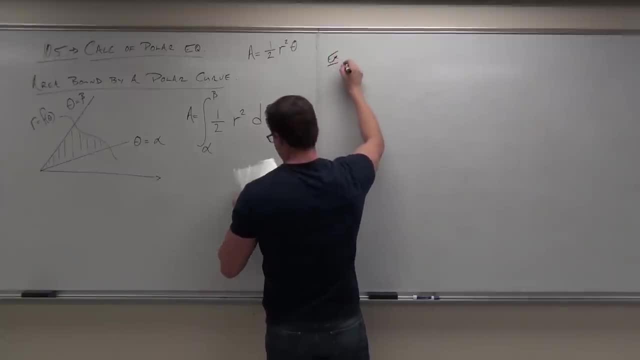 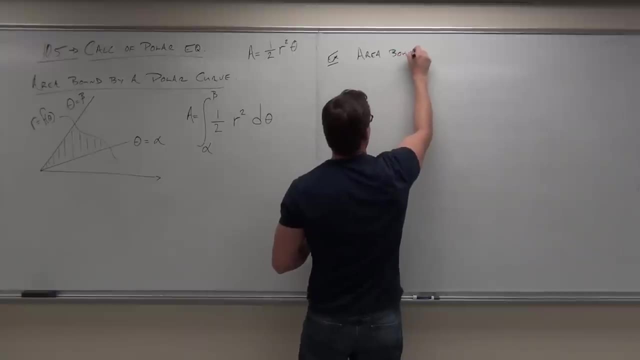 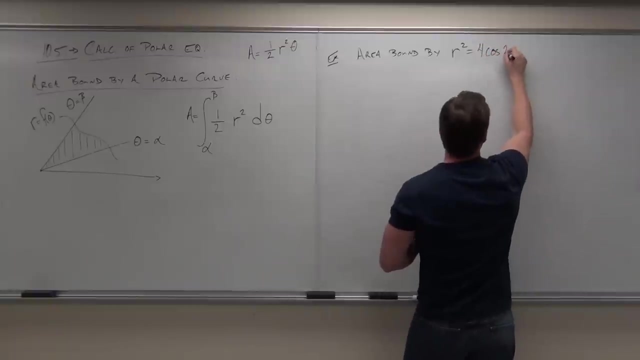 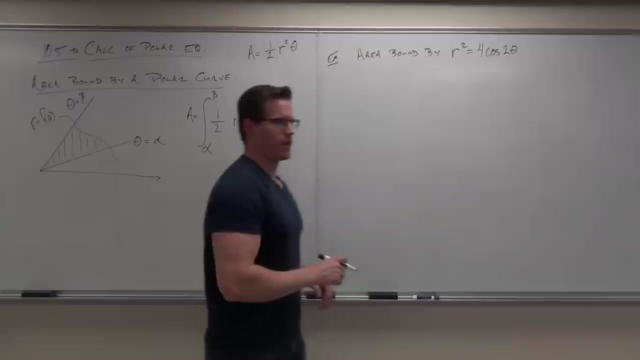 It's better to know where the formulas came from than to not know. So I want to find the area bound by r. squared equals 4 cosine 2 theta, Before you say: what in the heck is that? I don't even know where to go. 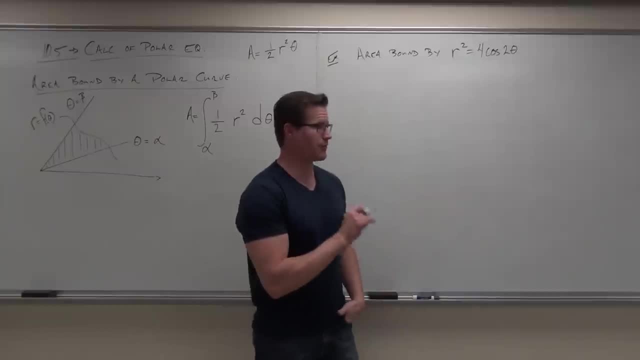 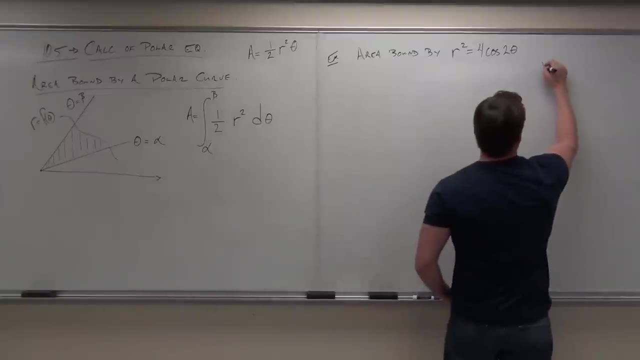 We've seen this before. In fact, in the last section, we graphed that It didn't look exactly like this. It looked like this: It looked like r equals the square root. I messed up already. It looked like this. 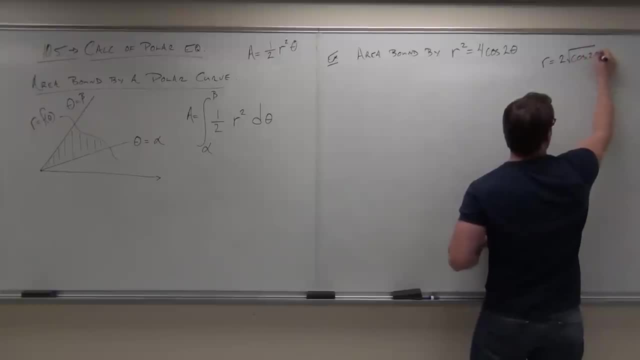 r equals 2 square root, cosine 2 theta. Is that ringing a bell at all? Yeah, That was the last example that we graphed, all right. So what this graph looks like- and you could probably just see it if you thought about here- 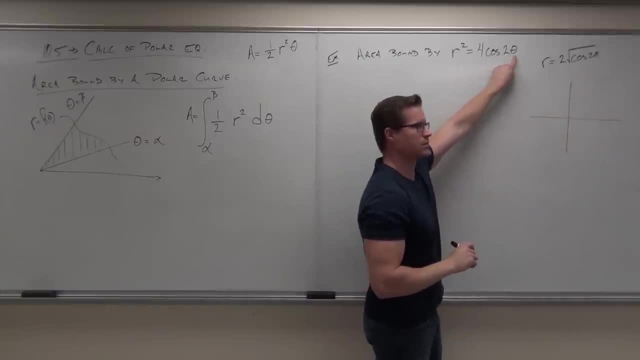 If I plug in 0, look at this: If I plug in 0. It's 2 times 0. OK, good. And then cosine 0. And then 1 times 4? 4.. And then take square root of that. 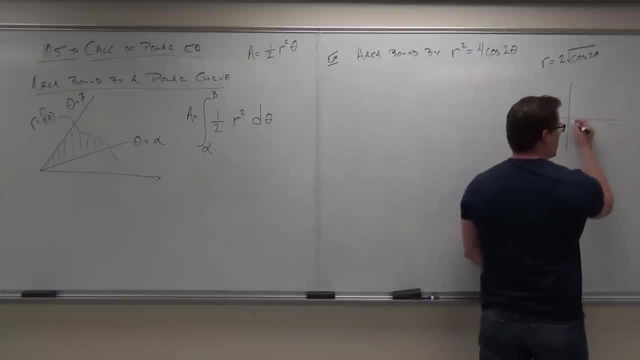 2. Or squared. So if I do an angle of 0, I got 2.. Remember that at all? Yes, And I plugged in pi over 2,, pi over 4.. Yeah, 2 times pi over 4?. 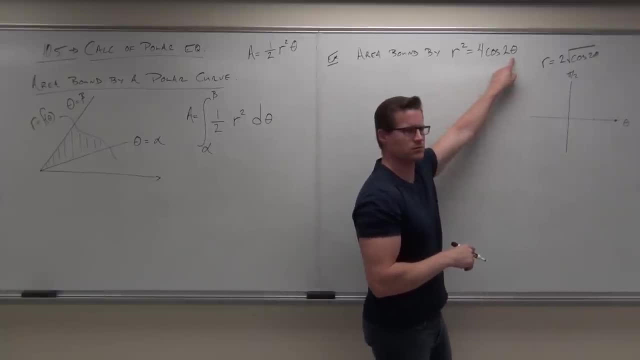 2 times pi over 4.. Hm, Say it again. Yeah, you're right: Pi over 2.. Cosine: pi over 2? 0.. 0 times 4? 2 pi over 4.. r squared. 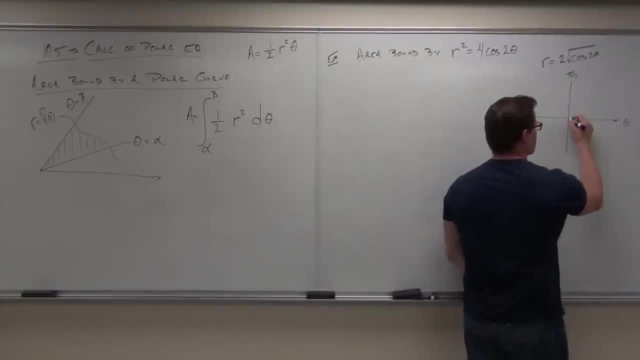 r equals 0.. So we got to here And we learned about the symmetry. We learned that anything past pi over 4 was undefined. Do you remember that? So we said, OK, well, that can happen. So what we got really was this shape that we got. 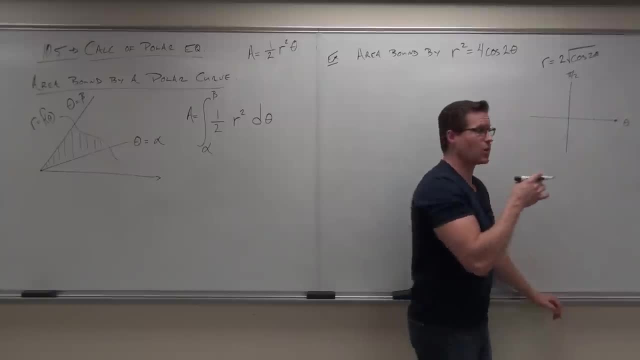 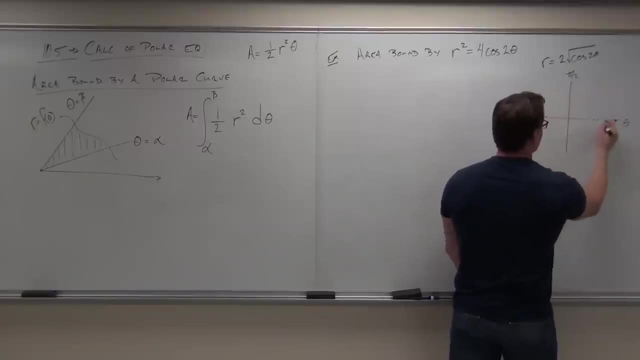 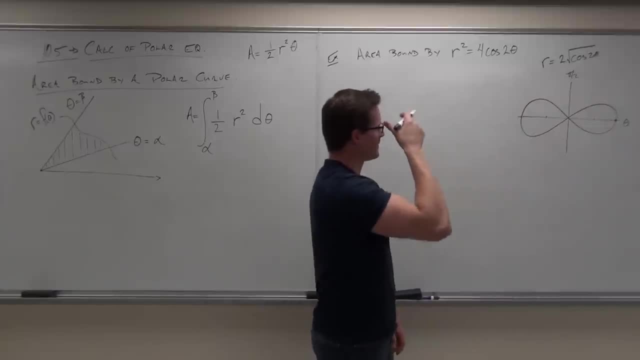 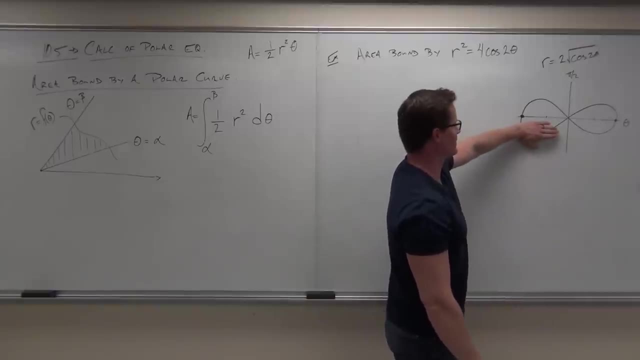 Upterm. I know right, That's pretty good. They said: just don't look at that one. Well, here's the deal As we know. that's what that looks like and we know about the symmetry. I'm not going. 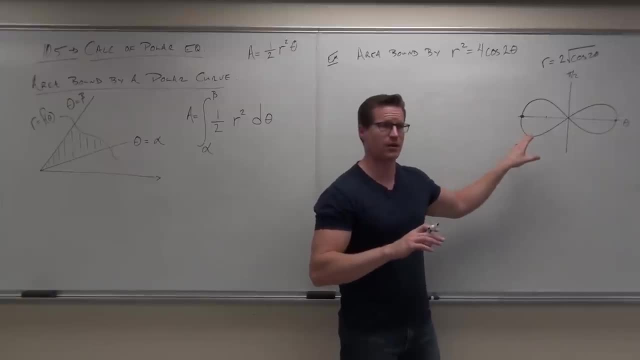 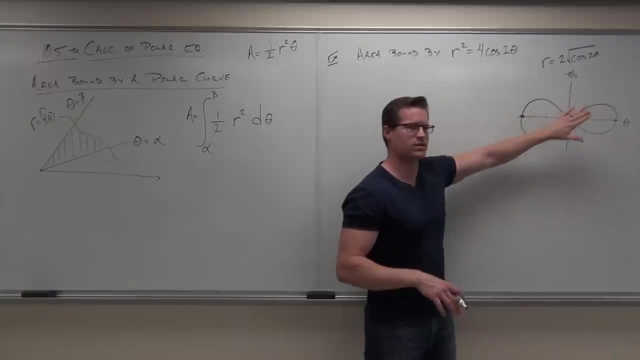 to reinvent the wheel. OK, If you want to figure out how to actually graph that thing, well, you watch the last section. OK, We've already done this. We know it's symmetric about the polar axis. We know it's symmetric about the theta equals pi over two. 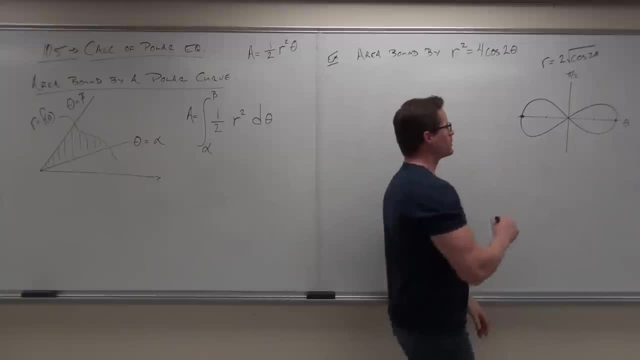 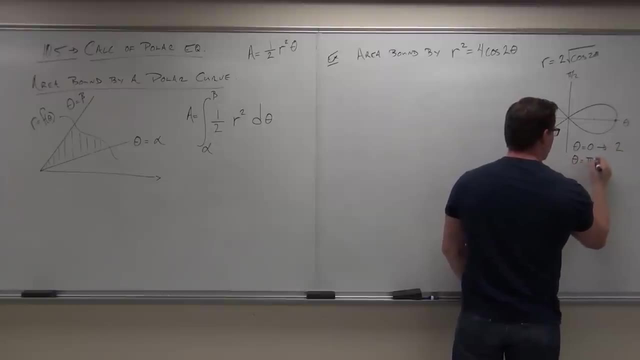 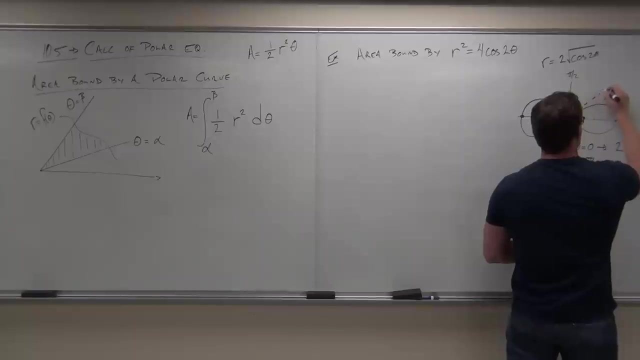 axis, you with me. So let's think about this: When we plugged in, theta equals zero, it gave us two. When we plugged in theta equals pi over four, it gave us zero. Does that make sense? So our angle, our angles, go from zero to pi over four. 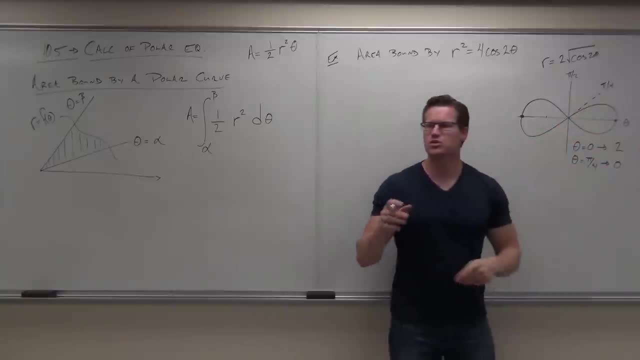 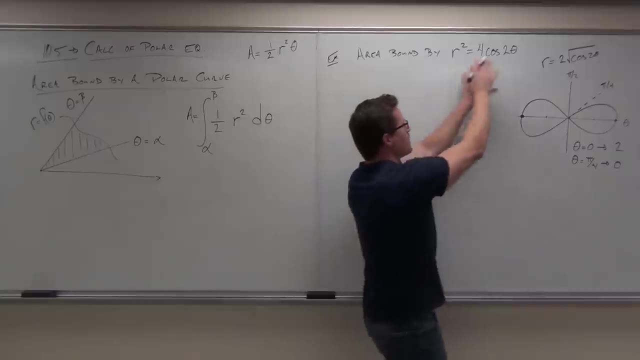 and it gives us this little lobe right here. It gives us that lobe. Now let's use that to our advantage. If we use it to our advantage, well, let's set this thing up. I want to find the area bound by this curve. 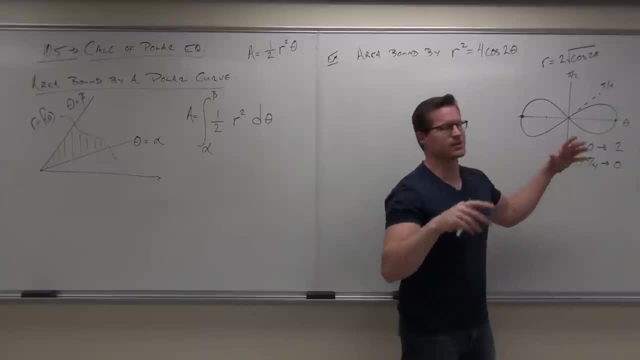 What that means is all of this stuff. Do you understand? It does not look like it from my picture, but you get that. this and this and this and this are all the same area. How many pieces are there? Four. So if we integrate, 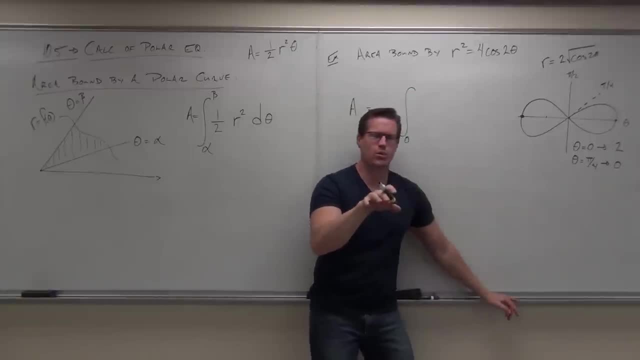 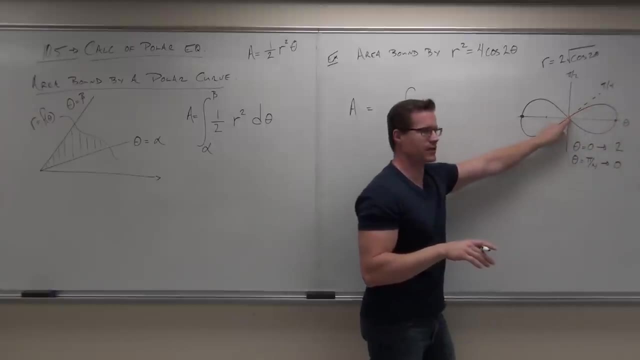 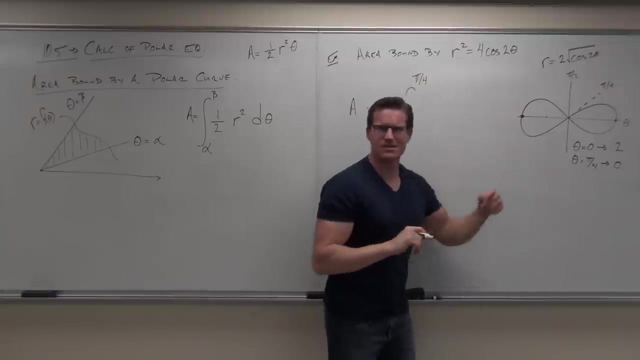 from zero. where do I want to go? Zero to where? Pi over two, Pi over four, Pi over four moves me from here to here. That's where I want to go. So if I did zero to pi over four, how many pieces is this going to give me? 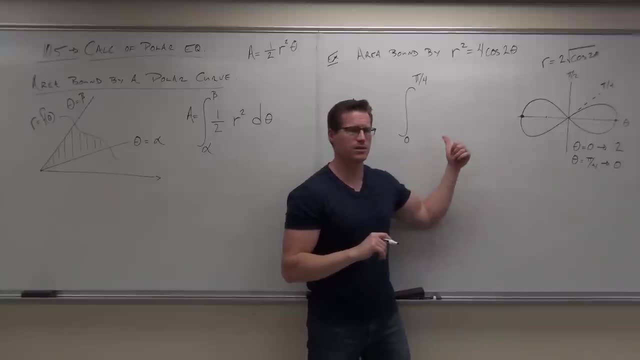 from zero to pi over four. Four, No, from zero to pi over four. it's giving me just this piece. What do I have to do to make all of it Four? Multiply it by four. Show of hands, if you understand that concept. 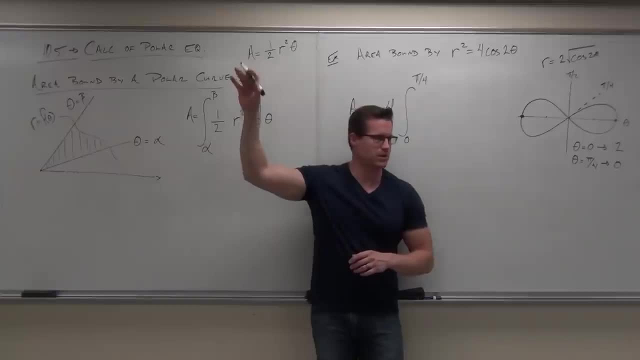 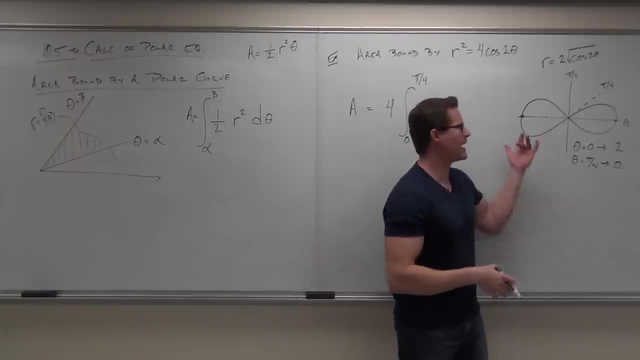 Are you sure? Yes, no, Yes, okay. So we said: I know from probably the previous sections how you'd graph this. You know, you go back there, you figure out how to graph it. I did it very fast here. 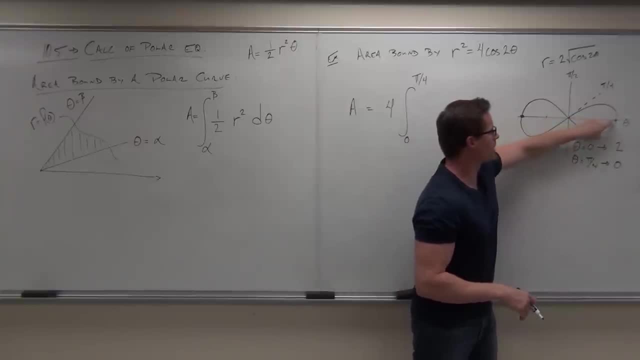 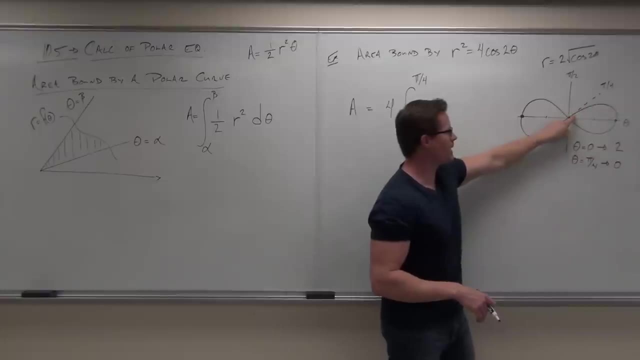 because, for the sake of time, We know that at theta equals zero, I get two. so I'm starting here. At theta equals pi over four, I was at zero. So from zero to pi over four, I get this little lobe. 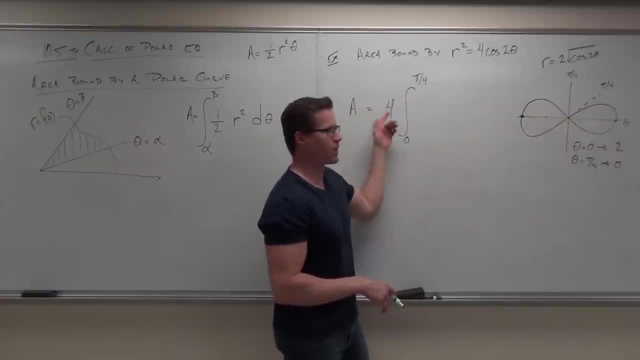 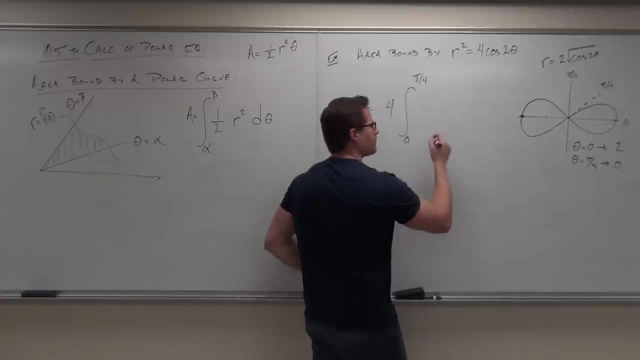 If I multiply one, two, three, four and just go from zero to pi over four, I'm going to have the whole entire area of that shape. You get me Now use the formula. What's our formula? to start with, 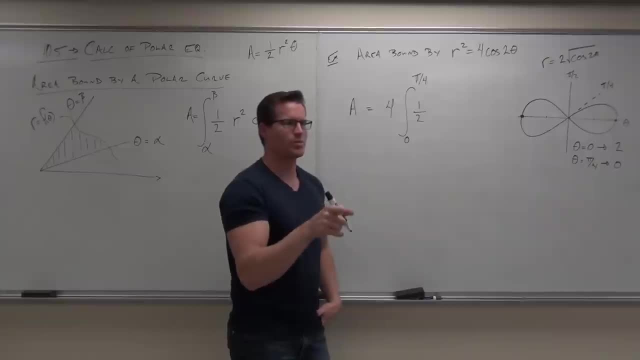 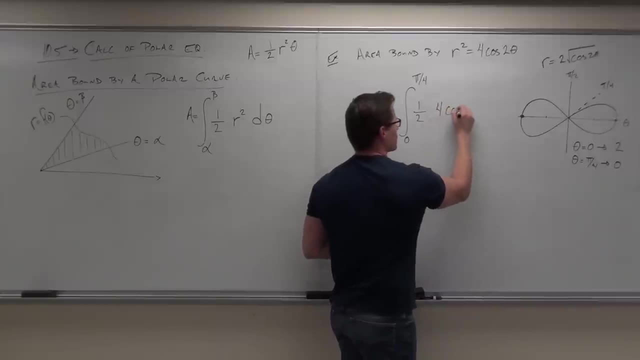 One half, One half, very good. And then R squared. Now be smart about this. Look at, we already have R squared. So if this is R squared, I'm just going to have four cosine two theta. See if you're really just paying attention. 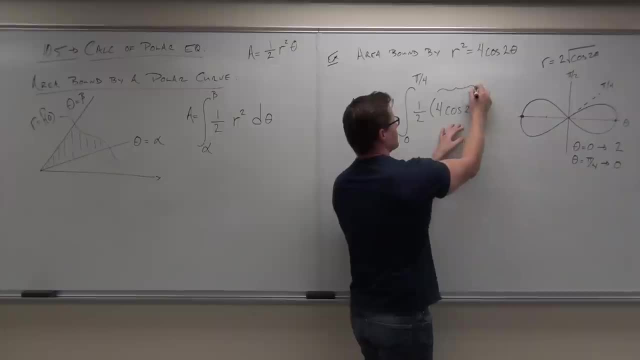 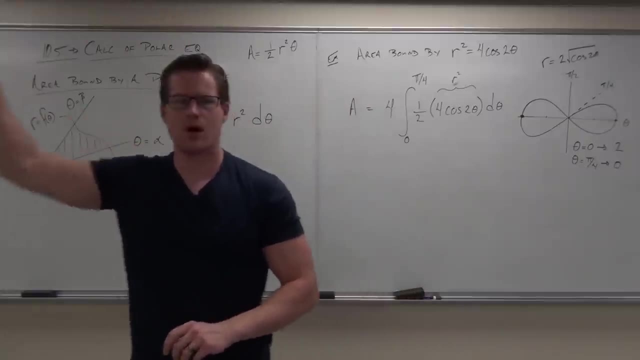 Should I square that, yes or no? No, Because this is R squared. And then d theta. Wrap that thing up with d theta. Show of hands, if you feel. okay with that one. Okay, let's make this thing nicer. What are we going to do? 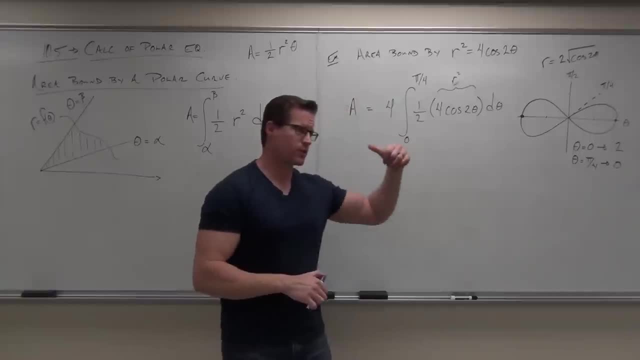 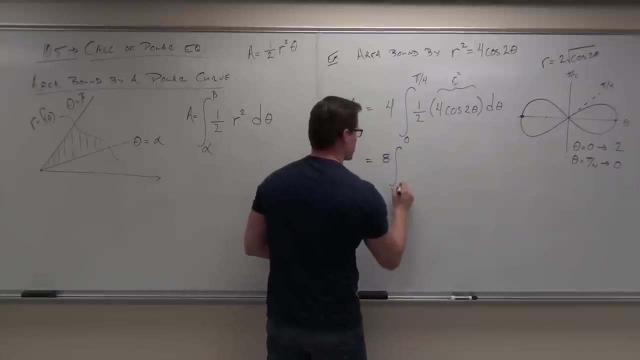 Probably take the one half out. Also going to take the four times one. half times four is We're going to get eight, Eight integral zero to pi over four cosine two theta. Oh my gosh, Have you done stuff like this in this class? 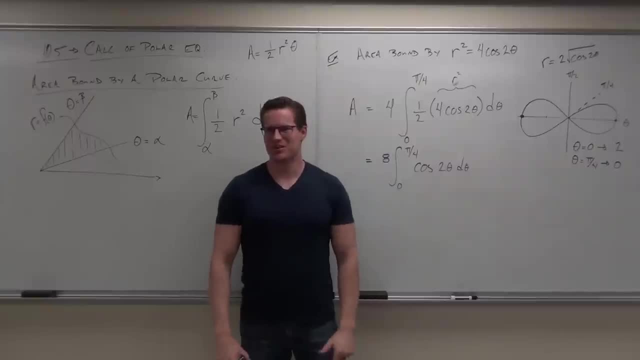 We covered chapter seven. yay, You know how to do integrals of trigonometric. If you wanna do it for functions, do it. What would you use for that? Is it a hard one? It's an easy one. No, it's an easy one. 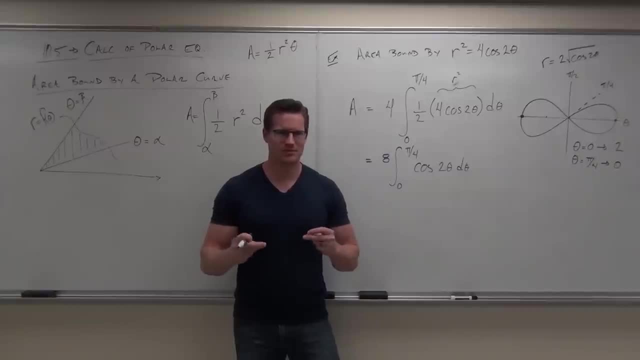 What would you use? What would you use? Substitution? Ah, good, yeah, a? U substitution is what you would U-ze. Yeah, you'd do it. In fact, I'd probably do it in my head, Because at this point you probably can do that. 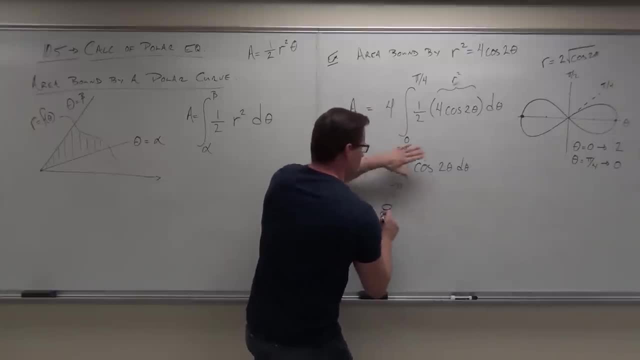 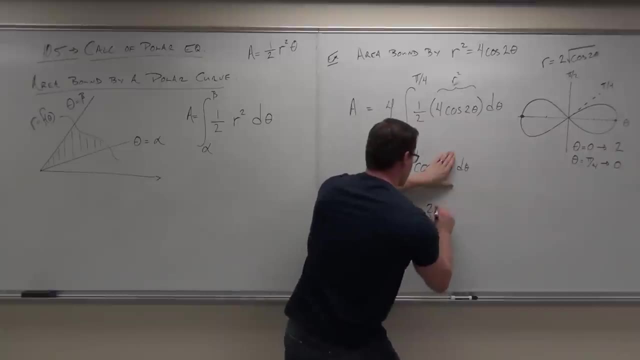 So when I would do this one, I'd say: okay, here's my eight. The integral of cosine is sine. Is that right, not negative sine. verify that Sine of whatever's under my hand divided by the derivative of whatever's under my hand. 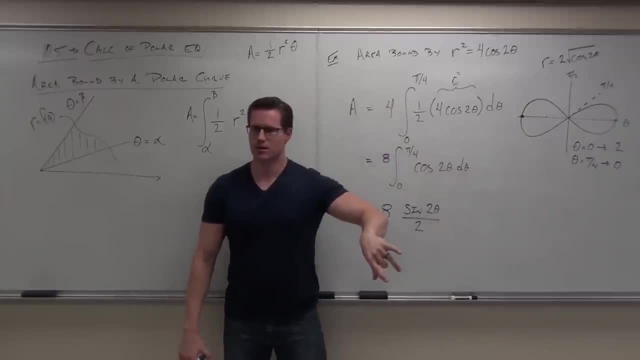 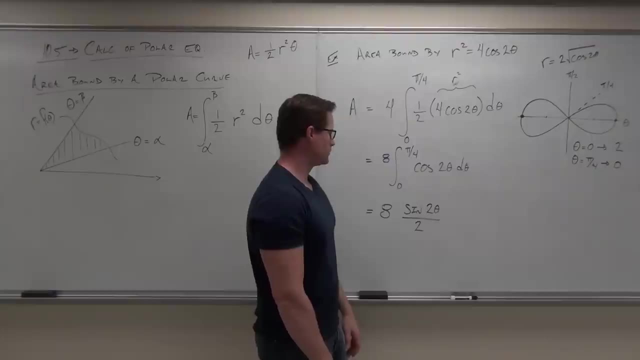 which is just two. The two goes on the denominator. do you understand that? A U sub says hey, take the derivative of that and divide by it. That's basically what we're doing here. What now? Simplify it with the two. 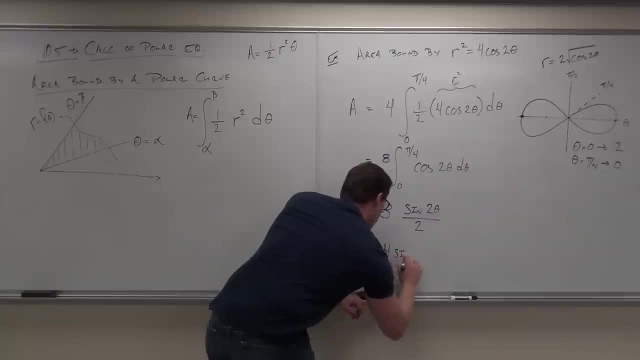 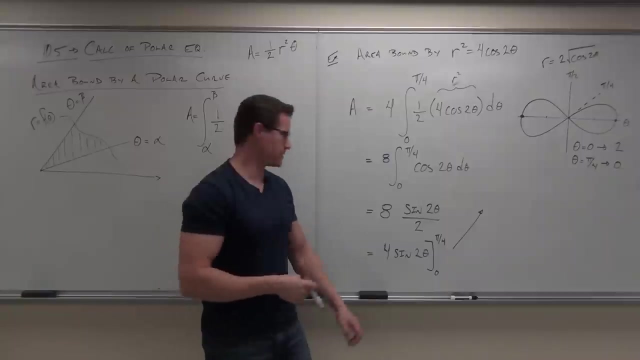 Yeah, let's simplify it. Okay, so we're gonna have four sine two theta. and now what? Yeah, let's go for our actual evaluation: zero to pi over four. Can you plug that in? Hello, yes, no, that should be pretty easy. 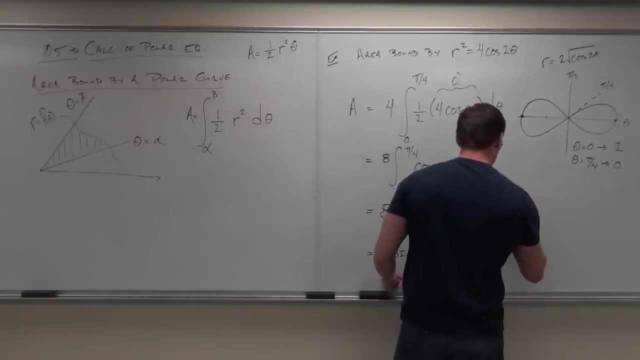 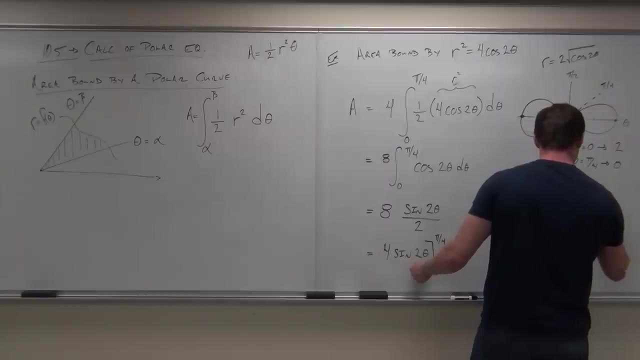 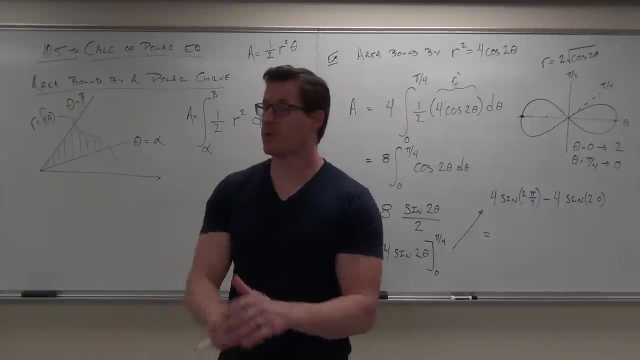 So we're gonna have four times sine of two times pi over four, minus four times sine of two times zero. Well, that should be pretty straight forward. What's two times pi over four? Pi over two? Good, what's sine of pi over two? 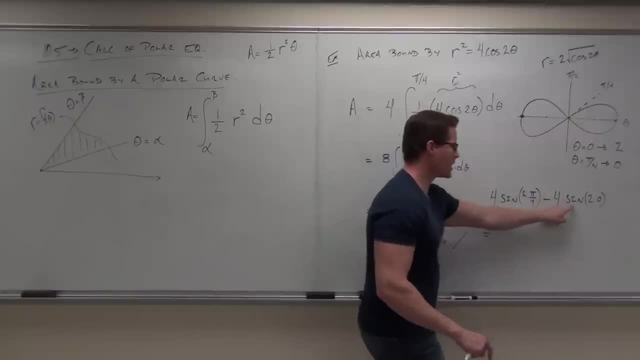 One times four. And what times four is Four? What's sine of zero, Zero? So this whole thing goes to zero, this thing goes to one. we get four times one. What's really, really interesting? the area that's bound by this polar equation. 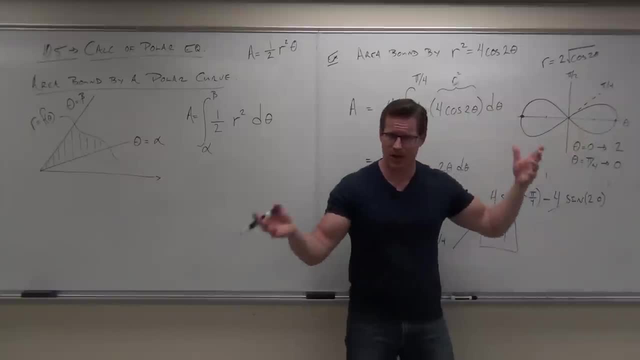 this polar curve is equal to: Does that blow your mind? That it's not some random weird decimal that doesn't end That area's four. that's crazy. What's the area of one of these things? One, One, yeah. 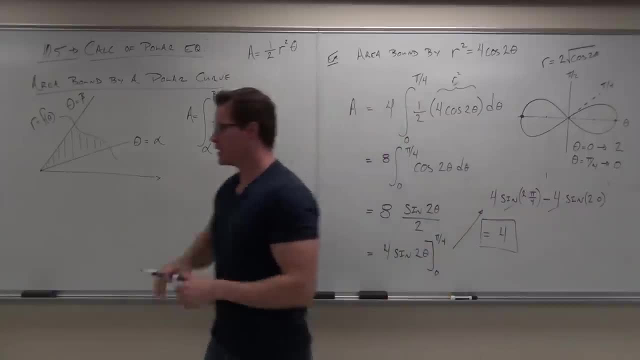 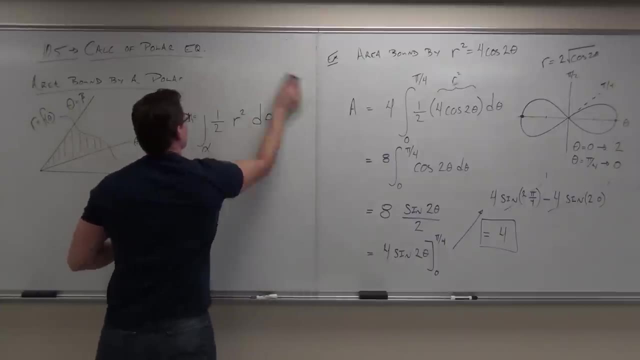 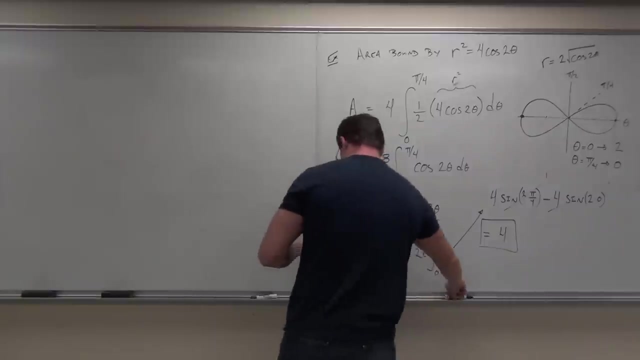 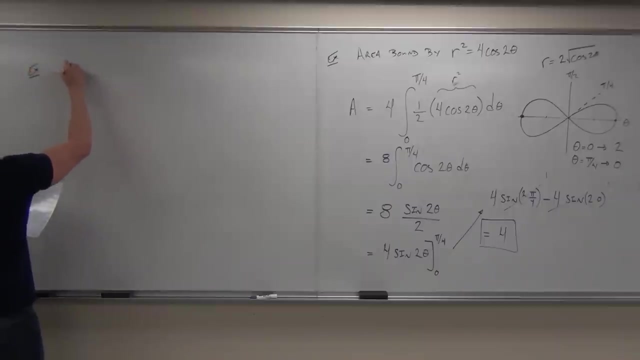 One, two, three, four. That's neat, so I guess we understand that one. Okay, I'll tell you what. let's do one more. we're gonna do as many as we can. So area by r equals one plus cosine theta. 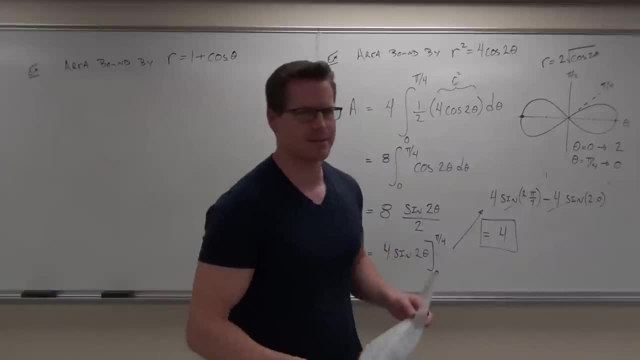 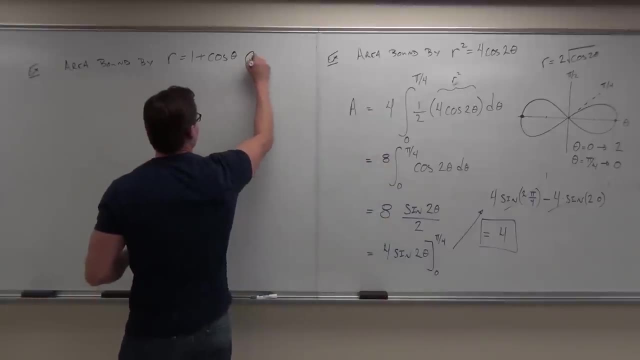 We've seen that several times now. what is that The butt? Come on, I should have said that to you. What is that? Cardioid? It's cardioid, that's right. So you said it was facing up because it's pluses. 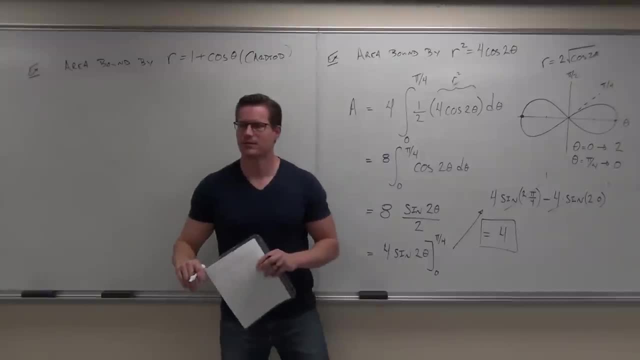 At first I said a heart, you said a butt. It's like the butt's on top or on the bottom. This is sideways. This is the laying down. This one is It was this one The spooning one, whatever. 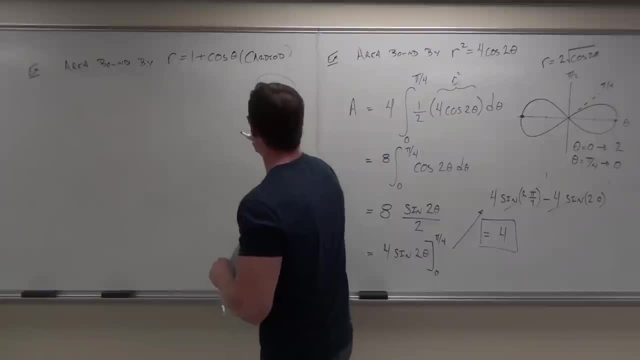 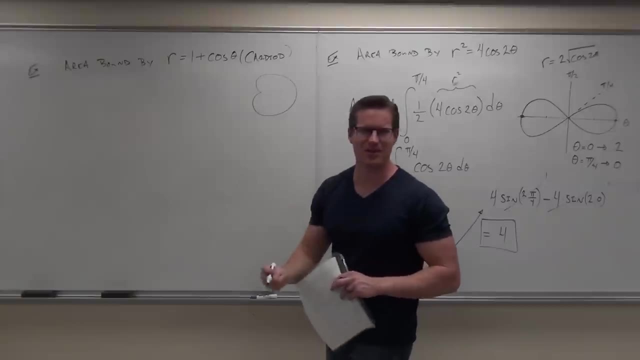 It was this one. Mine looks retarded, but it's okay That one. Okay, That's that one. I think I drew it backwards a little while ago. Oh yeah, I did draw it backwards. Oh, shame on me, darn it. 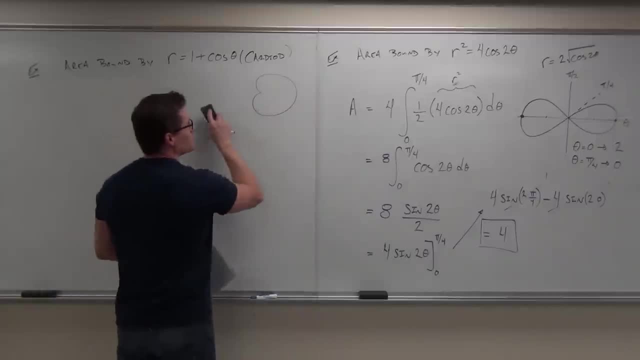 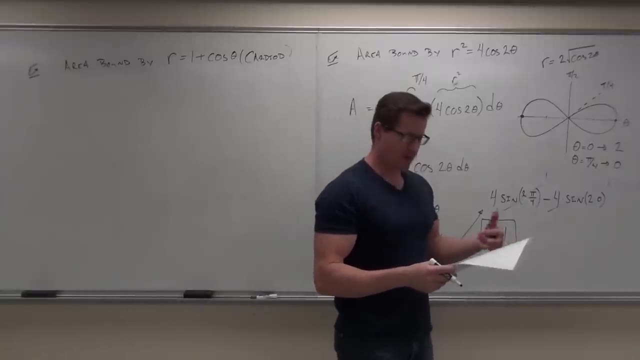 Oh well, it doesn't really matter. That should be me. So that's a cardioid, and that makes a lot more sense for a slope. anyway, Whatever, Let's find the area bound by this cardioid. Now there's two ways that you can do this. 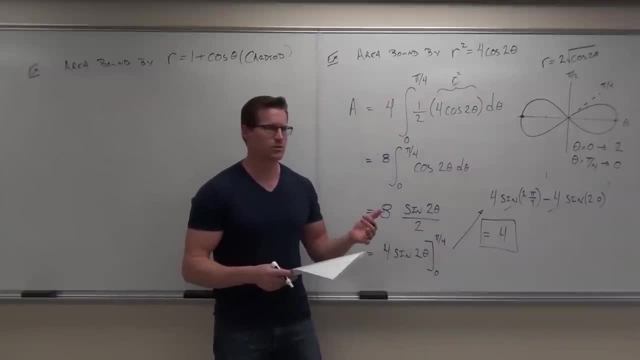 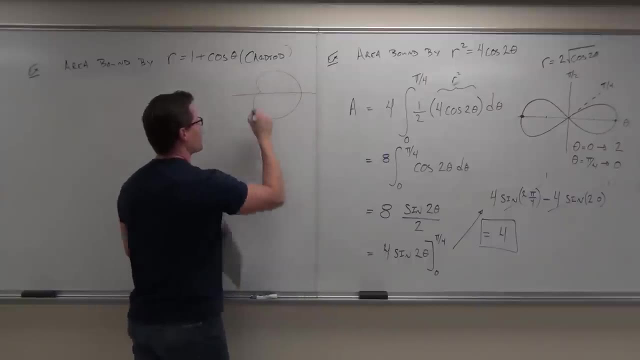 Firstly, do you understand that the cardioid is symmetrical? So, if I let me make sure I get it right, My dyslexia's kicking in. If I have that, If I have that, that point is at: theta equals zero. 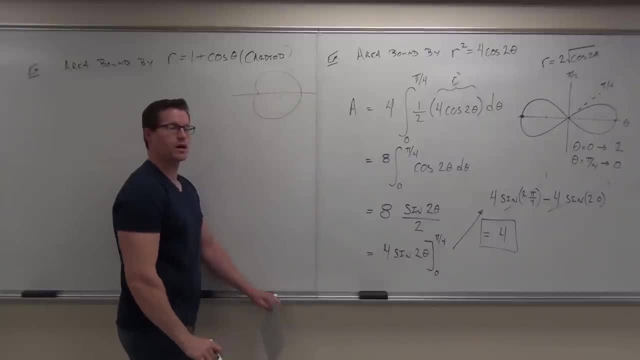 and this point is at theta- equals zero Pi Pi. that's right. So I can do this one of two ways. The first way I can set this up, we could set up the integral from. we could do it from zero to two pi. 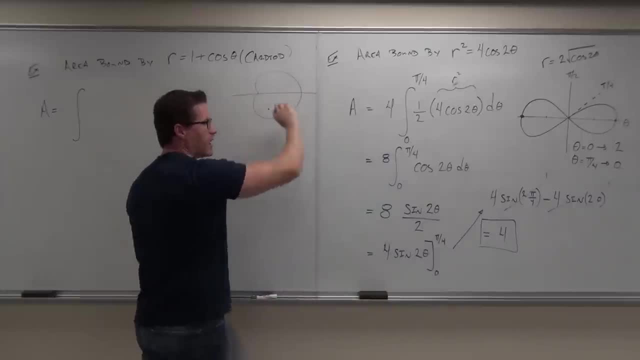 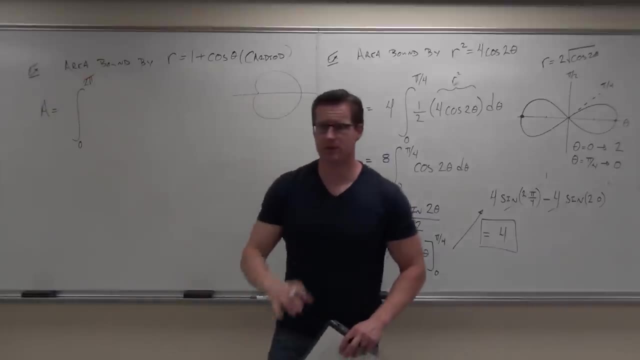 That would actually work. So if you want to go from zero to two pi, that's fine. Let's set it up that way first. So if I went from zero to two pi, that would be the entire region all at once. 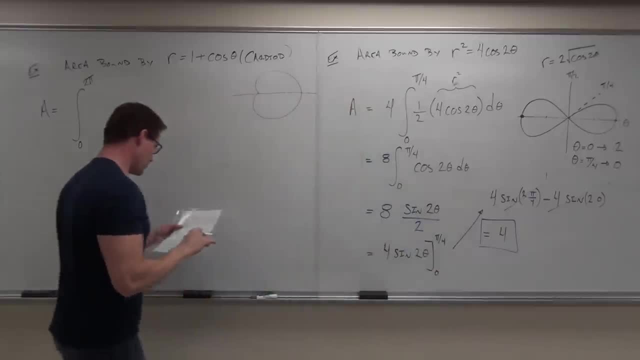 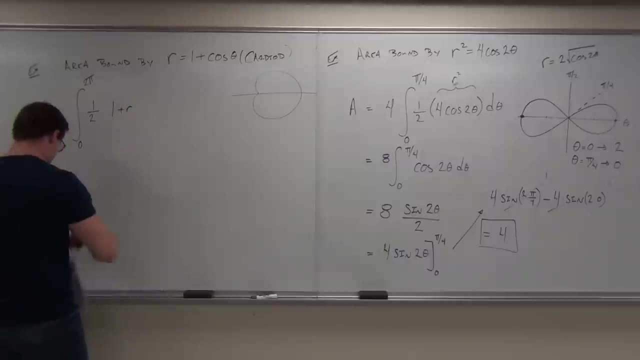 Are you listening? Mm-hmm, All at once, Let's do the formula. What would be inside of there? One half, Okay, the one half is there. very good. And then what? One plus cosine quantity squared? 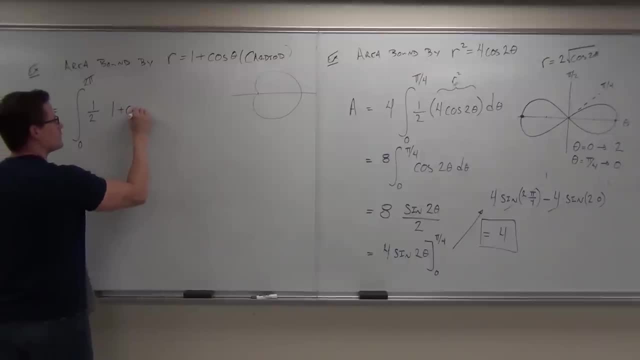 Where are we getting the one plus cosine theta from Rr? Uh-huh, square. Oh, why do we have to square it? Because r is not squared. Okay, very good. So this is one half r squared d theta. 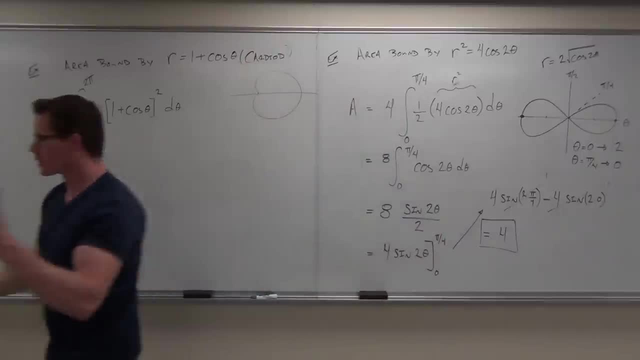 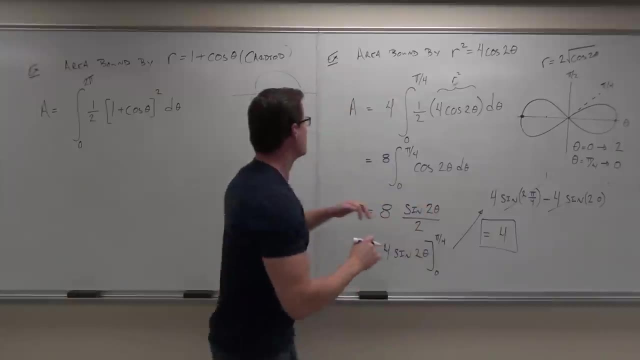 So can't you feel okay with that one? Now, if you work this out, you're gonna get exactly the same answer as if you were to do this one. So let's change our thought process a little bit. Let's say that I don't want to figure out. 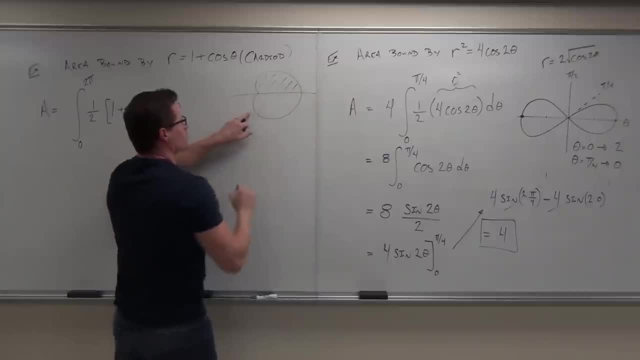 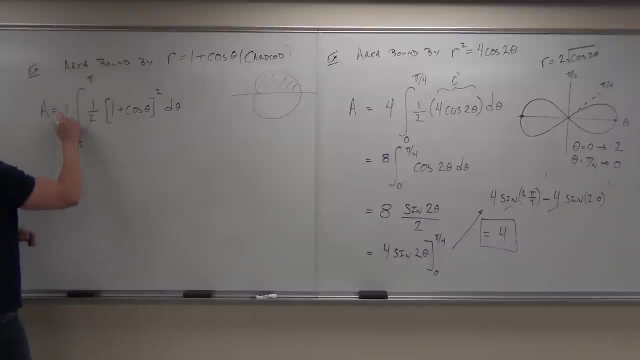 the whole thing at once. I just want to figure out this one. Do I still go from zero to pi? No, Where do I go from Zero to pi? And then what do I do? Multiply by two: Ah, so that is another option that you could do. 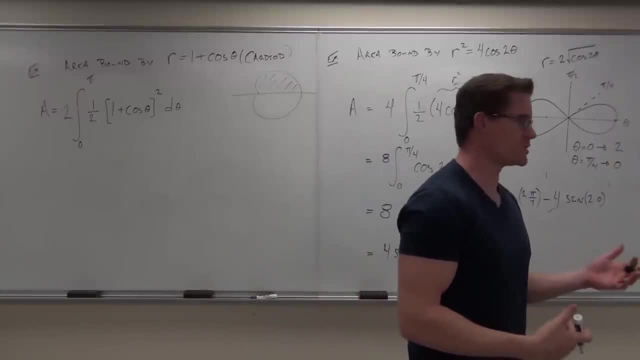 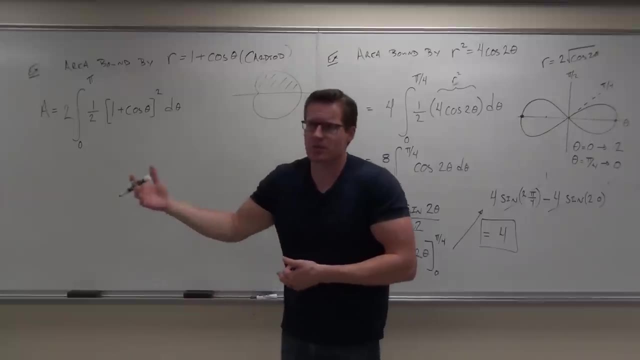 There's a couple ways to do this, because there's a lot of symmetry involved in these polar equations, So fancy, if you understand that idea. So, two different ways- does it matter? No, It does not matter. in this example, I would use a symmetry because I like smaller bounds. 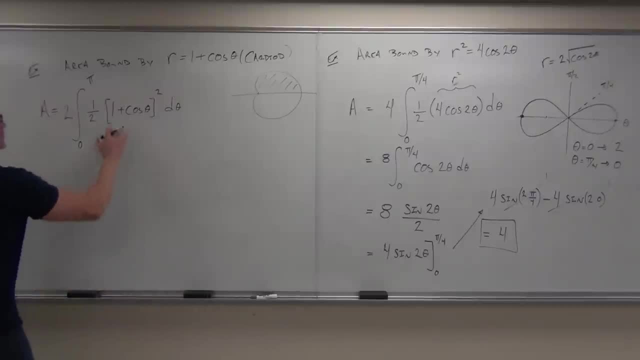 but it does not really matter. So let's go ahead and let's go through this. You want to do it this way, So maybe you don't have to deal with a fraction Two times one half, no problem. So our area is zero to pi. 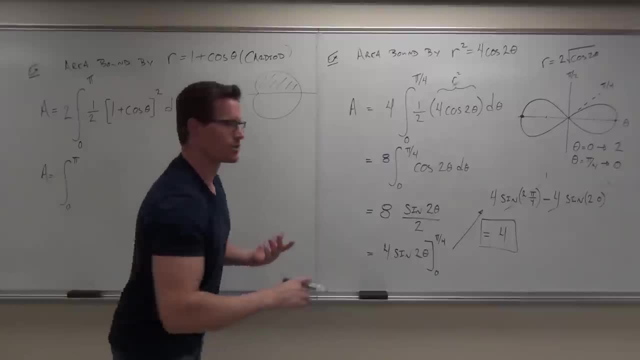 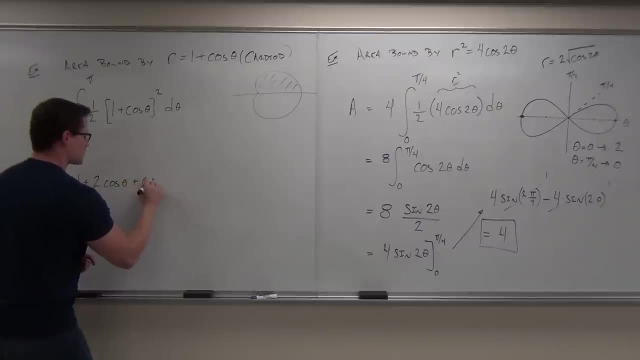 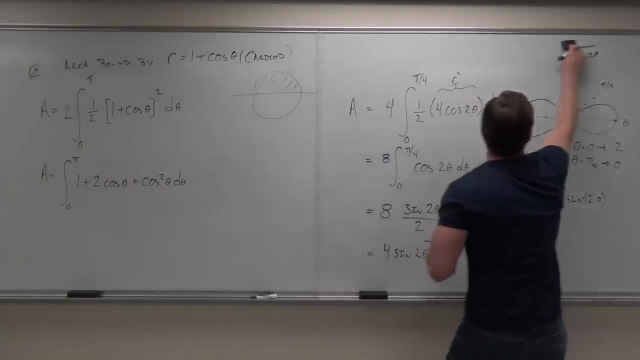 Two and one half are gone. You're going to have to distribute that. So we're going to have one plus two, cosine theta plus cosine squared theta d theta. Can you double check me on that? one, Mm-hmm. Yes. 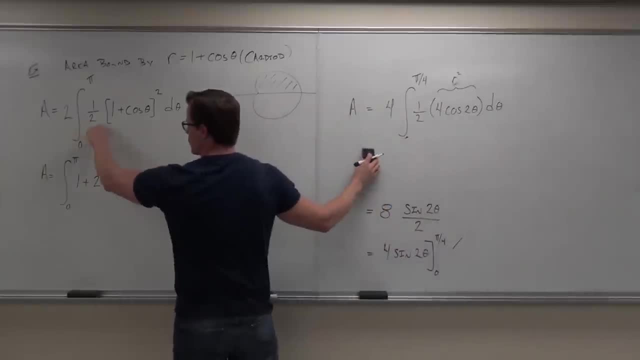 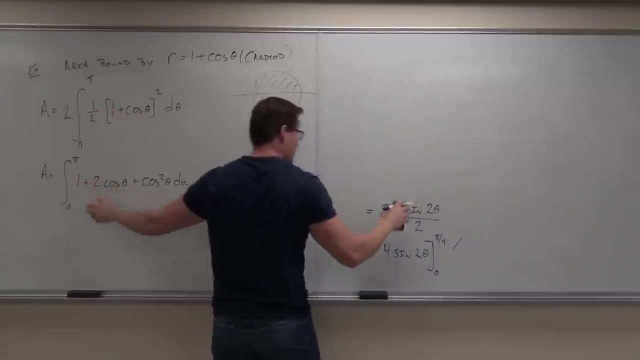 Hey, could you do the integral of and you understand why we don't have a two or one half anymore. right, We're just distributing this, Don't just square that and square that, Actually distribute it. Can you do this integral of one? 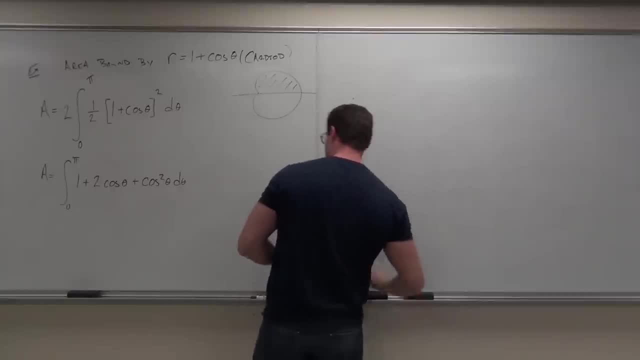 Can you do the integral of cosine a two cosine theta? That's pretty easy. Can you do the integral of cosine squared theta? Yes, Oh really, What is it? They were just on a roll with saying yup, Yup. 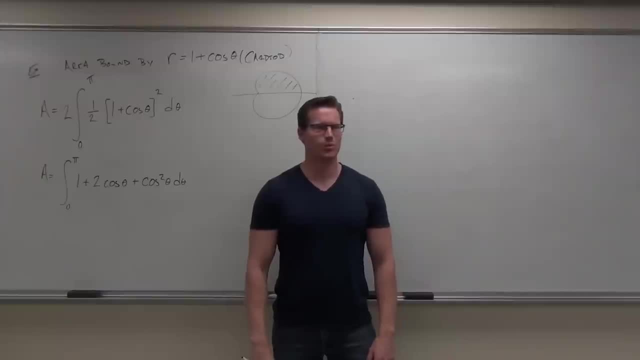 Yup, That's in the book. It's in the book, That's the book. I guess it's in the book. It's all in the book. Don't just say yup, Yup, Yup. I forgot Mr Leonard. Don't use the help. 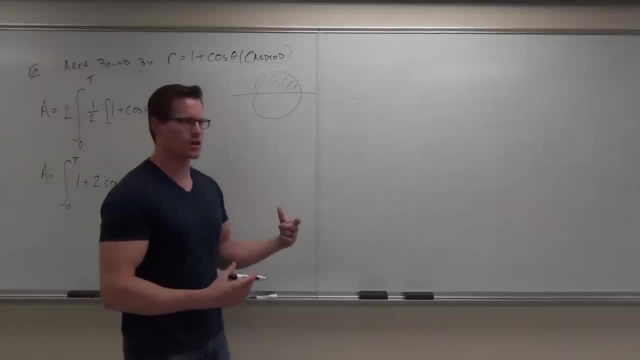 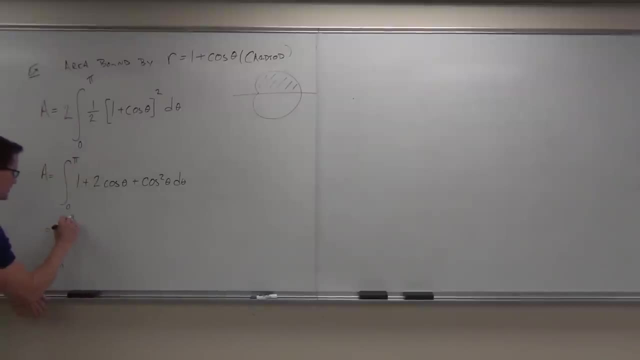 You forgot about your even functions when sine and cosine are both. even When sine and cosine are both, even You break it up. You do this. You don't just throw out random guesses, You use an identity to say: this is one half. 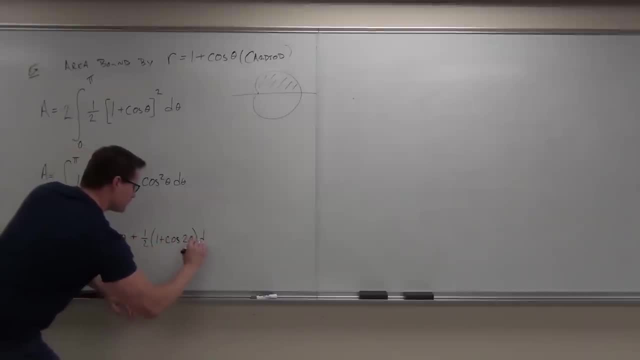 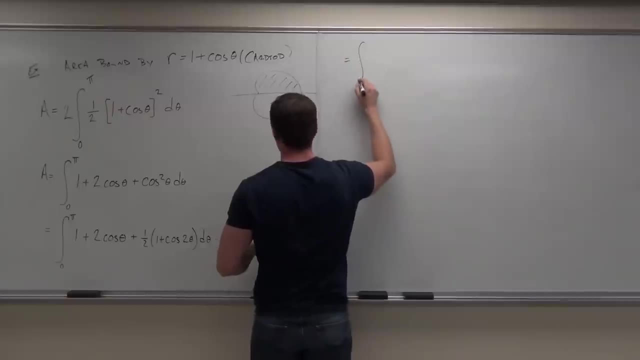 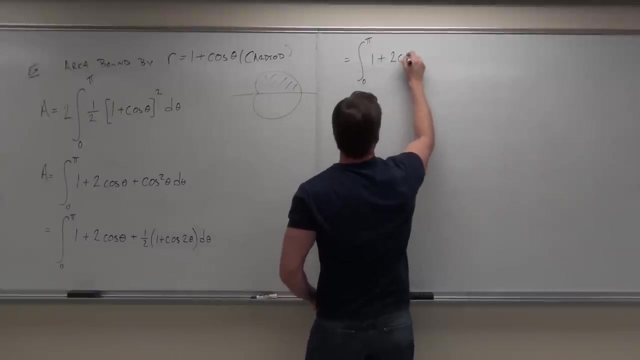 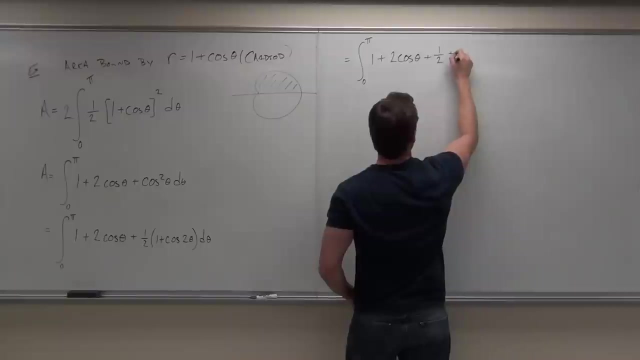 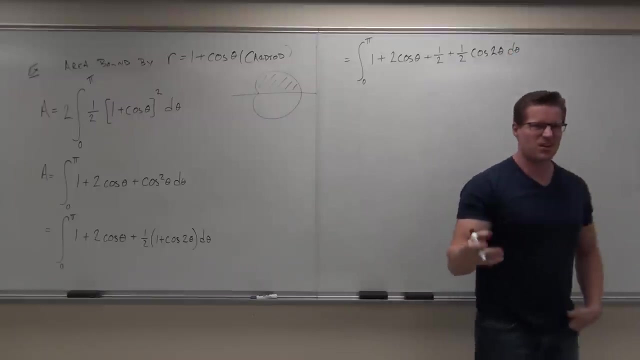 one plus cosine two, Cosine two. theta, That should ring a bell to you. Bells were a-ringing. Sad, sad news. Oh, what a Christmas Too loud to ring. Do you remember that at all? I hope that you do. 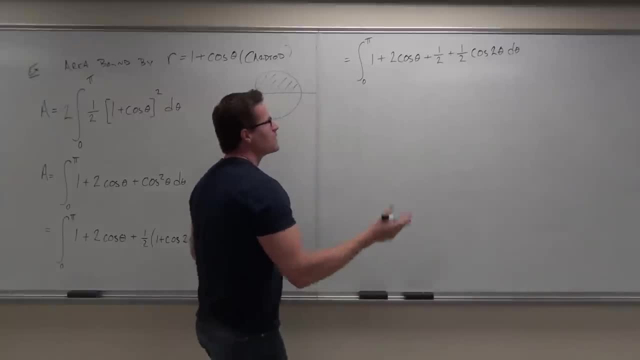 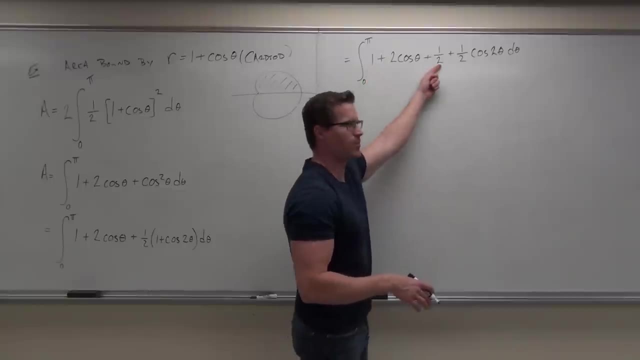 If you don't, you might want to refresh your memory on some of this stuff, because, hey, you're going to be using this. Before you start integrating, do yourself a favor and just combine some like terms, okay, So I want to integrate my one and my one half. 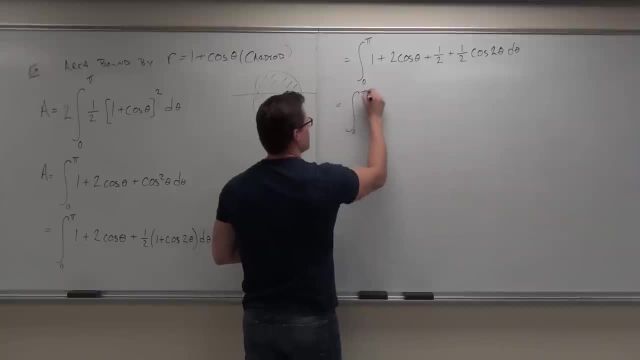 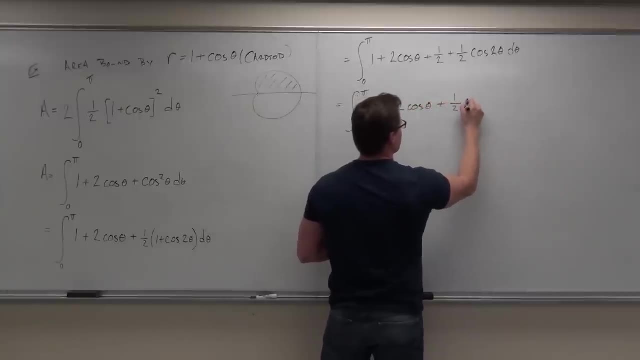 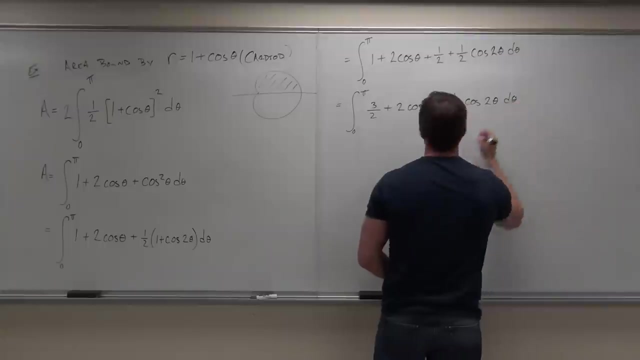 Just make that three halves and then integrate it, So we're going to go zero to pi. We're going to have three halves plus two cosine theta plus one half cosine two theta, Theta, d theta. Does that look better? Let's see if we can do all the integrals now, okay. 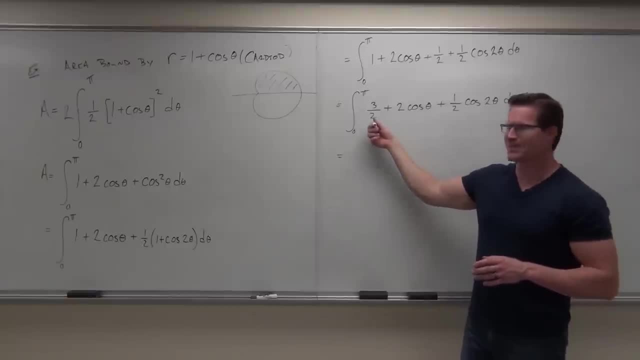 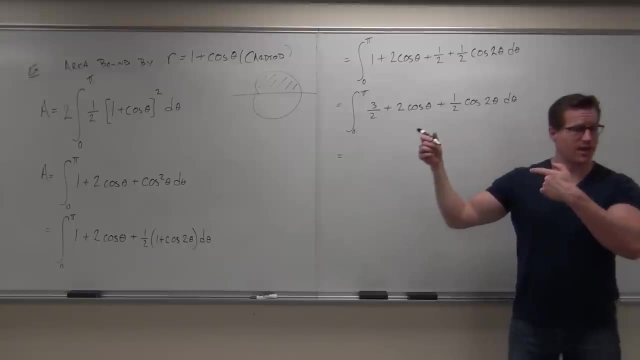 Don't just say, yup, Can you do the integral of three halves? Yup, How about the integral of two cosine theta, This one? Yeah, we actually just did that. It's a little substitution. We'll do it in our head. 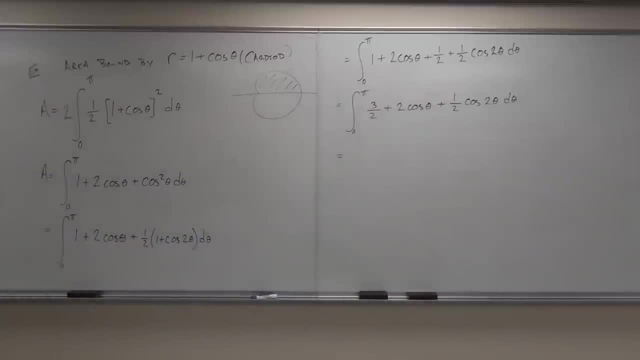 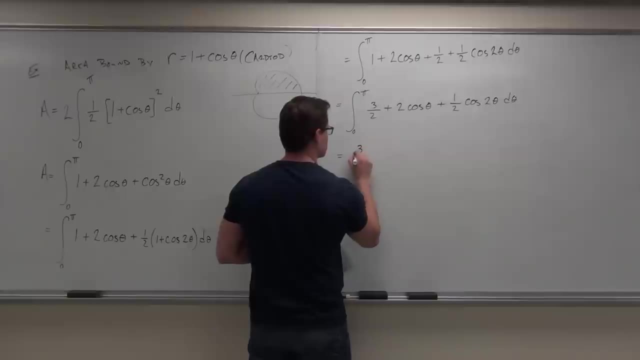 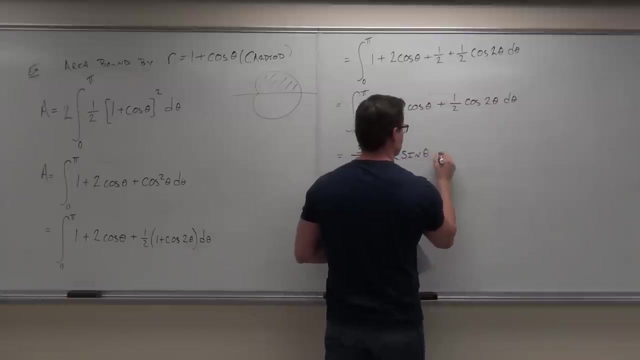 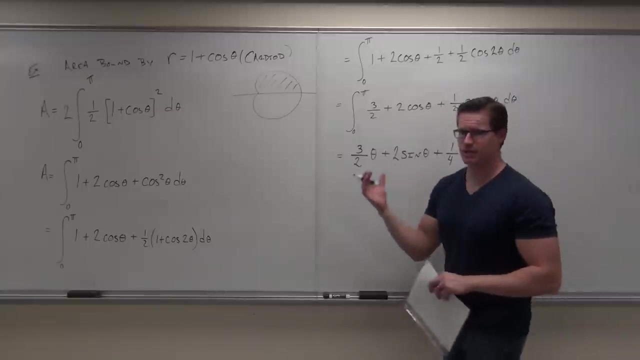 So go for it. Let's see if you guys can do it. Okay, I got a three halves theta. Did you get a three halves theta? Mm-hmm, Just go away. I got a two sine theta. Did you get a two sine theta? 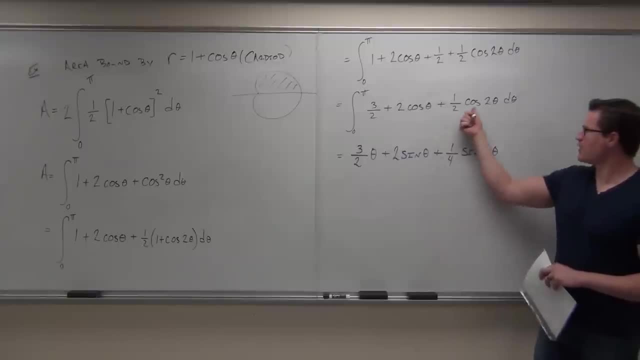 No negatives. I got a one half. Okay, I got a one half, but then this, right here, that's sine two theta over two because of our u substitution. We divide by the derivative of this little piece That's going to give me my one. fourth, 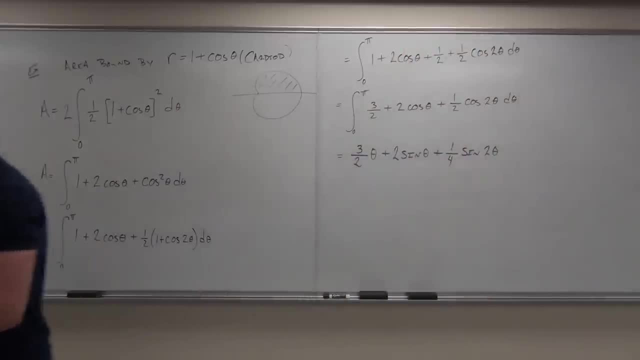 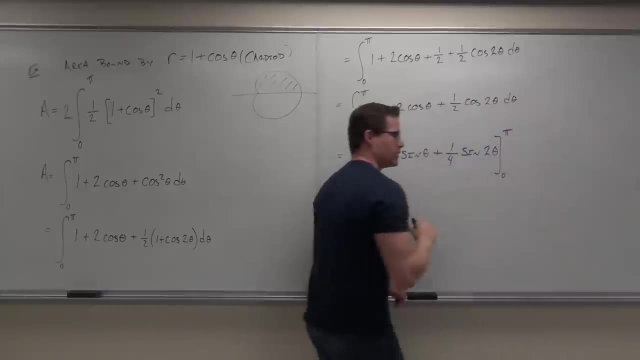 Show of hands. if you feel okay with that so far, Okay, We're good. What do we do now? Yeah, Let's evaluate Where are we going to go: from Zero to pi, Okay. So if we go from zero to pi, 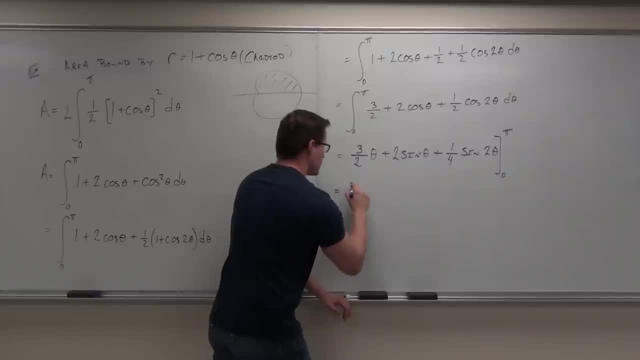 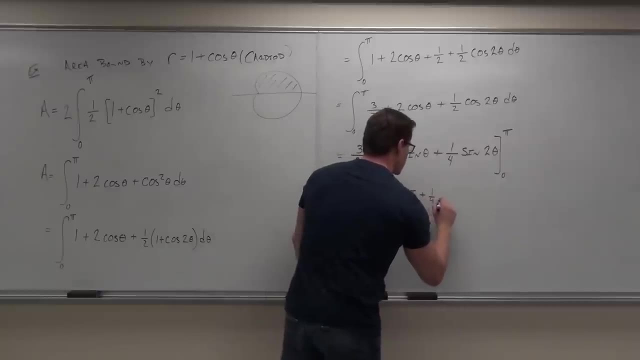 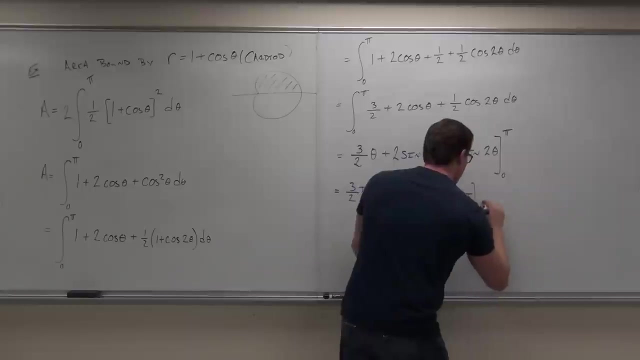 that says we're going to do which one do we do? first again Pi, So three halves pi plus two times sine of pi, plus one fourth times sine of two pi minus. well, you know what? I'm going to cheat a little bit. 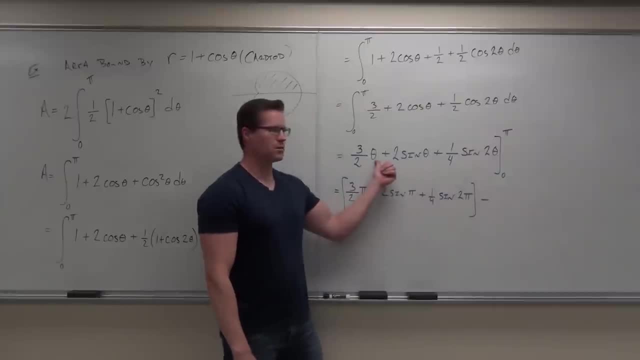 I'm not cheating, but let's look at it. If we plug in zero, that's going to be what Zero? That's going to be Zero. This whole thing is going to be Zero. This is all zero. Are you with me on that one? 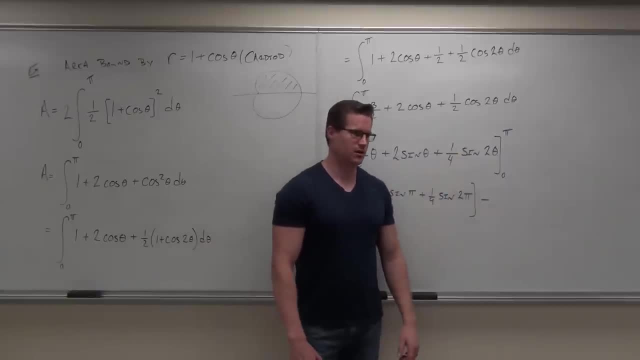 Yes. Now, if this was cosine, would I want to do that. No, No, because you're going to get ones out of those, okay, So this is a big old zero. Now let's do it. How much is sine of pi? 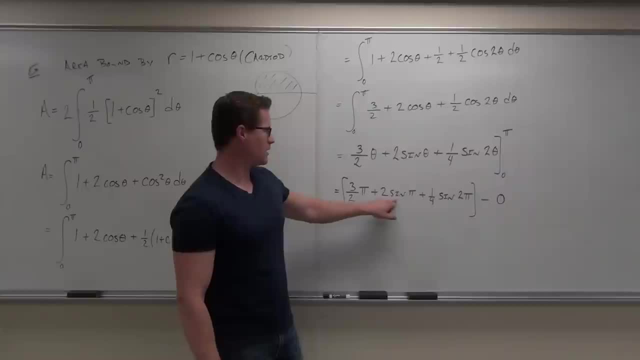 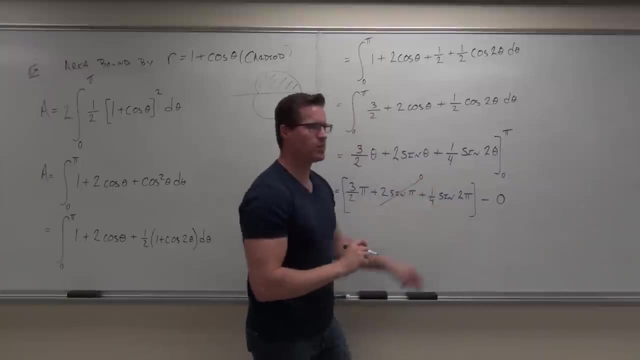 Come on quickly. Sine of pi Zero Zero. How about sine of two pi Zero Zero. Wow, That was a lot of zeros. What did we get? That's it, Our area. 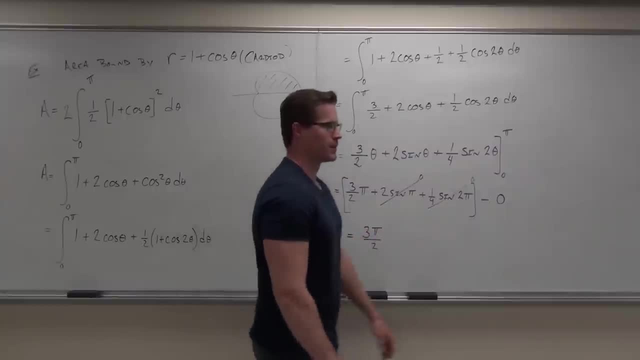 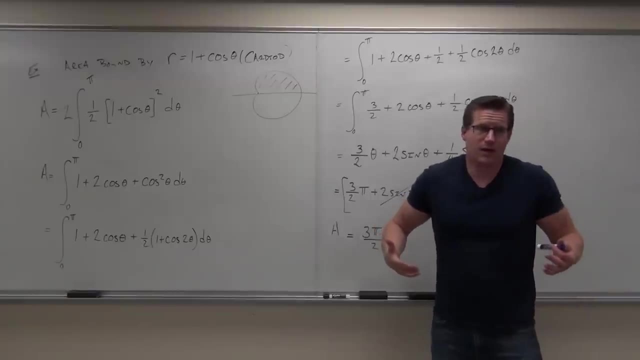 Our area is three pi over two. So when someone asks you, do you have a large heart, You say no, really, my heart is only an area of three pi over two. It's a finite number. 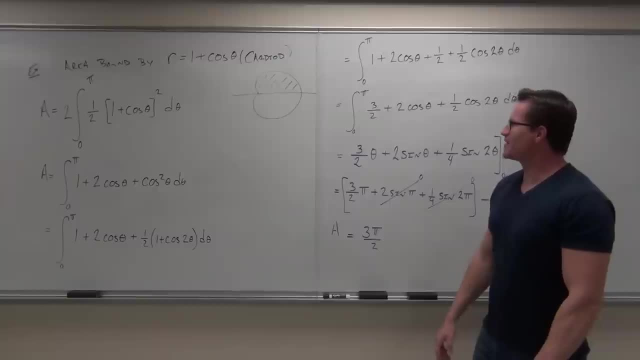 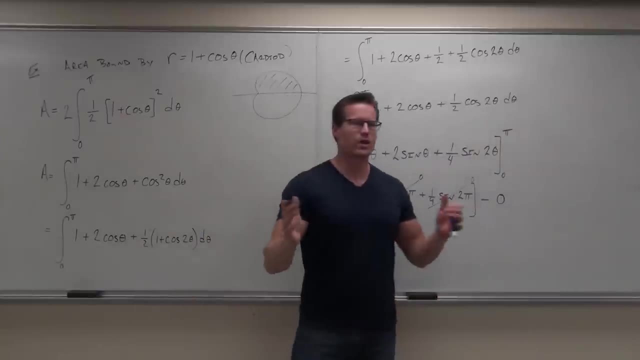 That was really dumb. Anyway, so the area of our car. by the way, do I have to multiply that by two, since I? No, Okay, we already did that, So we took care of it. Whatever way you work it. 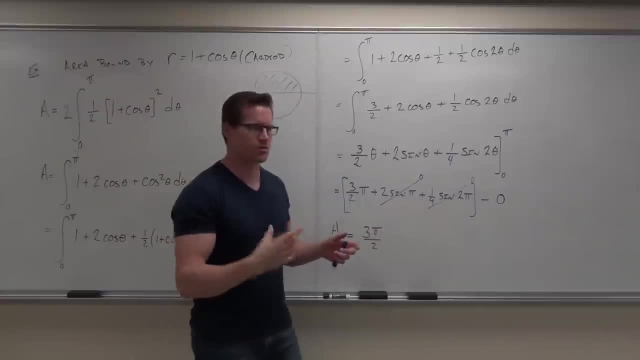 I did it another way too. Zero two pi works out the same. You're going to get three pi over two Show of hands if that one made sense to you. Cool, All right, we've got a couple more examples. We'll probably take care of them just next time. 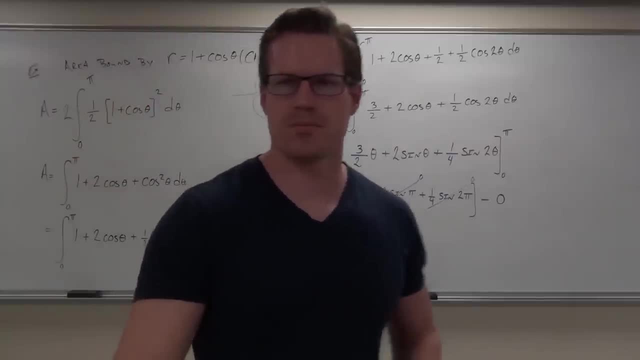 Okay, so the back end of our section here almost done. What we've done on last time was we found out how to find the area that's bound by a polar curve. Do you guys remember that from yesterday? Well, the way we did it was we said: all right, what we're going to do is we're going. 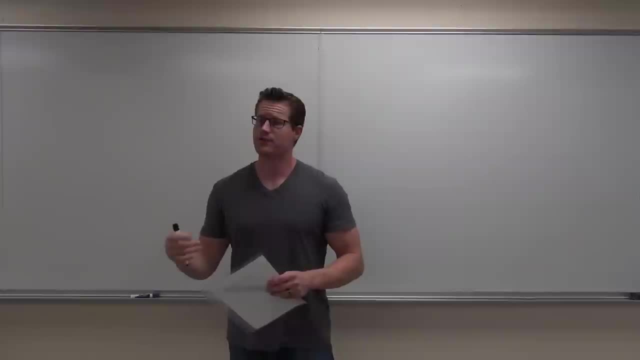 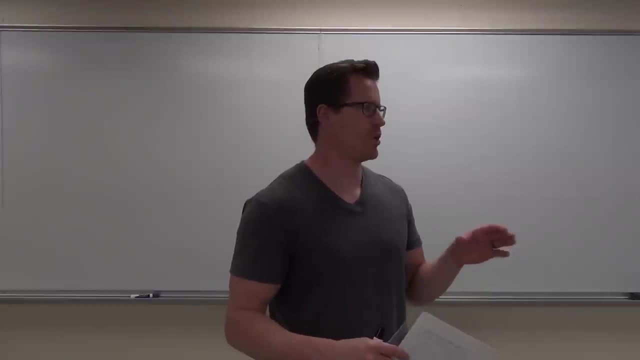 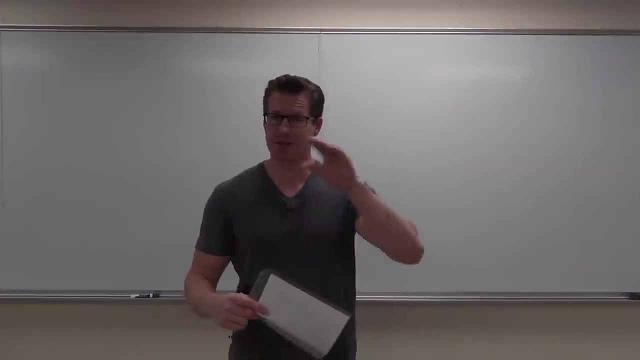 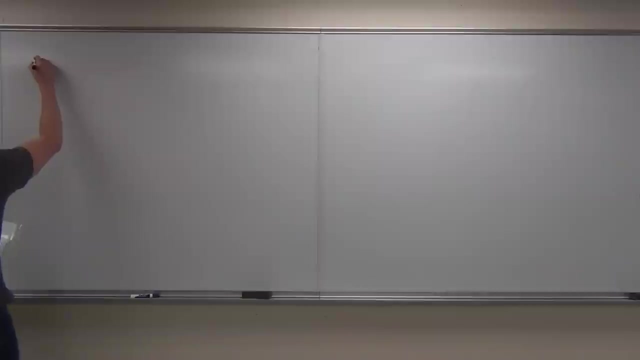 to take the area that's bound by a polar curve. 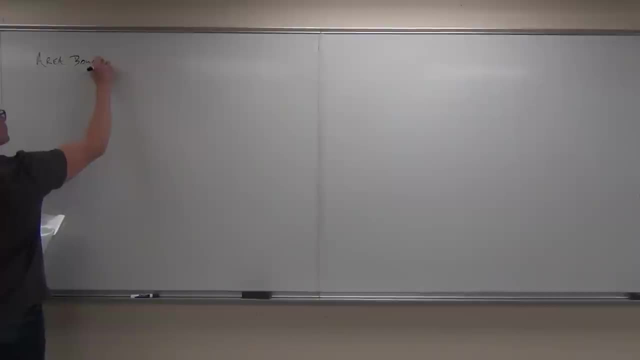 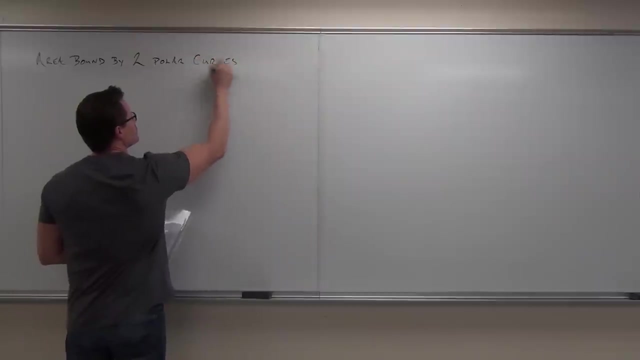 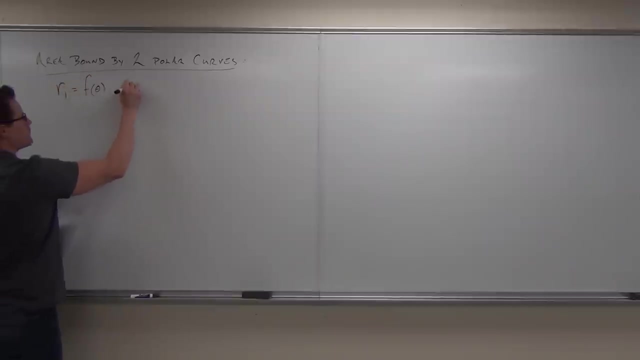 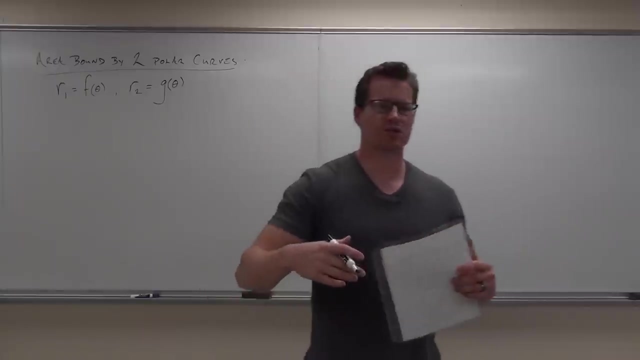 So let's suppose that we got two polar curves. We got r1 equals f of theta and we have r2 equals g of theta. So just two simple polar curves And we're going to integrate these on a certain interval. 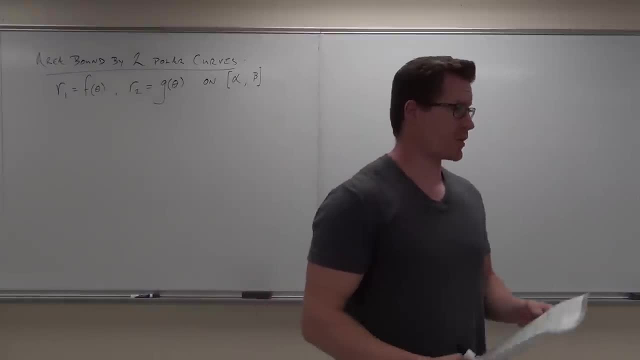 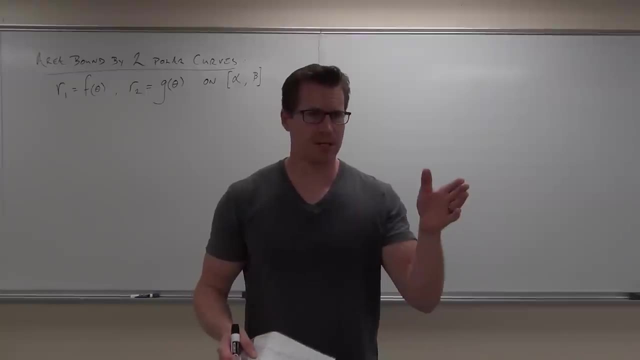 If you remember anything about calculus one, this is very similar to finding the area between two curves. You ever find the area between two curves, Do you at all? It was integral, right? It goes from a to b and it just said top curve minus bottom curve. 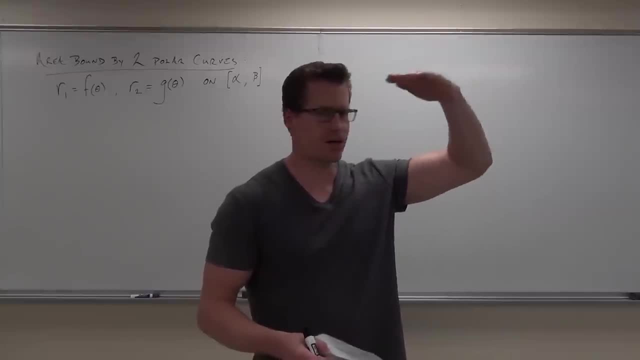 That's all it was. Area under the big curve minus area under the little curve. Well, that's what this is going to look like, except think about this for a second: The area bound by a polar curve looks a whole lot like the area of a sector. 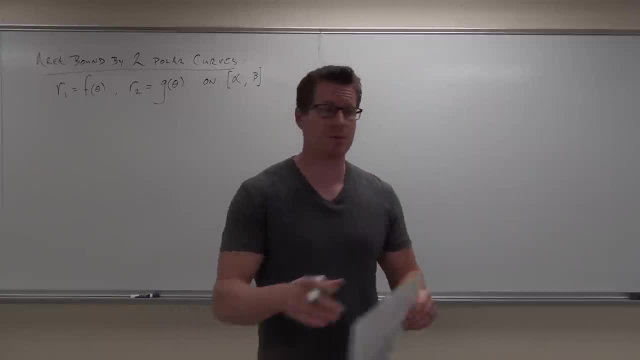 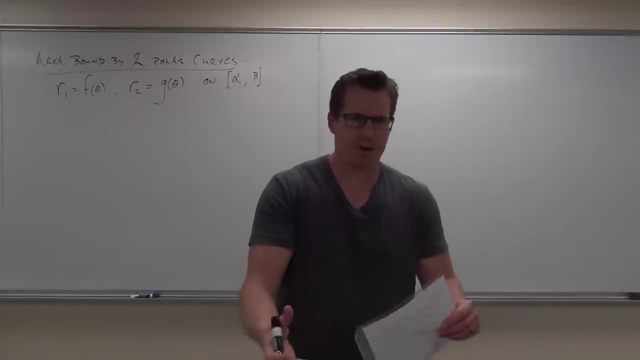 because the area of a sector is what we're integrating, And so this is going to be big, curve, curve minus little curve, but it's also going to fit our idea of area of a bound by a polar curve like a sector. So let me show you what this is. 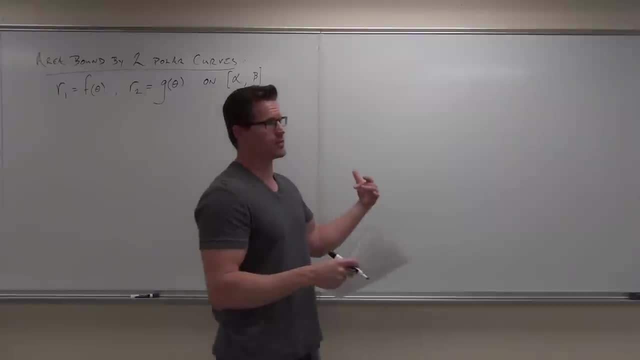 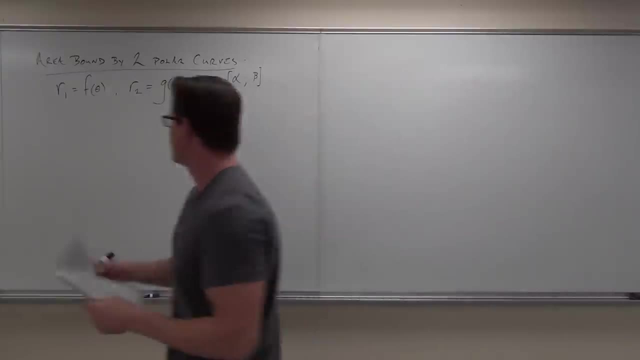 So suppose we have two curves- f of theta and g of theta- Those are our two polar curves- And suppose that we know the intersection of them or we're just going from two angles- alpha to beta- Then the area between these two curves is going to look like this: 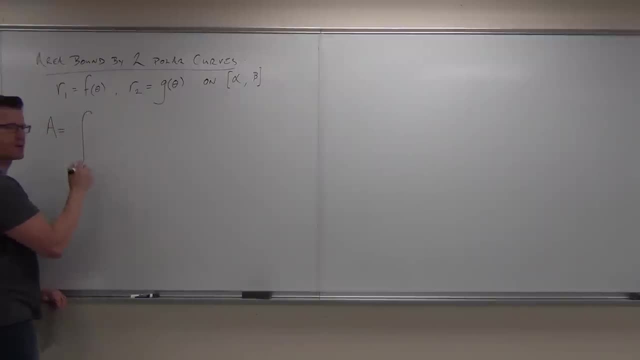 Let me refresh your memory here real quick. Area under or area bound by one curve would do this. It would do alpha to beta, It would have one, It would have r squared and then it would have d theta. Does that look familiar? 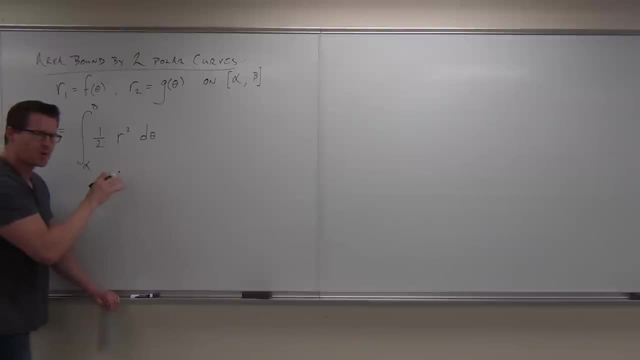 Don't write that down, You already have it. okay? Does that look familiar to you? Do you remember this? This was look at this. This is area of a sector as we're letting the angle change. We're adding up all little sectors. so adding up all the sectors as our angles change. 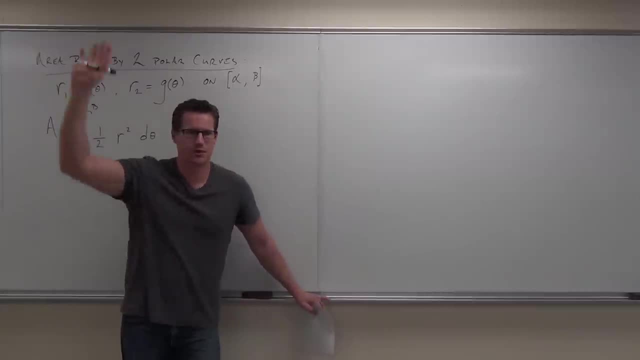 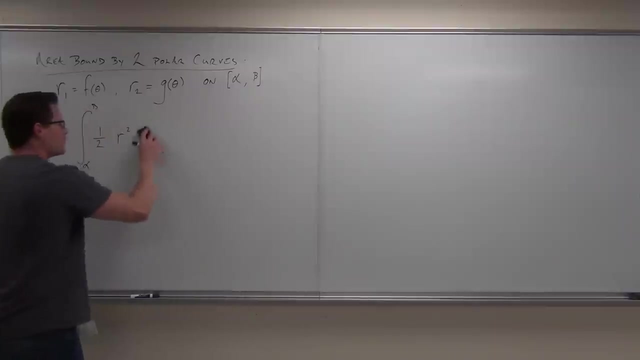 or with little teeny, teeny angles. Show of hands, if you feel okay with that one. Now, if we have two of these, then here's what we're going to do. Basically, we would say, all right, well, you know what we'd do. 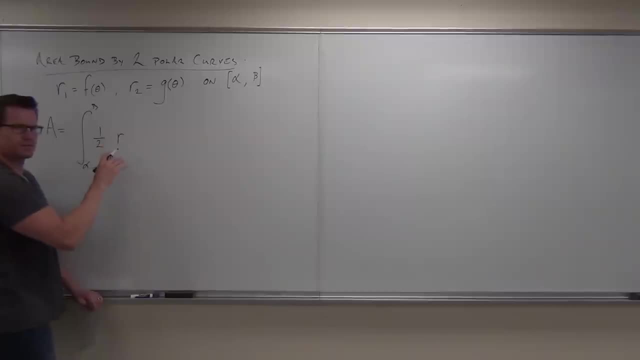 We'd have, don't? I'm going to kind of work with this for a little. I'll kind of semi-prove this, all right. What we would do is we'd say, hey, here's, here would be the big area. 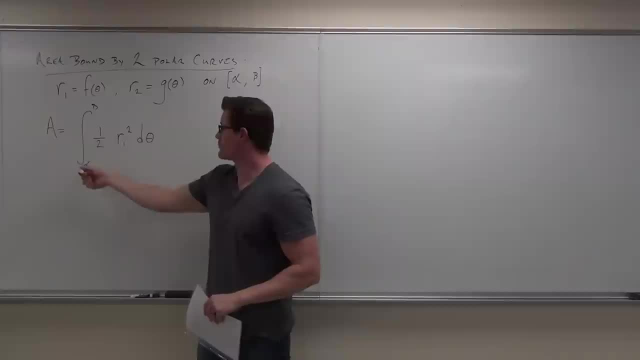 So if we want to find the area of this, just the area bound by this one, we'd go from alpha to beta. one half of r1 squared d theta, We'd find that integral. Does that make sense? If we want to find it between a big, 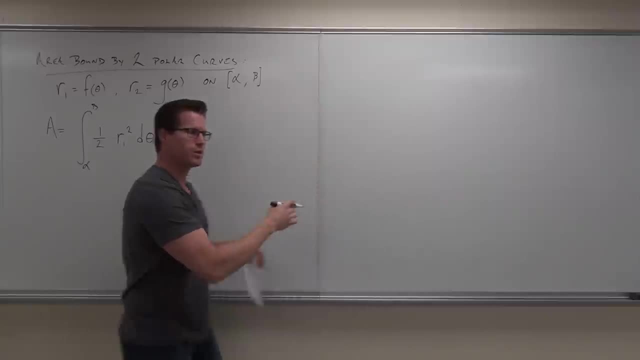 polar equation and a small polar curve, then we would do what? Remember this: Find the area between these two curves. What do you do? So, if that's x-axis, find the area between those two curves. What do you do? 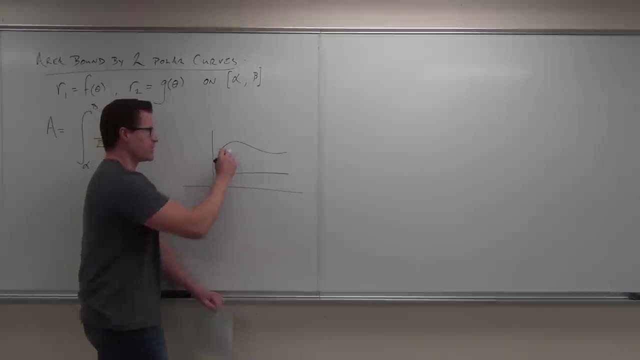 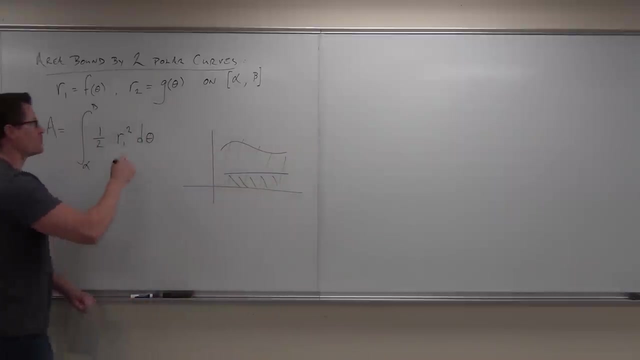 Subtract the little one from the big one, Little one from subtract the little from the big one. So we'd find all of this and we'd subtract that. Remember that. Well, we're going to do the same thing here. We'll find all the area of the big one. 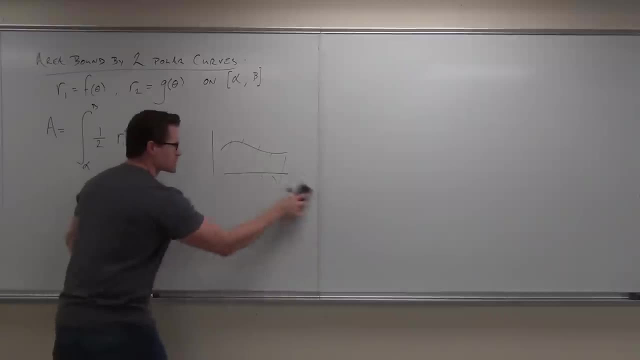 and we would subtract that Subtract the area of the small one. I'm going to work with this for just a little bit, so you can see where this is coming from. We'd subtract, on the same bounds of integration, the area of the small one. 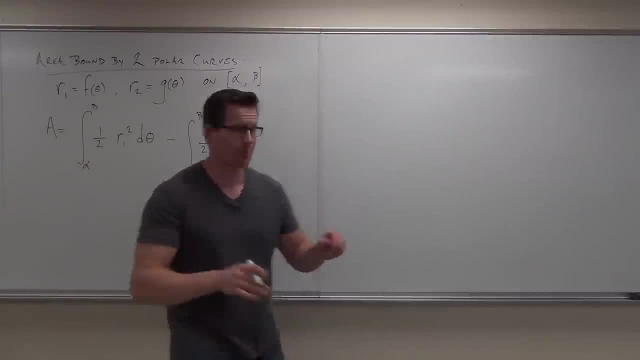 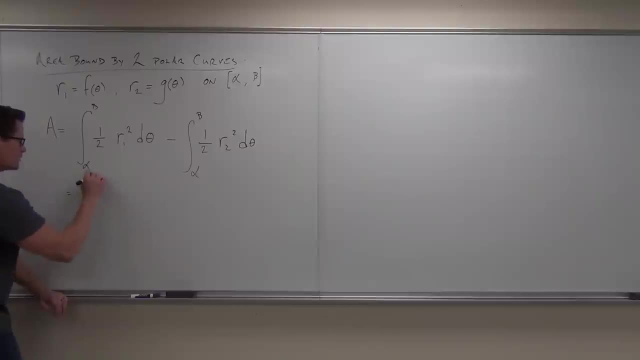 Does that make sense? Hello, yes, no, Okay. so if we put them together because they have the same bounds, we end up getting alpha to beta one half. I can even factor the one half R1 squared minus 1.. 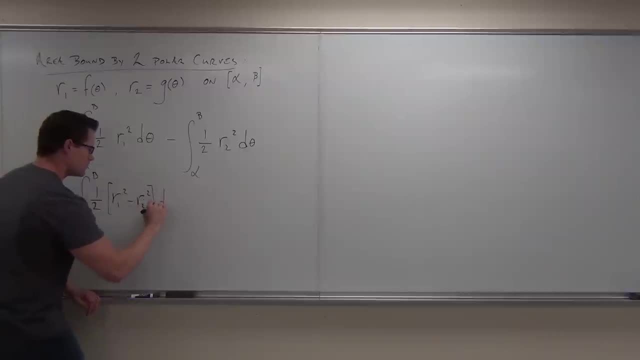 That's R2 squared d theta. Can you make it there algebraically? Just factor the one half. We're grouping these two things together. Well, let's go one step further. The one step further says that R1 is actually equal. 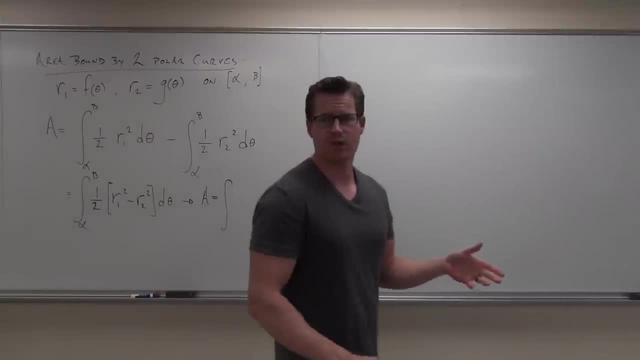 to some function in terms of theta. So instead of R1, we could write: okay, let's try this again. That was weird. Let's try this again Instead of R1,. R1 is actually equal to the function of theta. 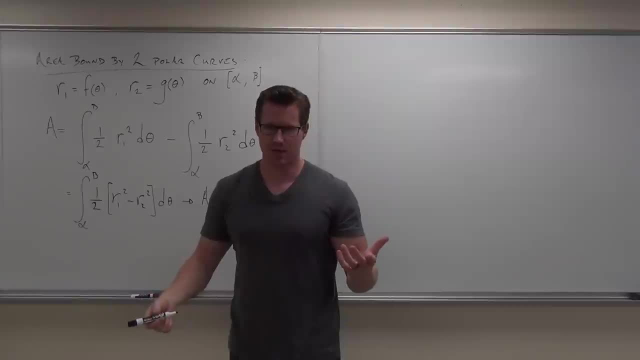 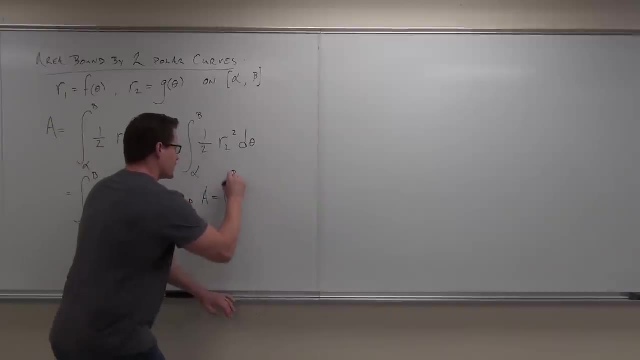 So instead of writing R1, we could write that's right. Instead of writing R2, we could write: that's exactly what we're going to do. This is the formula that you guys are going to find. So we'd say alpha to beta. we'd have the one half. 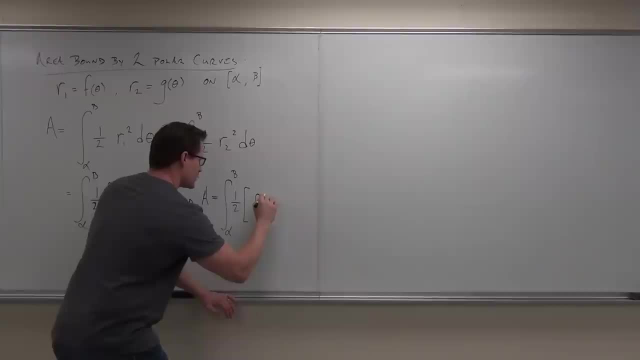 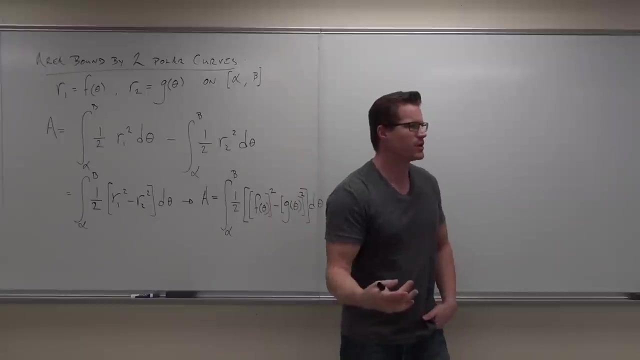 We would just have f of theta squared minus d of theta squared d theta. That's the whole idea. This is what we're working with right now. Chopin should be okay with that so far. Do you guys see what it's doing? 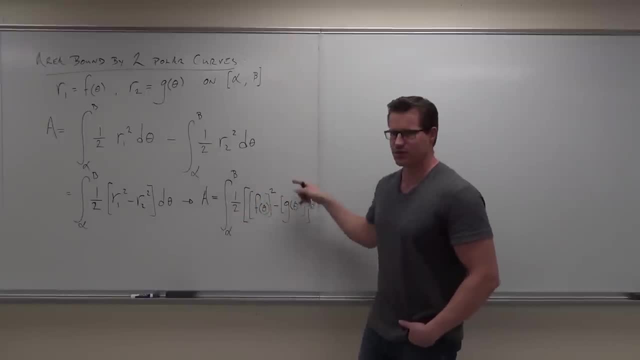 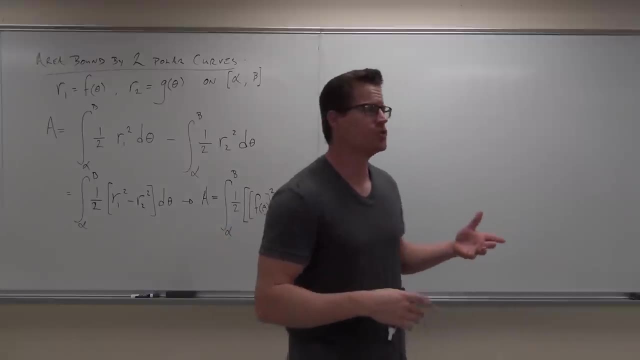 Do you see how it's taking the area of the big sector minus the area of the little sector? Do you see what it's doing? Just saying, hey, big one minus little one, That's it. That's going to give us the area between these two polar curves. 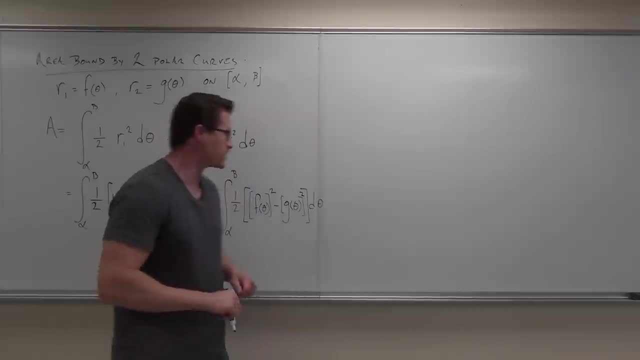 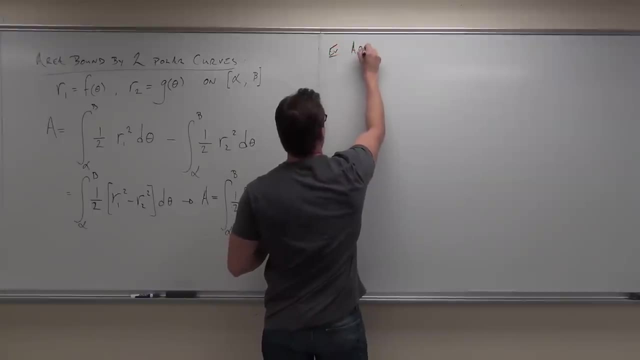 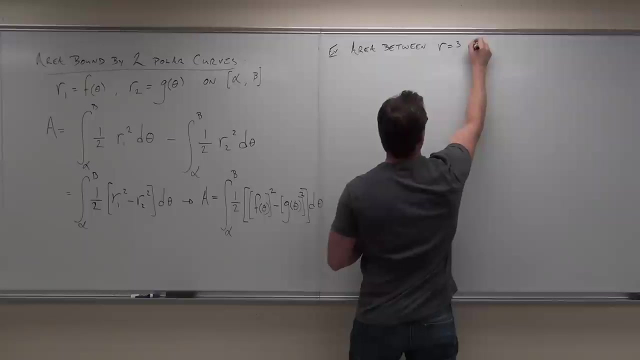 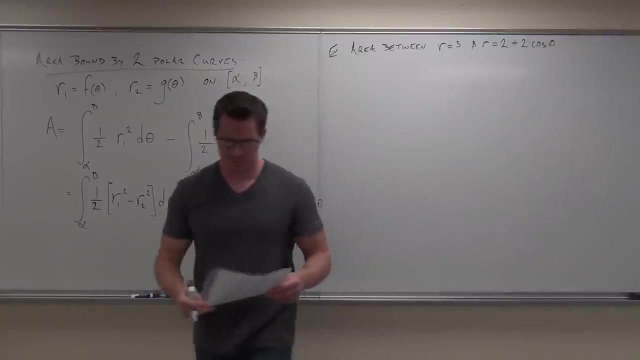 Do you guys want to try an example real quick to see what this is all about? Yeah, Okay, So let's do that. So I want the area Between R equals 3 and R equals 2 plus 2 cosine theta. Find the area between R equals 3 and R equals 2 plus 2 cosine theta. 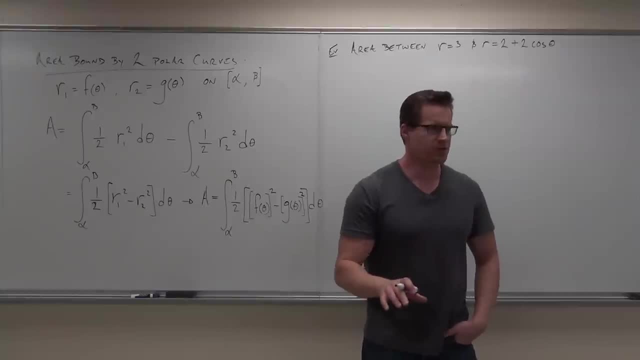 You know what? I'll show you how to do every bit of this, but we might want to think about what this even looks like before we get started on this. So So, firstly, do I have two polar curves? What do you think? 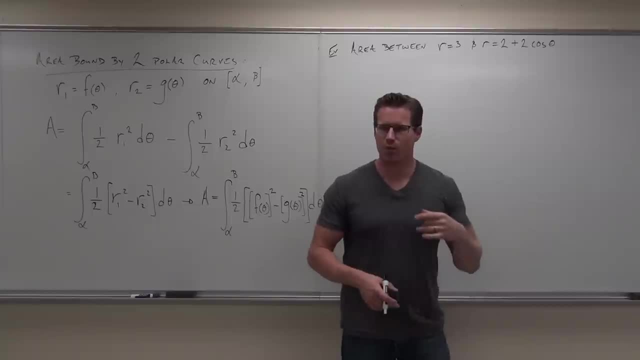 Yeah, Is that a polar curve? For sure. Can you think about what that looks like, If you can't do a little manipulation with this? So you might want to think of this as R equals 2 times 1 plus cosine theta. 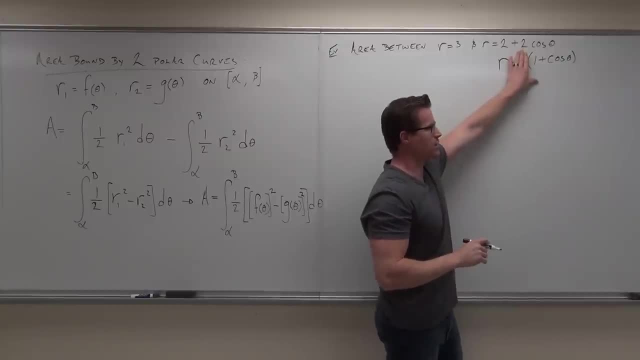 Hey, look at that. What's R equals? You all should know what's R equals: 1 plus cosine theta: R equals The cardioid. What's 2 times that? Just a bigger cardioid, A bigger, a larger heart. 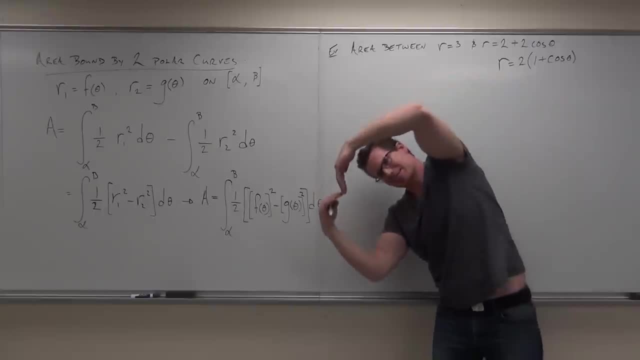 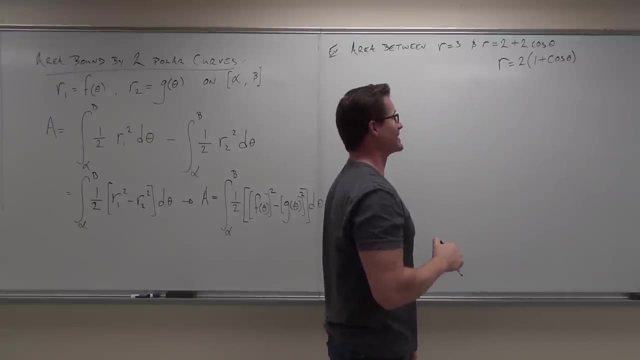 Now, is this the one that's like this Or the one that's like this On its side? Yeah, That's on its side, That's right. That's the spooning. cardioid is what we like to say. Well, what I like to say, 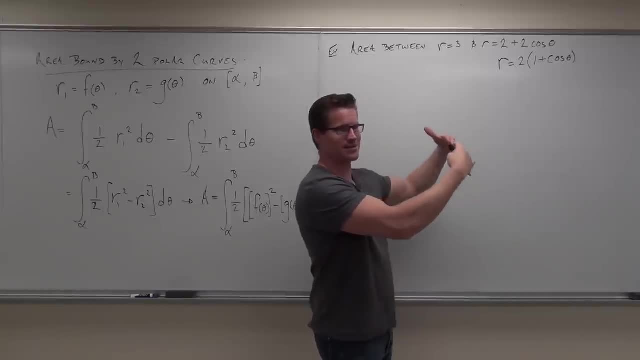 It's just funny Anyway. so this is a bigger butt, This We like big butts and I've been working on that one for a while. The bigger butt, These little brothers. they can't deny. When a cardioid walks in with a hood, look, it doesn't matter. 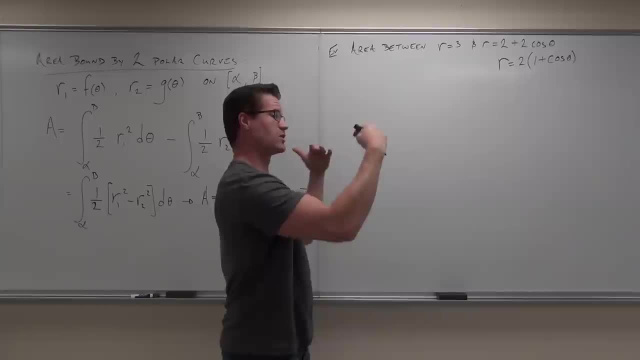 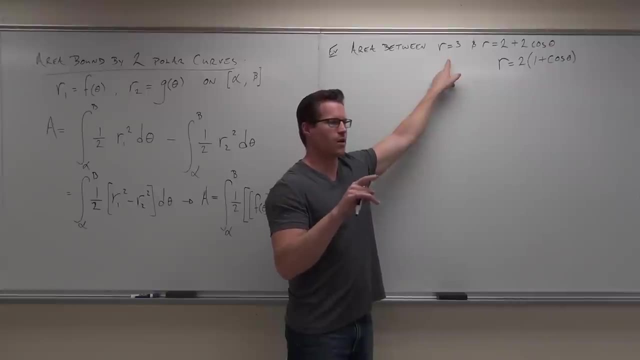 Okay, so that's a cardioid. It's on its side, just a little bigger. Now, what's R equals 3? Is there a theta there? No, No, Now think about this. This says R equals 3, no matter what the theta is. 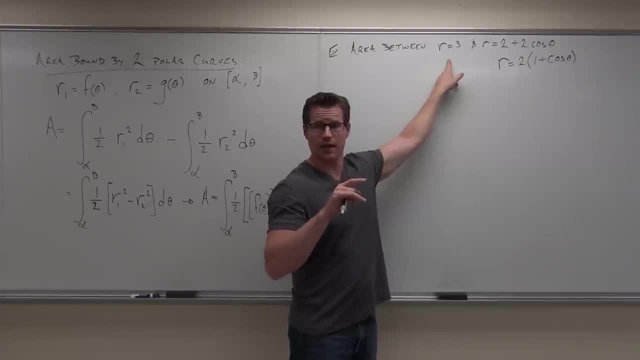 R is a constant. R does not change. What does a curve look like when it has an R that doesn't change, no matter what? the theta is A circle, Not a line. A circle, It's a circle. Can you imagine something that just has a line? 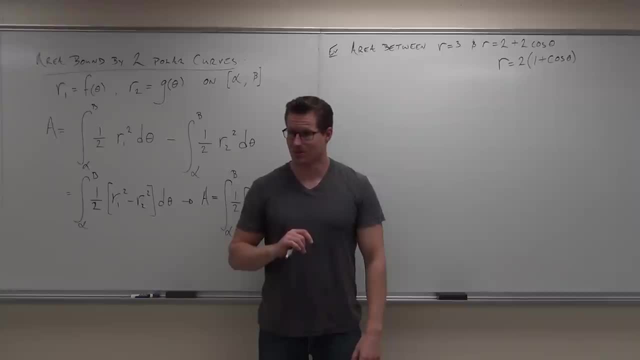 A circle, A radius of 3.. What is it? It's a circle. So what this says is that our curve looks something like this: We have 1,, 2,, 3, and 4.. Our circle would have a radius of 3.. 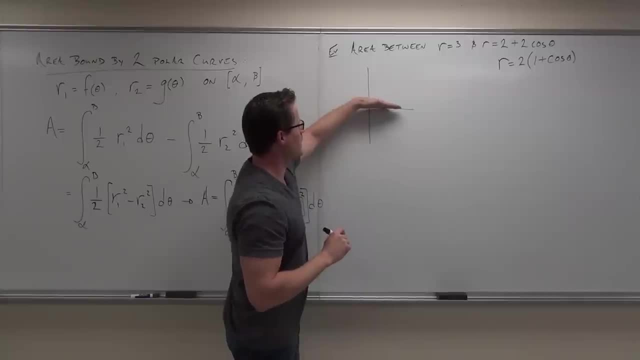 So notice this. This is what it's saying. It says that if you allow the angle to change and the R doesn't change, it says, hey, R is always 3,, R is always 3, R, R is always. it's going to be a circle. 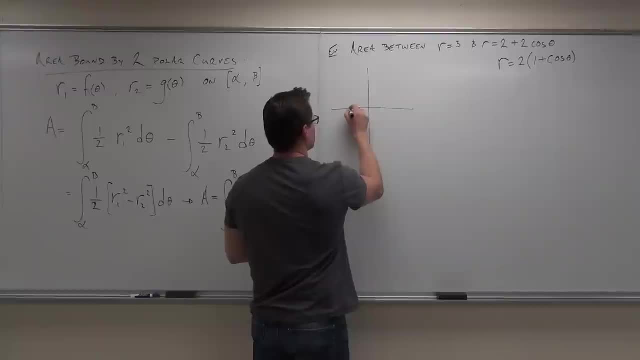 1, 2, 3, 1, 2, 3, 1, 2, 3,. so our circle would look like: oh man, I don't know if I get this right. Oh, it's okay like that. 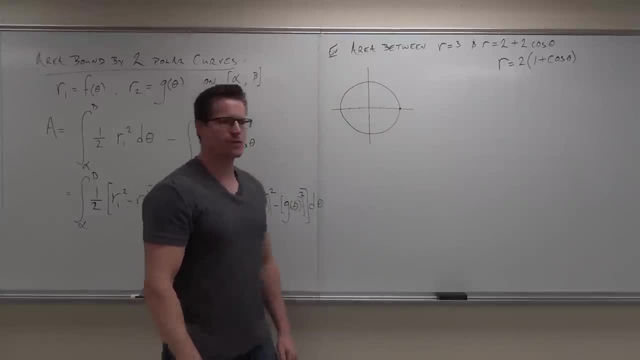 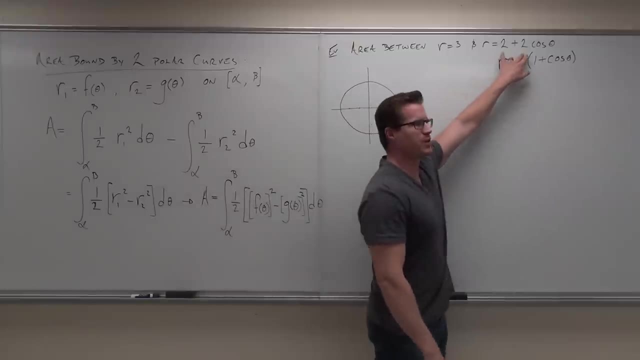 Should fans feel. okay, that R equals 3 equals that circle. Now how about the next one? Check this out: R equals this cardioid, this bigger cardioid. Now, here's what cardioids normally do. Look up here at the board, please. 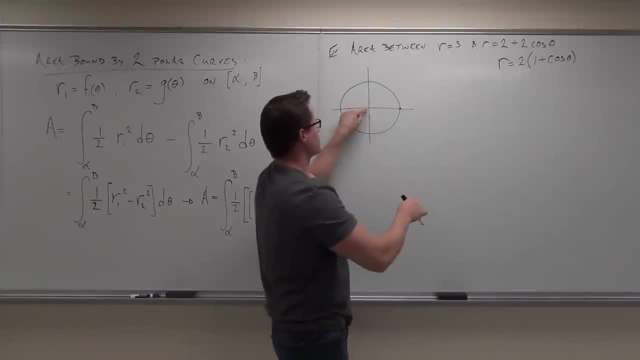 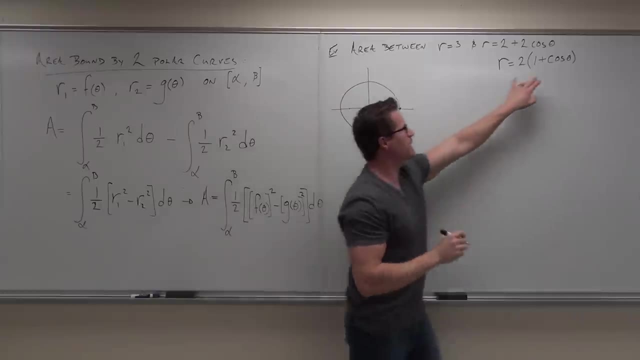 Typically, this is what cardioids normally do. This cardioid would have a point at 0 and would have a point at 2.. Do you remember that? It would look like this? Well, if you take all those values, those R values, and you multiply them by 2,. 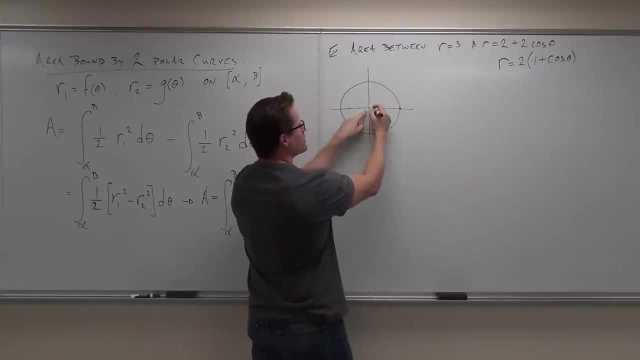 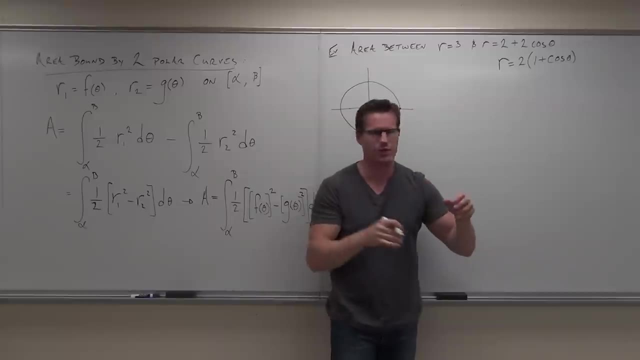 it just doubles that. so instead of having oh well, we still have 0,, don't we? Because 0 times 2 is still 0. So we're going to be crossing at the pole, at the origin, But if we normally went to 2, now we're going to be going to 4.. 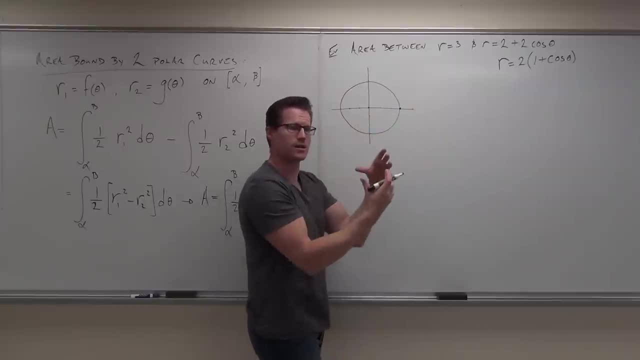 Very good. So our cardioid's going to be outside and inside of our circle, So here's how it's going to look. Cardioid looks something I'm going to draw in purple so you can see the difference. Looks something like this: 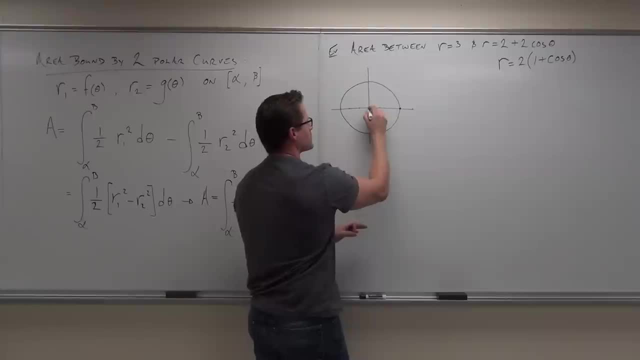 It says normal cardioid. hey, goes like this: Wow, that was awful. So bad at this Normal cardioid that An enlarged heart would do this, This, This, This would say: now we're taking all those Rs and we're multiplying it by 2.. 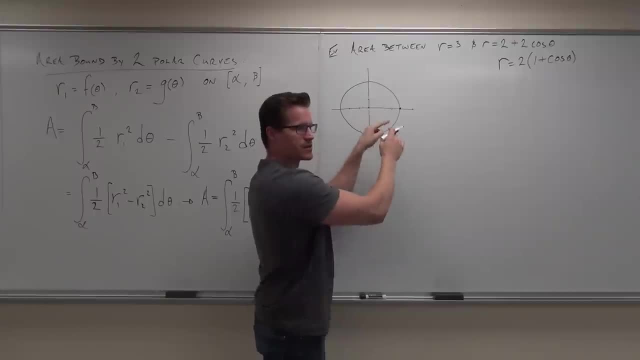 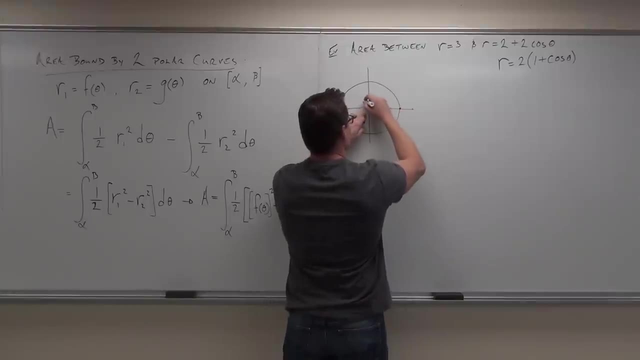 So every distance is going to get a little bit further from the radius It's going to. all those Rs are going to double. Does that make sense to you? All the Rs double looks something like this: Okay, I'm you know what. I'm a little off. 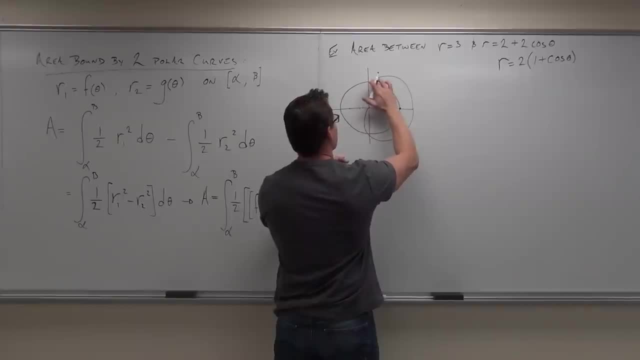 My heart's got a bad heart. It's too emotional. Felt like that. This one's way off. Okay, let's kind of just assume. all right, I wish I wasn't a perfectionist. It's called OCD. Okay, obviously I'm not a good artist, okay. 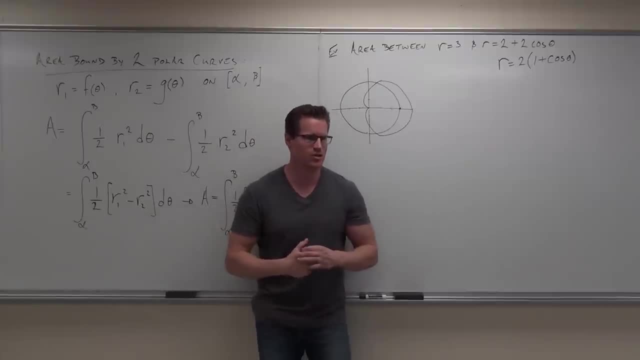 My bad, My bad. Do you get the picture? No pun intended, but do you get the picture, the idea here? So R equals 3, circle radius of 3.. R equals 2 plus 2. cosine theta is a cardioid. 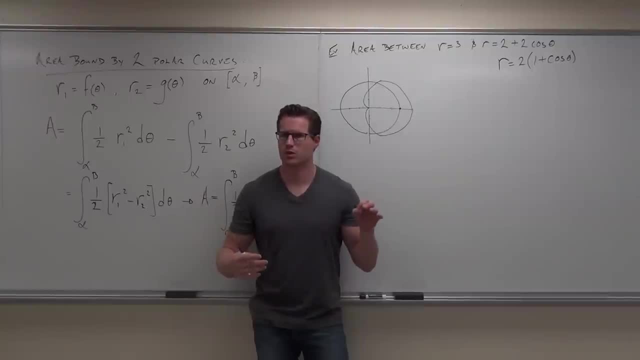 It's just a bigger cardioid. Do you see that these curves are going to intersect? So what we're looking for is the area bound by these curves. The area bound by these curves in this instance that I want to look for is this: 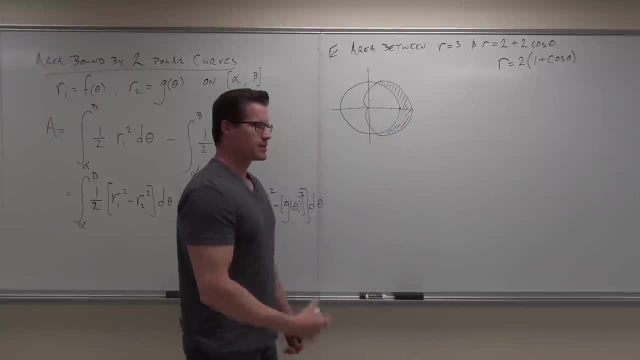 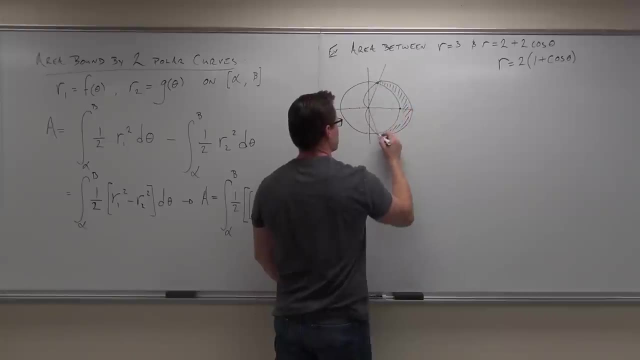 I'll look for that. Now, these things intersect. They intersect here and here. at those two points. We need to find out what these are. Here's why we need to find them. Think carefully on this stuff, Look at this, Look at, look at, look at. 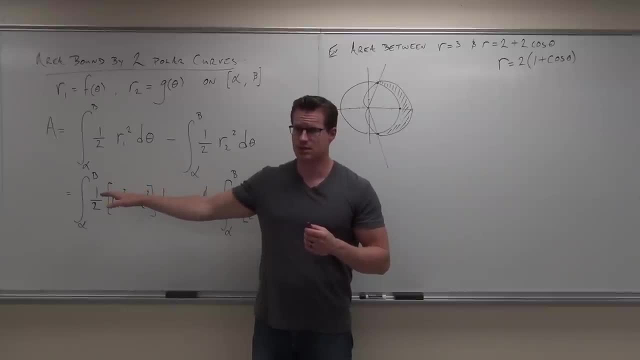 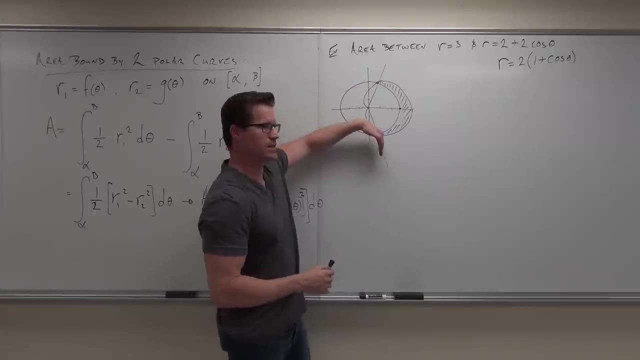 Notice that our equation here deals in angles. Do you get it? It doesn't deal in X and Y. It says: I need your starting angle, I need your ending angle. We need to find out the angle where these things intersect and the angle. 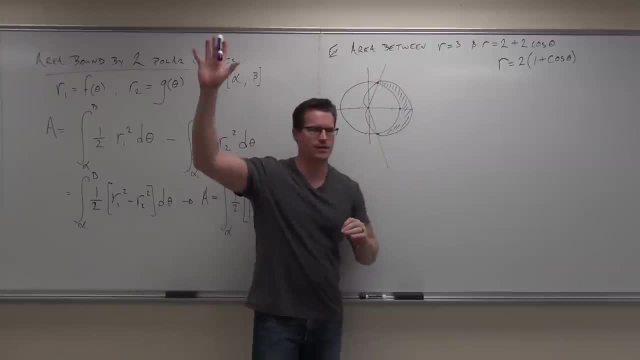 where they stop intersecting, where the intersection stops. Okay, Show of hands if you can understand that concept here. So, in order to do that, how would we do it? How do you ever find the intersection of two curves? What do you do? 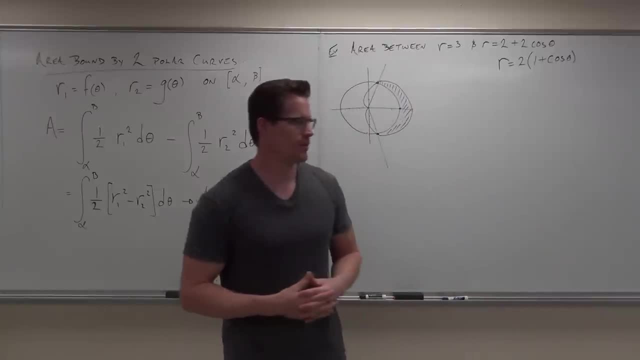 Check Nope. How do you find Nope? Usually in calculus, if you don't know the answer, you say: take a derivative, And you're right. In this class it's take an integral, But no, not this time. 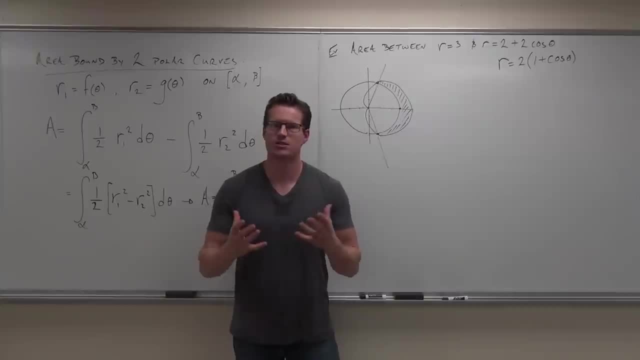 This goes back to algebra, actually. How do you find the intersection of two curves? people, You need to know. You need to know how to find where two lines cross. Make them equal to each other. Look at it, Hey, if R equals 3 and R equals 2 plus 2, cosine theta, could you make them equal to each other? 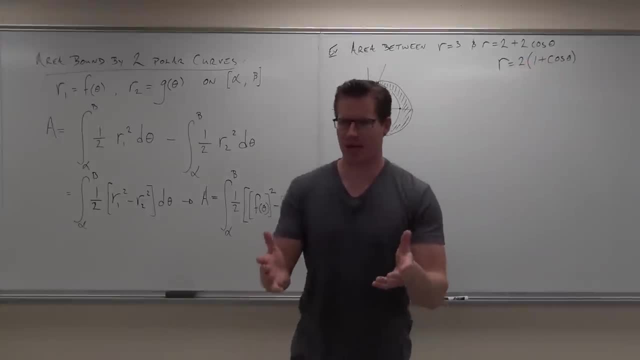 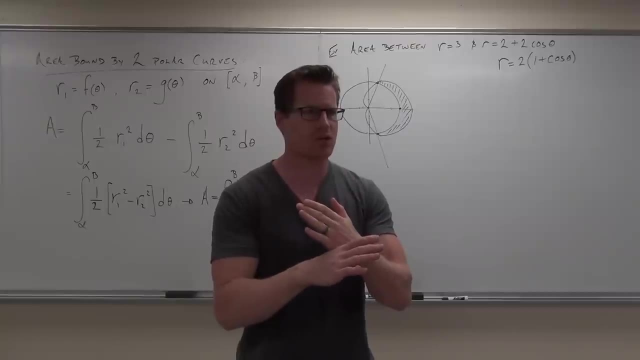 Hey, that's going to give you where they intersect. They always have. it always happens where, if you set two curves equal to each other, you're going to find out where they're equal, where they cross, where the intersection is. Click here now if you understand that concept. 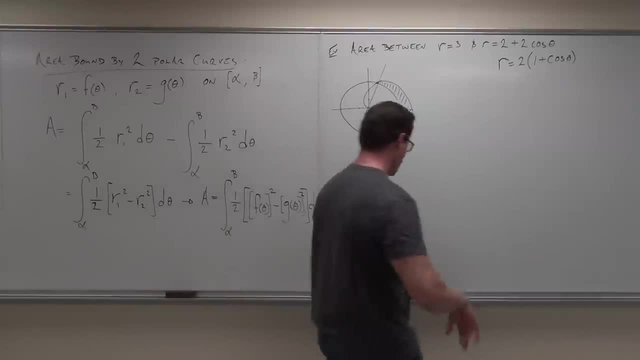 It goes back to algebra. If you ever want to find out where two curves intersect, set them equal. So we're going to set them equal to each other. We're going to find out what these intersections are. So setting them equal, 3 equals 2 plus 2 cosine theta. 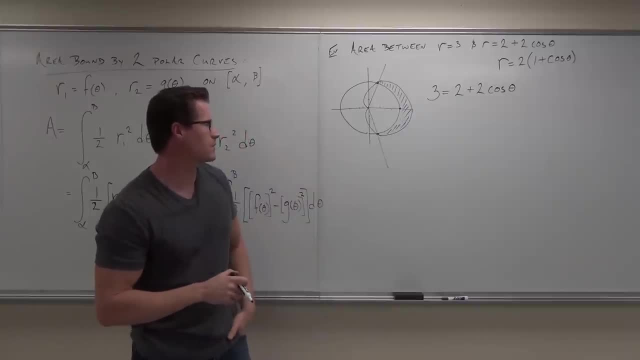 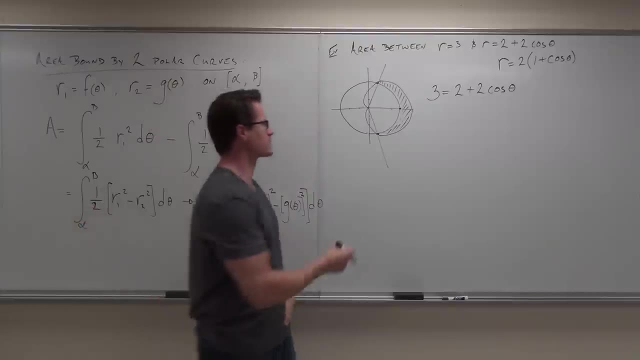 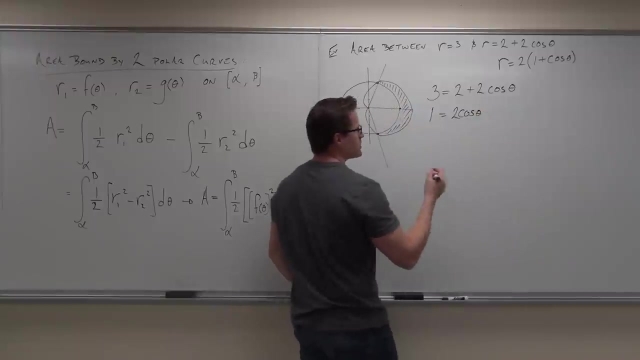 So far, so good. Solve it. How are we going to solve that? Probably a good idea. So we have subtracting 2, 1 equals 2 cosine theta Divide by 2.. So I'm going to flip the sides. 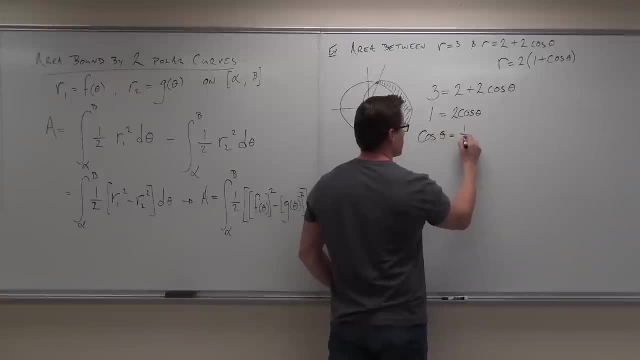 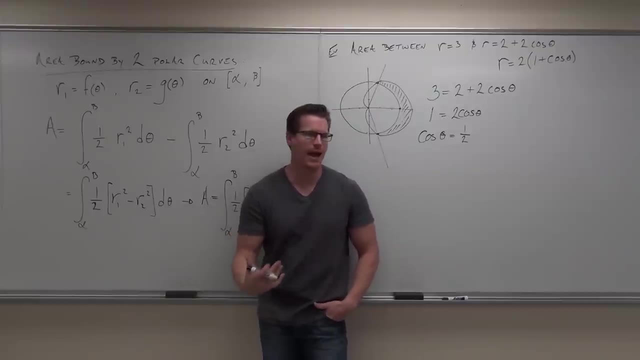 Cosine theta. Cosine theta equals 1 half. Now stop and look at your picture. This is why we usually like to have pictures here. Think about where cosine theta equals 1 half. If you know anything about trigonometry, you know that cosine equals 1 half. 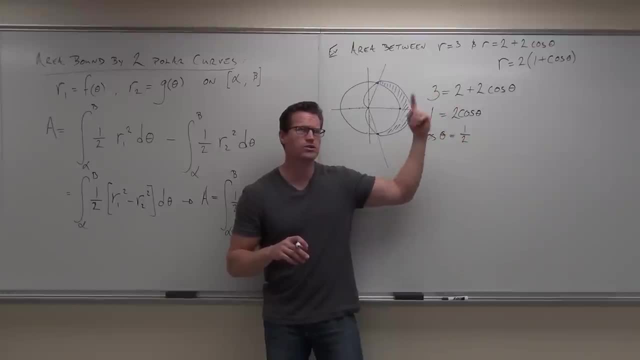 positive 1 half in quadrants 1.. All students take calculus quadrants 1,, but not 2 and 3, and then quadrant 4.. Does that make sense? That's where cosine theta equals positive 1 half. What is cosine theta equals positive 1 half for quadrant 1?? 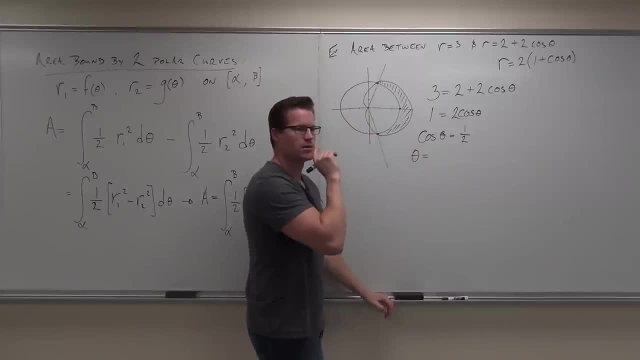 What's theta for quadrant 1? 5 pi over 3.. 5 pi over 3.. Very good, I had to think for a second. but yes, How about cosine? theta equals 1: half. for quadrant 4? 5 pi over 3.. 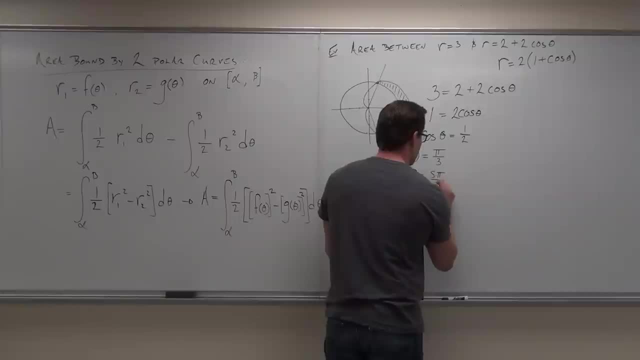 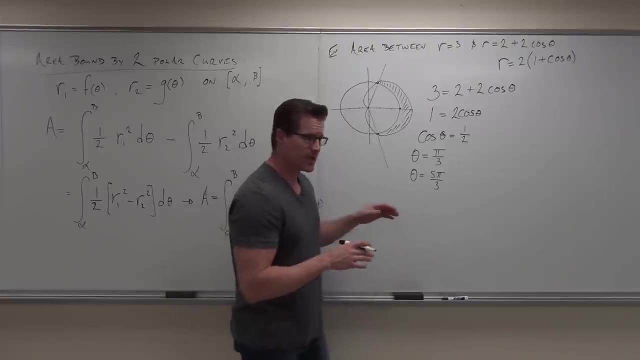 5 pi over 3.. That's right Now. I need to clear something up for you right now. Please listen. Please listen. We need this area right here. Are you with me? So what I need to do is I need to go from here to here. 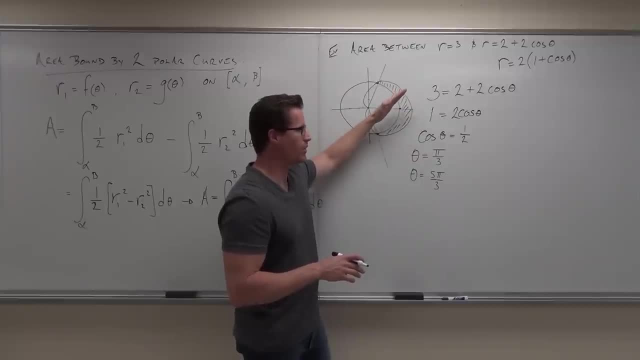 We're going to be going in the positive direction for angle change. Well, the problem is is, if this is 5 pi over 3 and this is pi over 3, can I possibly go from 5 pi over 3 and go positive and add up at pi over 3?? 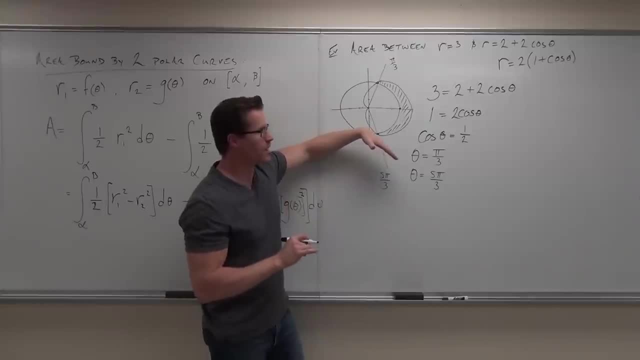 No, that's a bigger angle. That's a problem Now if I switch around and I go pi over 3 to 5, pi over 3, I'm going to get a positive angle. Remember that this is going to go positively in the positive direction. 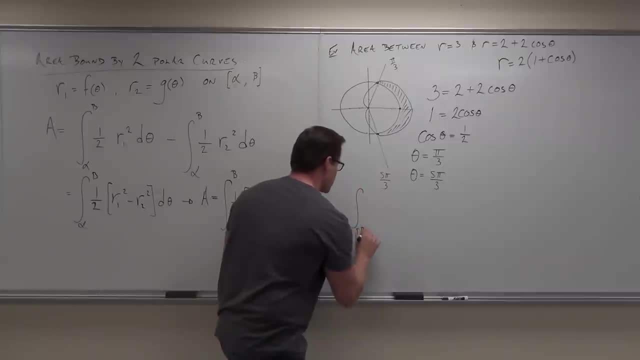 So if I set up my integral from 5 pi over 3 to pi over 3, I have a problem because I can't go from big angles to small angles and still be positive. Does that make sense If I go backwards and do 5 pi over 3 over sorry pi over 3 to 5 pi over 3,? 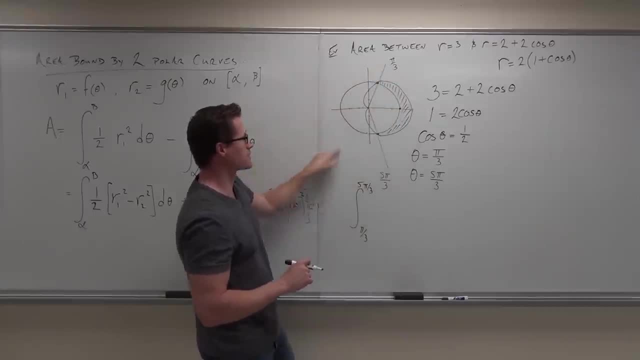 it's not doing this. It would actually be doing this. You'd find this area. Does that make sense to you? That's also another problem, and so we're looking for it. Okay, what we want to do is we want to start here and go here, but still gain angle. 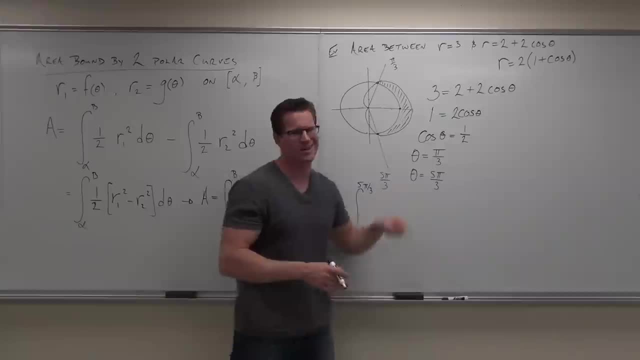 So still go in the positive direction. So instead of 5 pi over 3, what could I call that? Negative pi over 3.? Let's call it negative pi over 3.. That way I start here. That's still negative pi over 3, right. 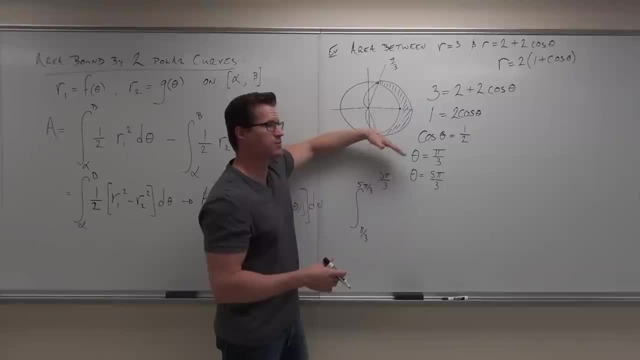 It's the coterminal with this. So negative pi over 3, I'm going to go positive to pi over 3.. That makes sense. and I'm also going for only this range, only that angular range. Show of hands, if you understand that concept. 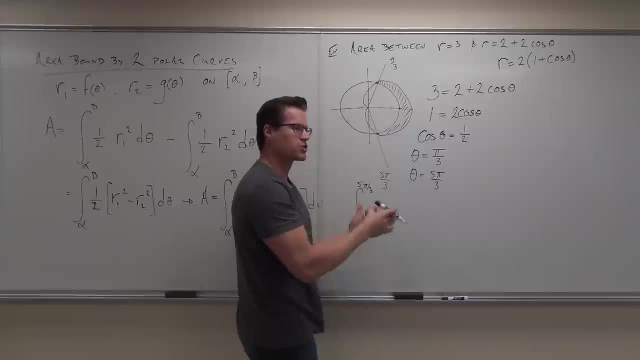 So you have to think about this. You have to think about what your quadrants are and what your picture really looks like. That's why we talked about graphing all these pictures, So we're not going to use 5 pi over 3.. 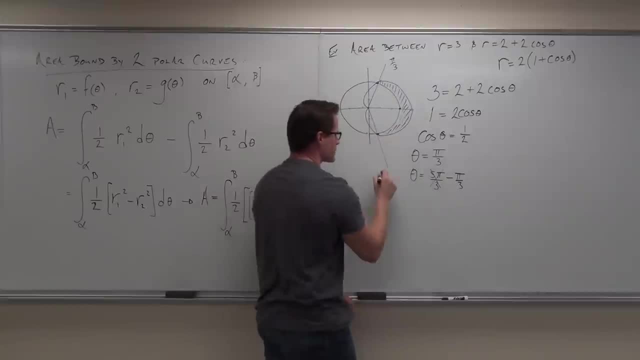 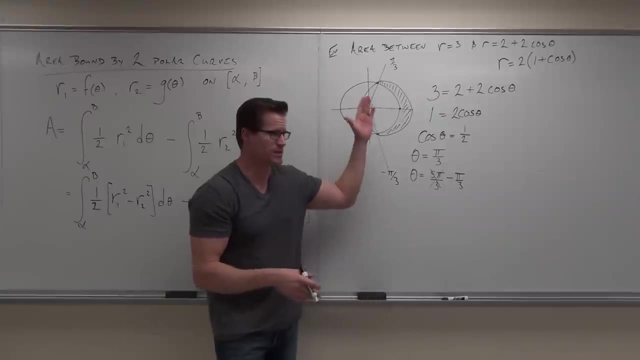 We're going to use negative pi over 3 because that will give me this. Did I explain that well enough for you to understand why we're not going from 5 pi over 3 to pi over 3?? Firstly, because we can't, because that doesn't make sense. 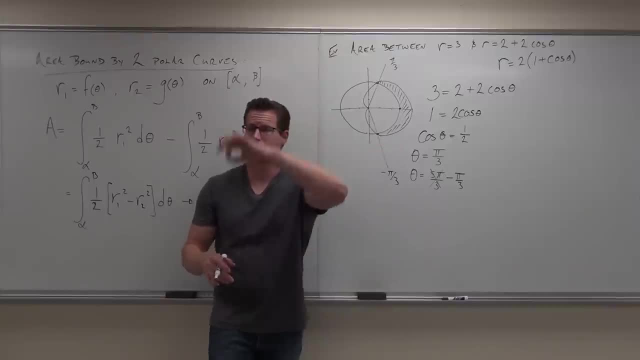 Do you understand why we're not going from pi over 3 to 5? pi over 3?? Yes, Because that's this way. That's this, that's not this area. This is the area we're looking for, So Let's go ahead and let's set this thing up, and then we'll work on the integral together, okay. 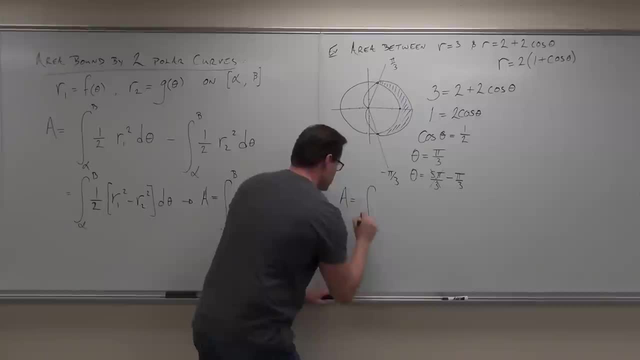 So our area. we're ready to go. Where's our integral going to start, please, Pi over 3.. Very good, Where's our integral going to stop? Pi over 3.. What am I going to have here? One half. 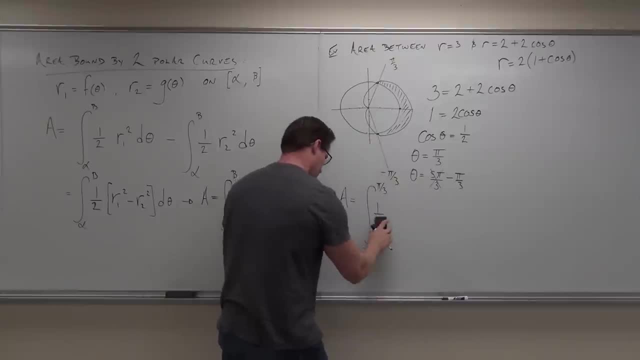 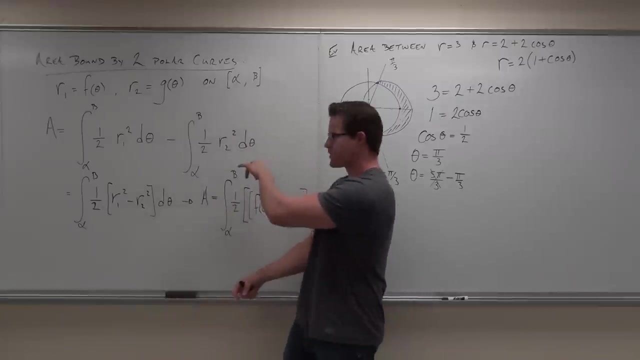 Okay, that's our formula: One half One. I just like threes. you know, One half. What's going to go first? Three: What's going to go first? Now? what's going to go first is: think about this when I gave you the curves over here. 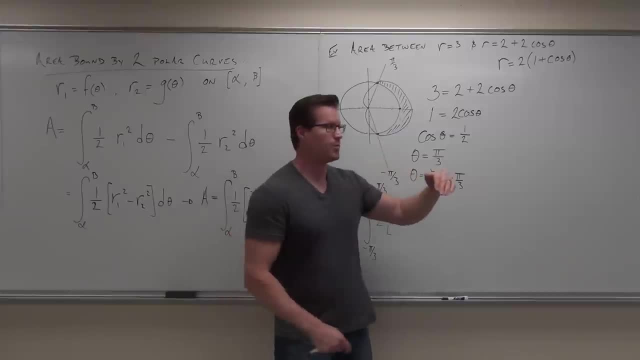 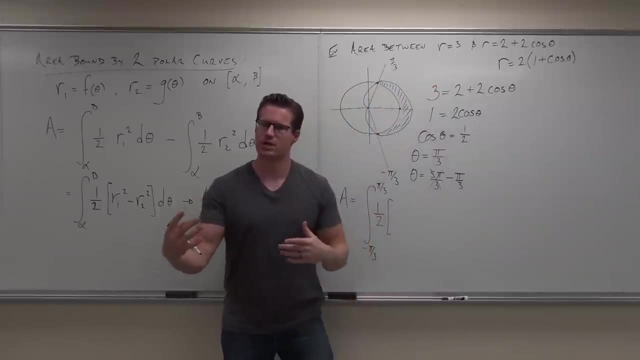 you took a big curve minus little curve. Big here means the one furthest away from the origin. So big curve minus little curve. What's the outside one? Is it the 3 or is it the 2 plus 2? cosine theta. 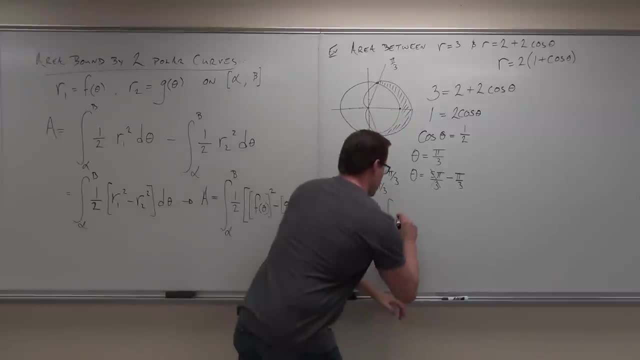 2 plus 2.. That's the outside one. So we're going to have 2 plus 2. cosine theta, Keep going. Come on, Help me out Square. Oh, the whole thing gets squared. That's going to be yummy. 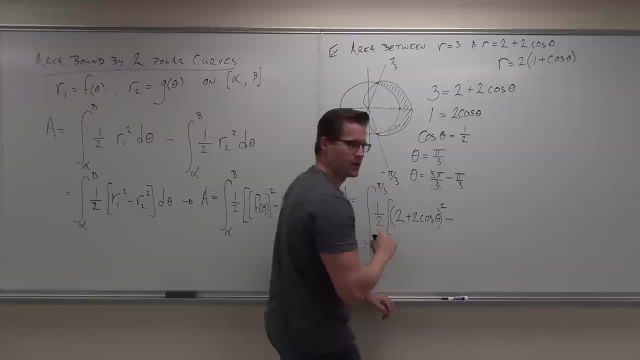 And then what Minus, what Three squared Perfect, because that's the inside one in this case. Okay, let's double check. Do you understand why we're going from negative pi over 3 to pi over 3?? Yes, no. See where the one half comes from. It's our formula. It's the area of the sector. We're just taking big sector, the most outside, minus little sector, the one most inside, and then we're integrating d theta. Show of hands, you feel okay? Now let's work on this one. What's the first thing we're going to do? We're going to integrate d theta. What's the first thing we're going to do? We're going to integrate d theta. What's the first thing we're going to do? We're going to integrate d theta Show of hands. you feel okay, Now let's work on this one. What's the first thing we're going to do? What's the first thing we're going to do If there's no questions, I'd like to move over here. 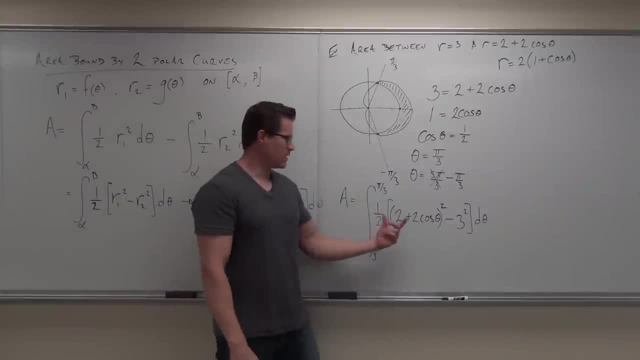 Do you guys have any questions on this? Okay, So I've got lots of space, I've got a lot of space, I've got a lot of space, So I'm going to do my first two cents. So I'm going to integrate d theta. Okay, So I'm going to integrate d theta. That's the first thing we're going to do. Who wants to do this? So let's do this again. This is not you know. say, I've got the third, fourth, fifth and I've got the seventh. 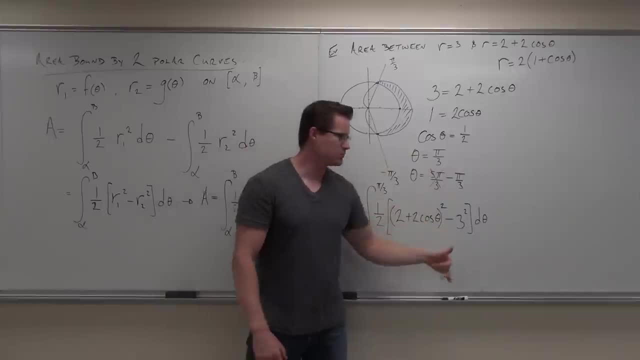 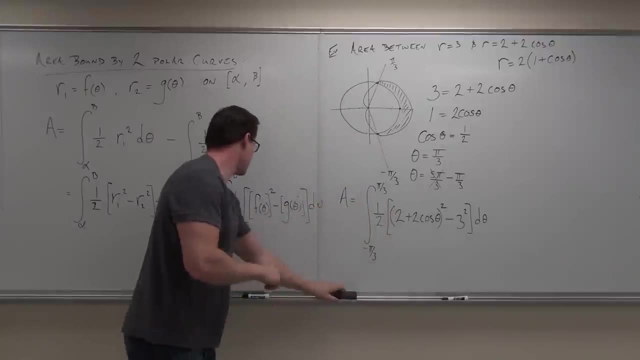 minus the little sector, the one most inside, and then we're integrating d theta. Show of hands. you feel okay, Now let's work on this one. What's the first thing we're gonna do? If there's no questions, I'd like to move over here. 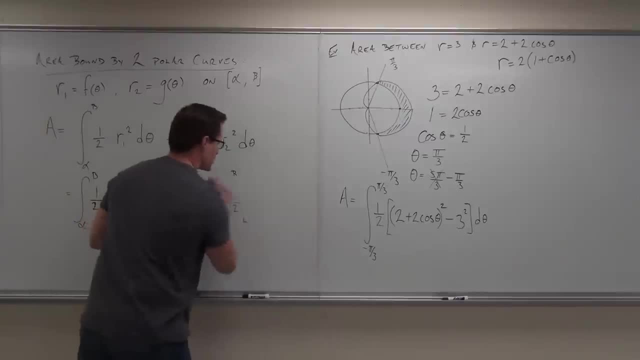 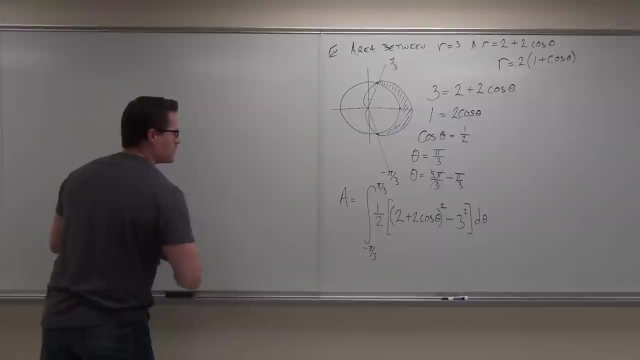 Do you guys have any questions on this? Okay, So I want lots of space. Okay, tell me, what are you gonna do? Go from zero to pi over three and just get rid of the one half. Oh, that's a good idea. 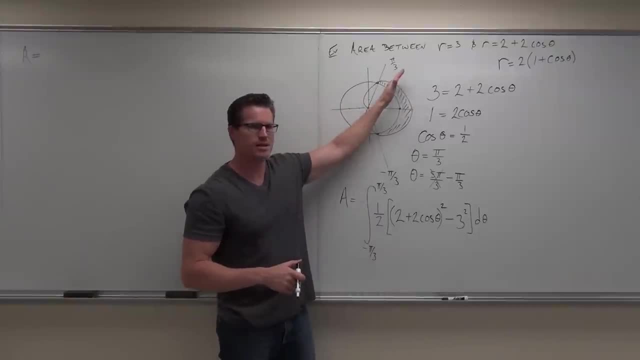 Why is that a good idea? So we could do this, couldn't we? Is this symmetrical? We know circles are symmetrical. We also know cardioids are symmetrical about the polar axis, So that means that our area is also symmetrical. 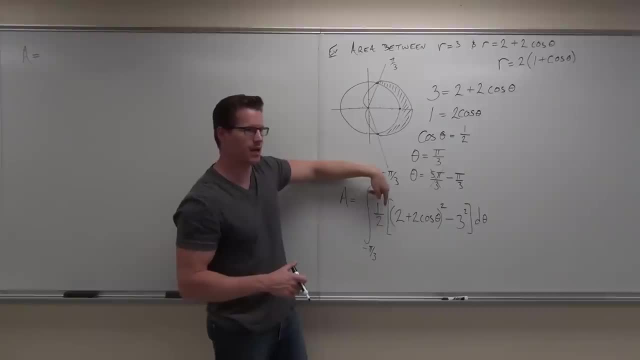 So if I wanted to, man, in order to get rid of that one half, that'd be kind of nice. Instead of going from negative pi over three to pi over three, let's go from zero to pi over three. Do you guys wanna do that? 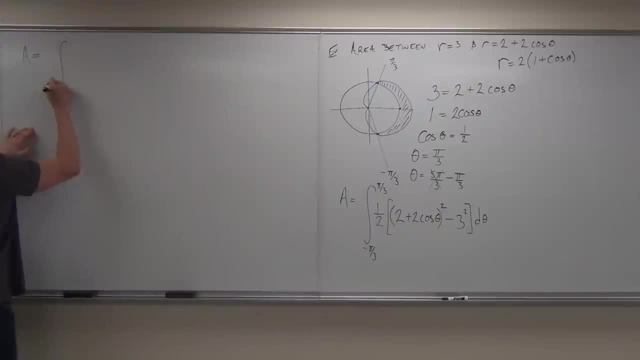 Let's do that, Okay. so if we go from zero to pi over three, then we still have one half and we still have all this stuff. I'm actually gonna distribute this right now. So we have four plus how much? 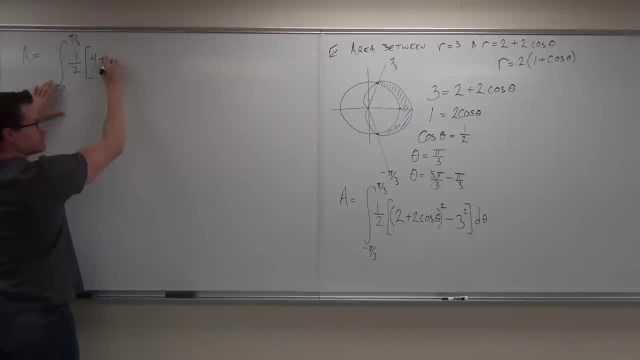 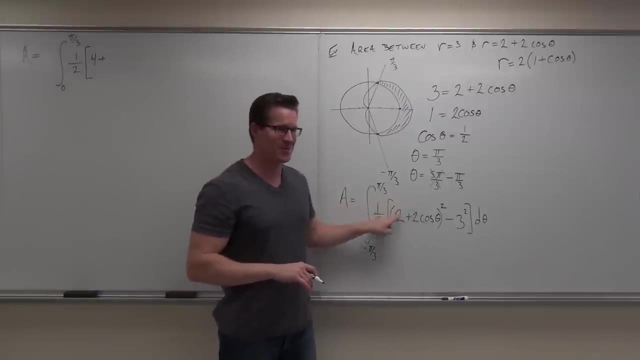 Four cosine squared: No, Well, that's gonna be up there, Yeah, but what's the next thing? Let's try distributing this correctly. okay, We have four. Then we have how much? Four cosine theta: No, Eight. 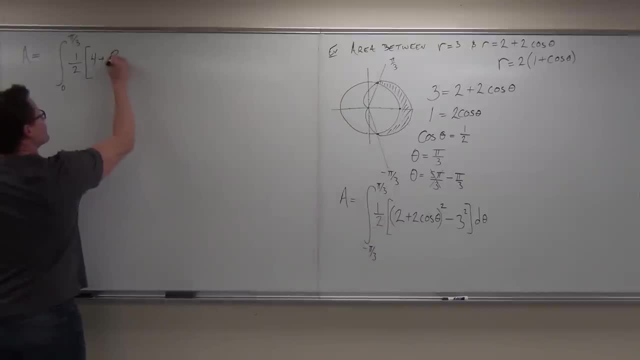 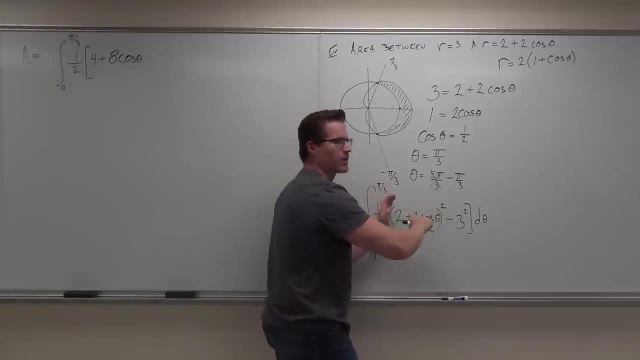 Eight cosine theta. Do y'all see where the eight cosine theta's coming from? If you distribute, it's this times itself. So we got four, then we got two, and, okay, we got four and four. That's eight cosine theta. 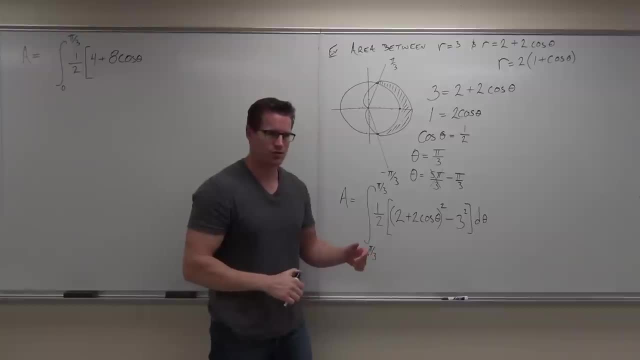 Then we have our four cosine theta. If you don't know how to distribute these quickly, you just square this, multiply, this, multiply by two and then square that. So we're gonna have four cosine squared And then we're gonna have minus nine. 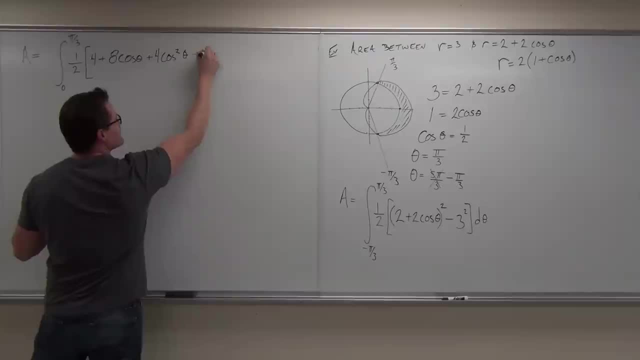 and then we're gonna have a d theta. Now we talked about something here real quick, You guys. okay, Since we changed bounds, wouldn't the one half disappear? We're talking about that right now actually. So I want to make sure you guys are clear. 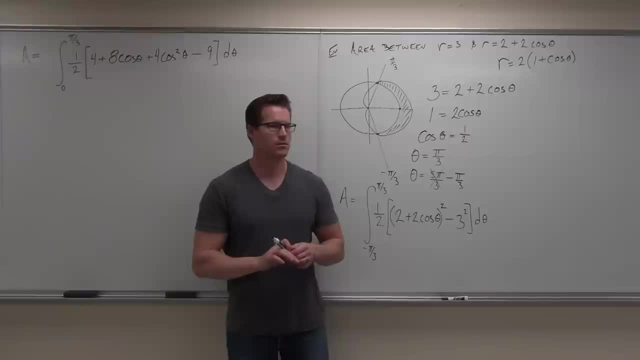 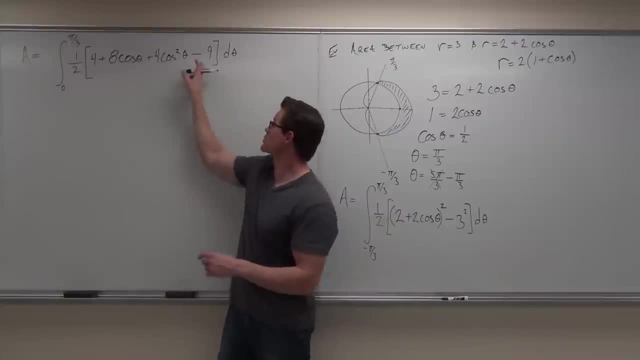 Yeah, Yeah, Yeah. All right. Now this side is a square. We're distributing this, We're just squaring our nine. Now what we did? we changed our bounds. We're not going from negative pi over three to pi over. 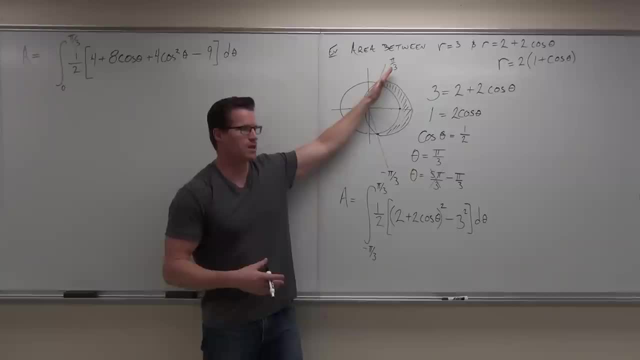 three anymore. We're going from zero to pi over three. If we're going from zero to pi over three, that's only giving us half of the area we want. How do I make this thing fit that? Multiply the two to two. 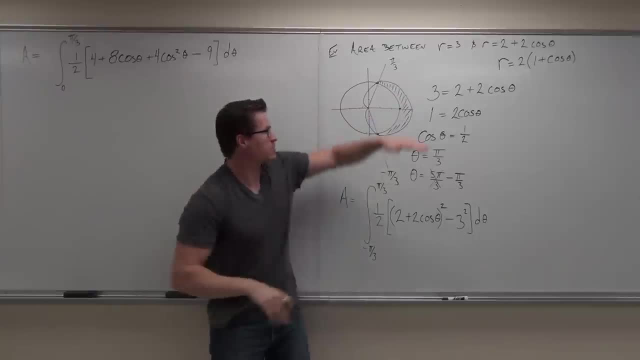 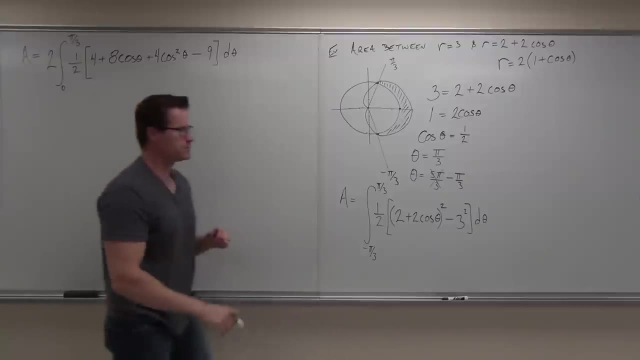 That's right. So what this is representing right now, the way it is, it's representing this area. If I want all the area, I just times it by two, because it's symmetrical. Does that make sense? Okay, now let's start working on this thing. 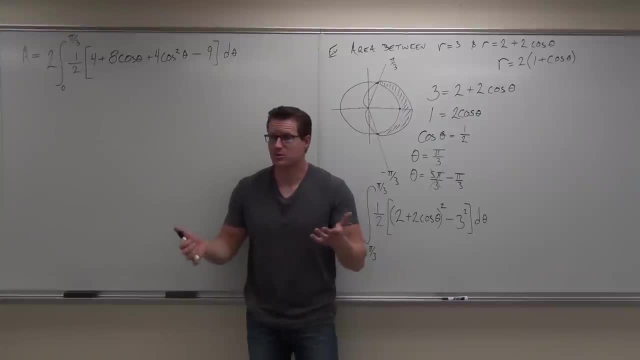 A couple things we can do. What's going to happen. That's kind of one of the reasons why we did this, because, firstly, 0 is nice to plug in rather than negative pi over 3, so when we get to the very end, I don't want to have to do that. 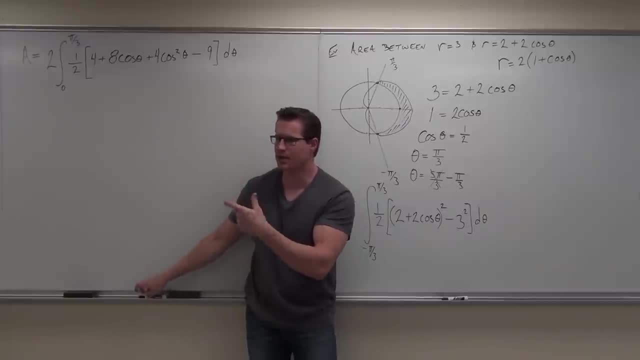 So 0 is nice. Also, it's getting rid of all of our constants that we have outside of our integral. So we've got 2 times 1 half gone. Also, maybe we can combine some like terms here. So we've got area equals 0 to pi over 3 in our integral. 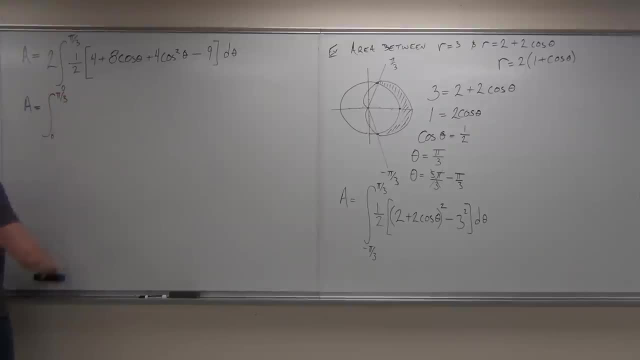 We're going to have 4, actually we're not. What are we going to have? Not 5.. Plus 8 cosine theta, plus 4 cosine squared theta, and then d theta. all that stuff, Easy, medium, hard. what do you think? 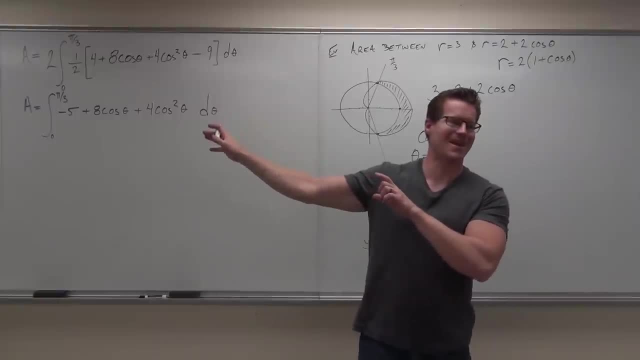 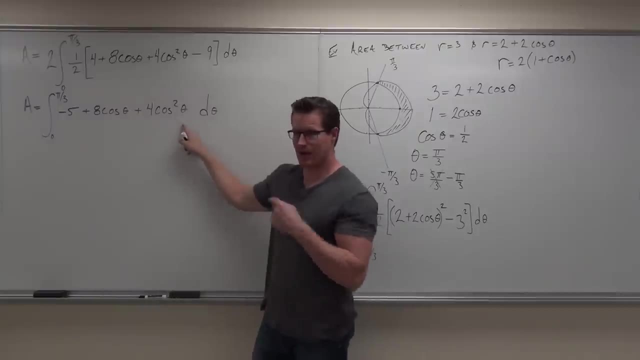 Doable? Have you seen this before? Oh yeah, Can you integrate that Piece of cake? Can you integrate? Can you integrate this Piece of cake? Can you integrate this? Yes, Right now, the way it is, No. 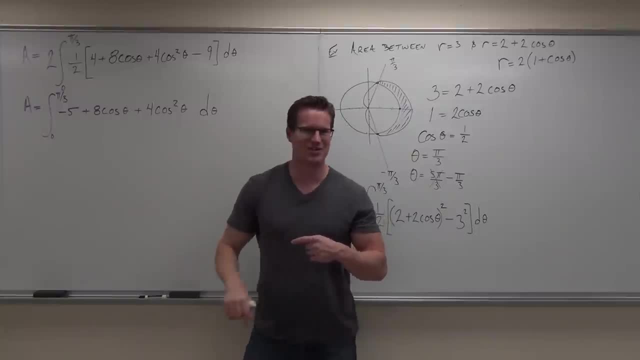 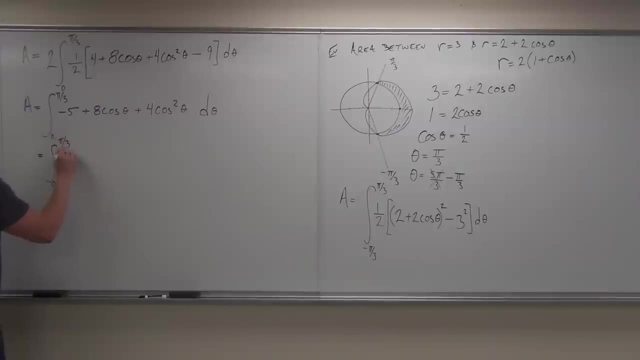 No, Can you change it? Yes, Yes, Oh, you guys are the yes crowd. I forgot about that. No, Or yep, Yep, Yep, Yep, Yep. No 1, half 1, plus cosine 2, theta d theta. 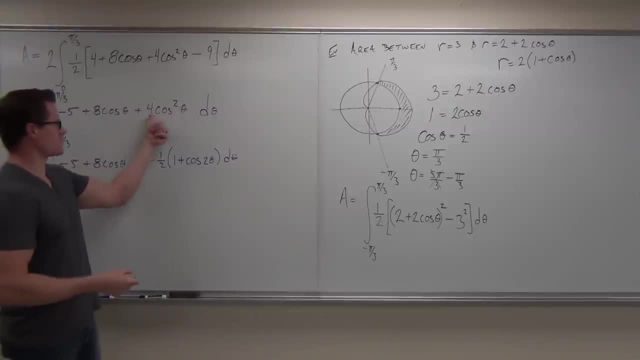 Yeah, we're going to use that identity. So this says: well, keep it, for this is 1 half times 1 plus cosine 2 theta. What's nice for us, we've got even numbers. So 4 times 1 half is 2, we go all right, cool. 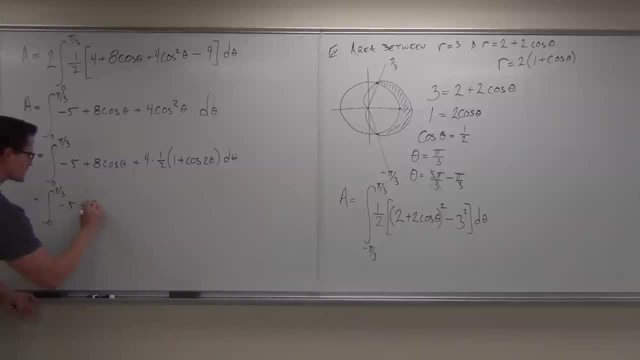 We've got 0 to pi over 3.. We've got negative 5 plus 8, cosine theta plus 2.. If this whole thing is 2, then I have 2 plus 2 cosine 2 theta. I know I'm doing a couple steps at once. 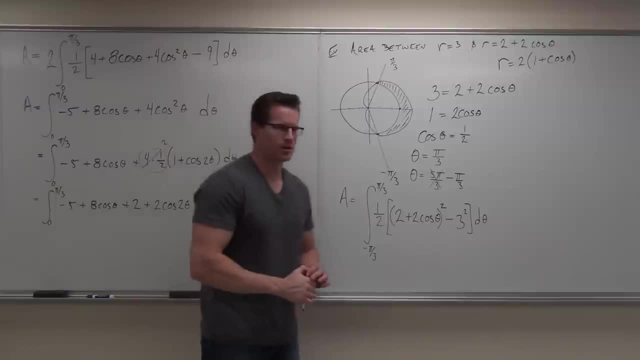 I'm simplifying and I'm distributing. Are you guys okay with it? Okay, Why don't you go ahead and see if you can do the? actually, you know what we might want to do. one more thing: What's the last thing we might want to do? 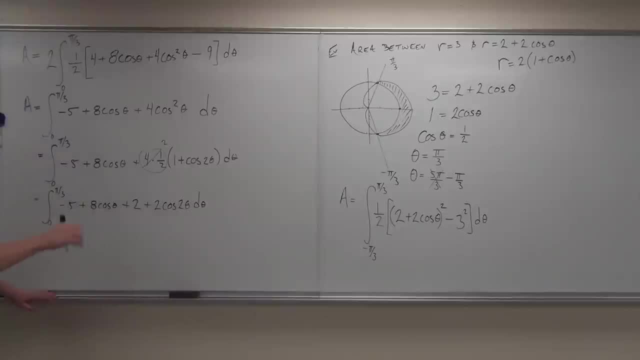 Probably combine these guys. So let's do that. and then I want you to integrate it. So here's the last thing. oh, hold on, here is the last one. I like to do one more thing. Here's the last thing. 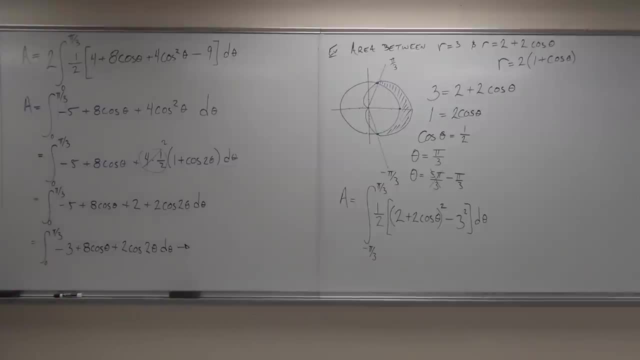 Say: oh, I want to do 1 half times 1 plus 3 plus 2 theta. Okay, 2 times 2 theta plus 2 plus 3.. Okay, We're going to multiply that by 2 times 1 plus 2 theta. 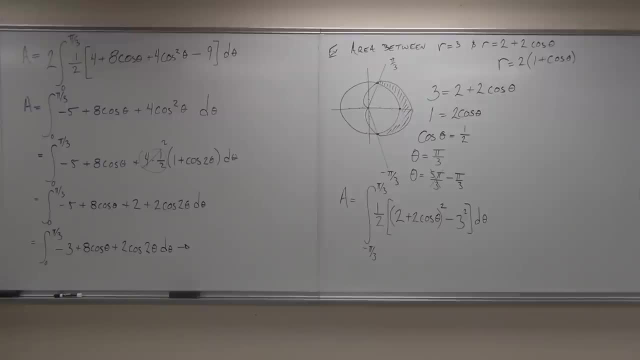 Yes, that was easier. What do you guys think? It's a little bit hard. I guess we should just do it one more time. Go ahead, All right. All right, All right. Did you integrate it? How many people did integrate it? 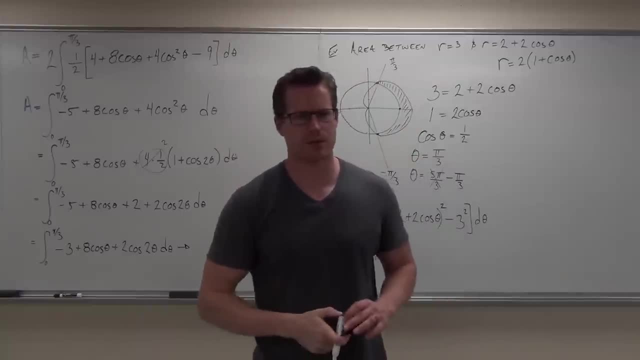 You got it. How many people did? I'll give you some more time. I want you all to integrate this. It shouldn't take you long. I don't care if you evaluate it, I want you to just integrate it, Just get the integral done. 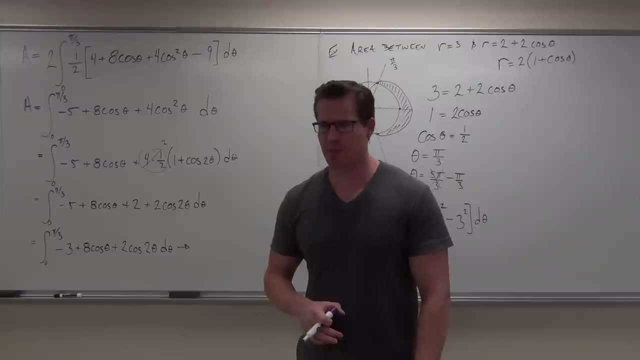 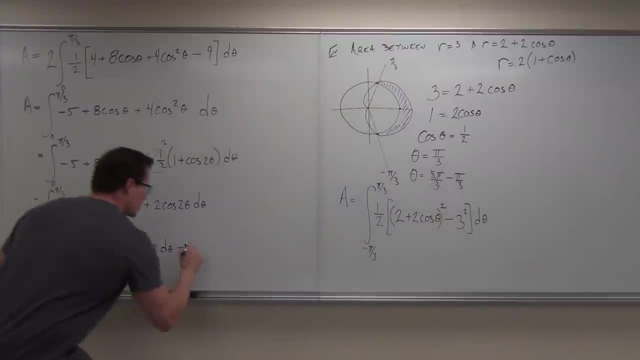 We'll evaluate this together in just a minute. So, as long as you get the integral done, that's what I care about. Have you got the integral done yet? You guys over here, yes, no, Okay. So if we integrate here, we're going to have- remember it's d theta. 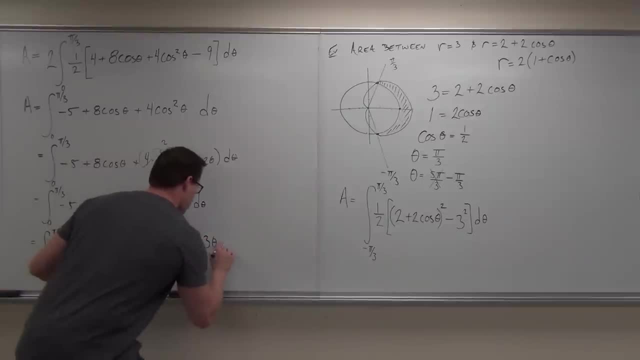 So we're going to have negative 3 theta. We're going to have plus 8 sine theta. We're going to have plus cosine, I'm sorry- plus sine 2 theta. Actually, what you get is 2 sine 2 theta over 2.. 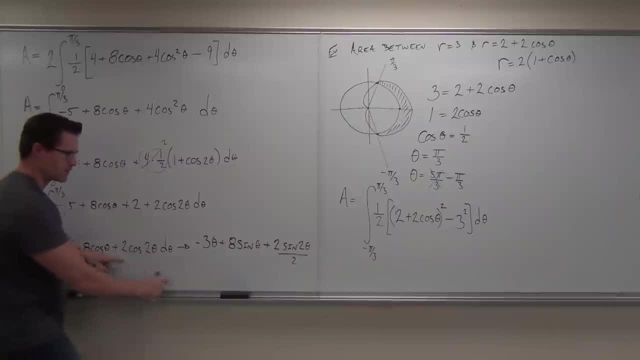 You get 2 sine 2 theta divided by the derivative here, but your 2s are going to be gone, So it depends. if you made it that far on your own, That's great. That's fantastic. So I'm going to raise my 2.. 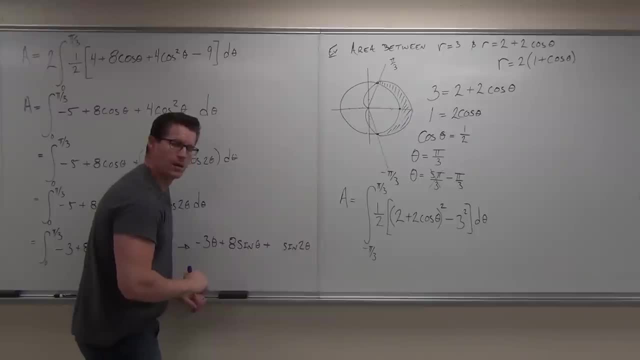 I'm going to raise my 2s. Now what Say what? Where does it start? It's kind of nice to have a 0,, isn't it? So we don't have to plug in all those negative pi over 3s to all this stuff. 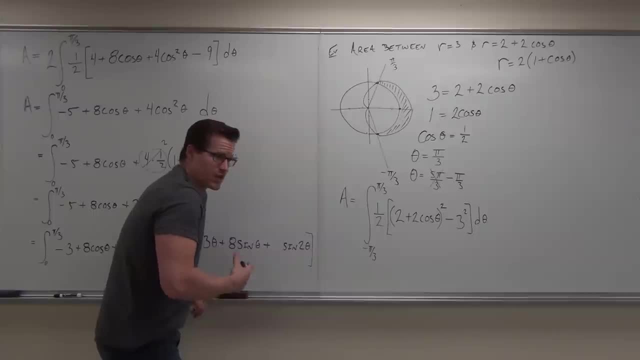 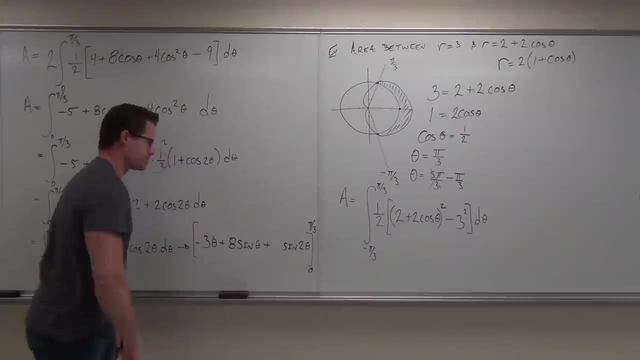 because that would be kind of, that would be nasty And we could do it. It would be the same answer, but we don't have to now. Which one do we plug in first? So we're going to plug that in And we're going to get negative. 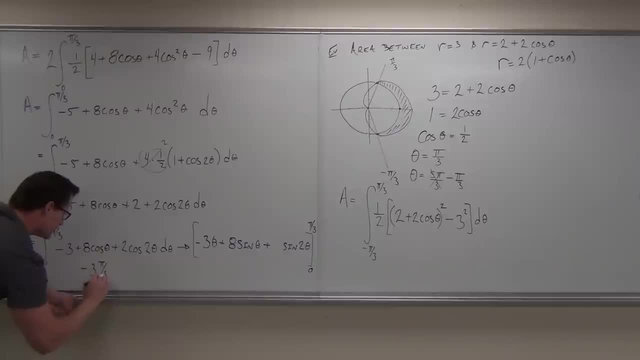 So we're going to get negative pi over 3 times pi over 3 plus 8 sine pi over 3 plus sine 2 pi over 3 minus. Now let's check this. okay, Don't make the mistake of just leaving this hanging out, okay. 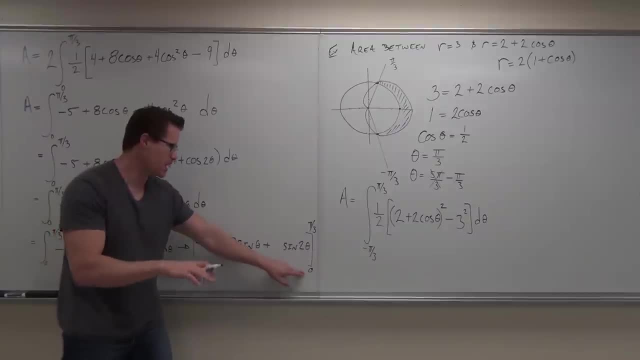 A lot of people, especially students, who are just coming through this the first time or something. when they see 0, they just go, oh, it's always going to be 0. That's not true. If you had cosine here, it's definitely not going to be 0. 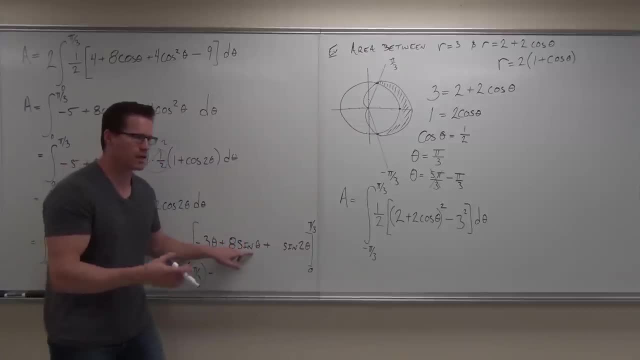 Now 3 times 0, okay, Sine of 0,. okay, Sine of 0,. okay, So all the rest of it's going to be 0, but you do need to check this. Does that make sense? 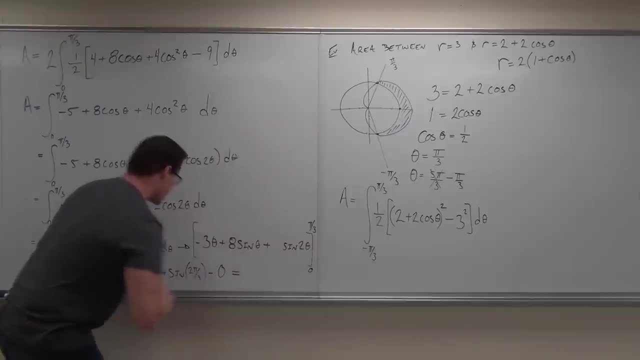 So this is all 0, yes, So minus 0 gives us. well, let's think about that. What's negative 3 times pi over 3? Negative pi, Negative pi. Okay, How about sine of pi over 3?? 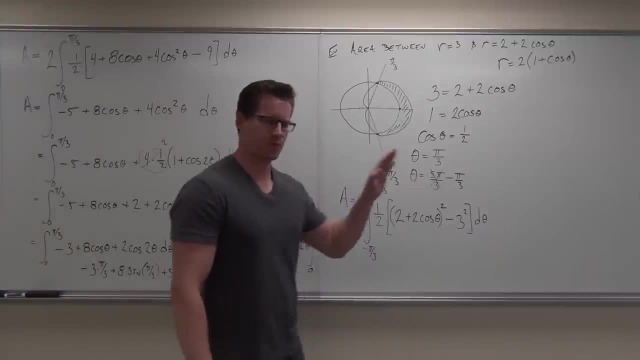 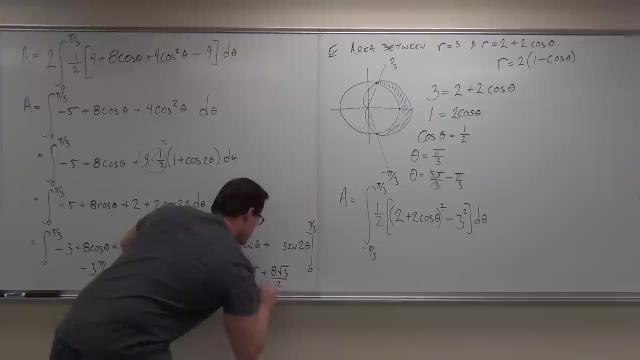 Do you know what sine of pi over 3 is, 3. 3 over 2. 3 over 2.. So we have plus 8 root 3 over 2.. We'll simplify that in a minute. And then sine of 2 pi over 3.. 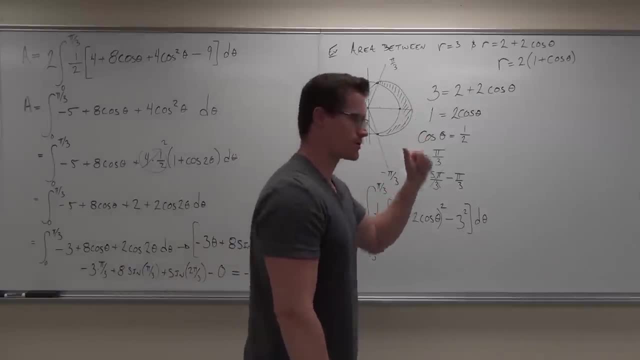 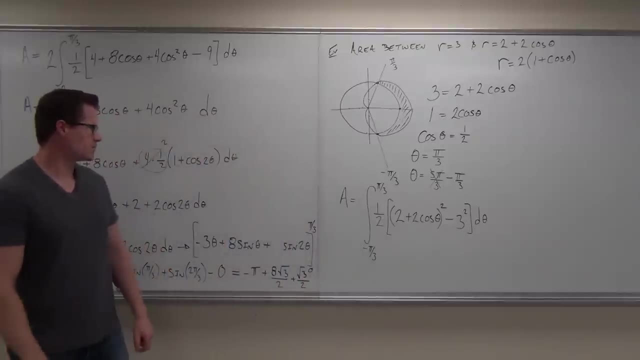 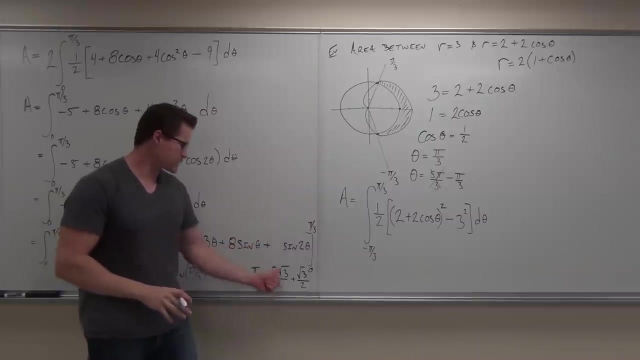 What's sine of 2 pi over 3? 3 over 2.. That's right. Could your hands feel okay with that? so far, Now you can choose to do a couple things, but I probably wouldn't do this. I wouldn't simplify this right now. 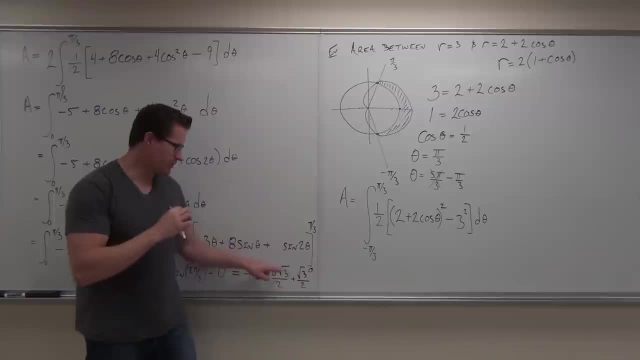 Because right now we have a common denominator and we also have a common root. So if I have 8 root 3 over 2 plus root 3 over 2, that's 9 root 3 over 2.. Does that make sense? 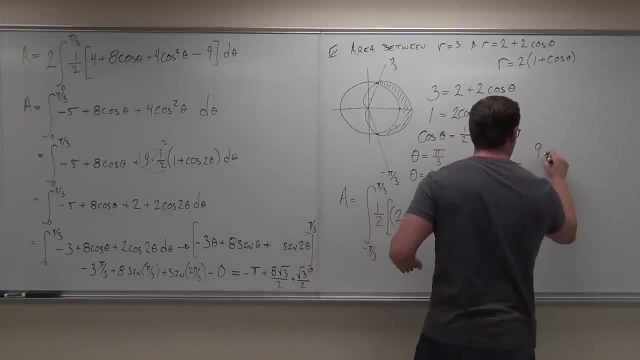 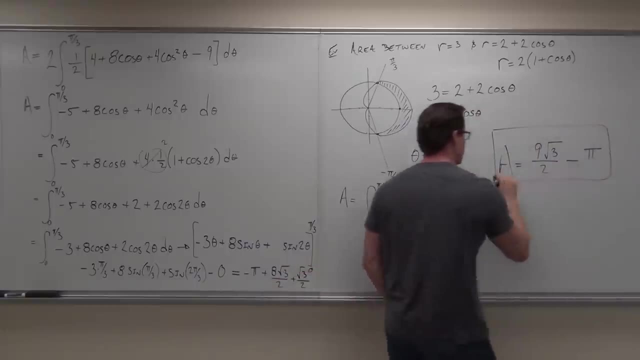 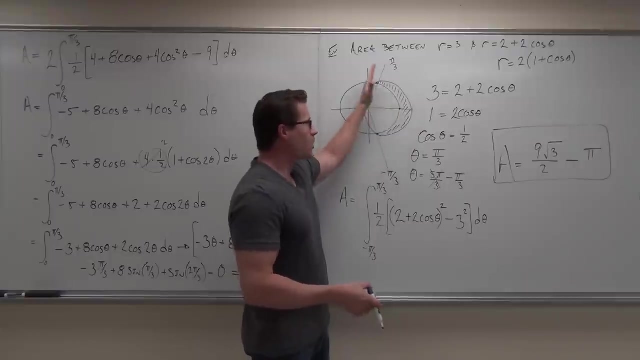 So our area equals 9 root 3 over 2 minus pi. Not a nice looking area, but we found it. That's kind of cool. So the area between a large heart, a large column and a large column, that's 9 root 3 over 2.. 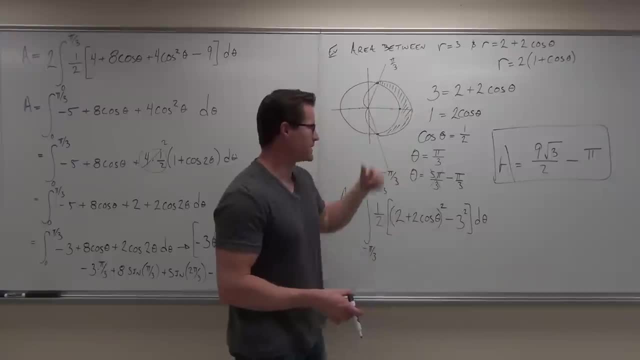 Or a large cardioid and a circle. this particular circle is 9 root 3 over 2 minus pi. Could you find an approximation for that if I asked you to? Yeah, That's the whole idea, So your hands should be okay with this one. 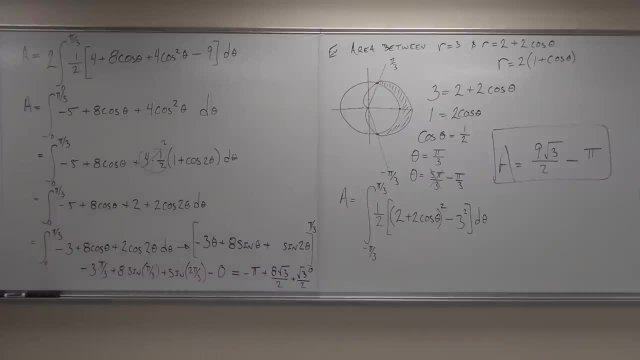 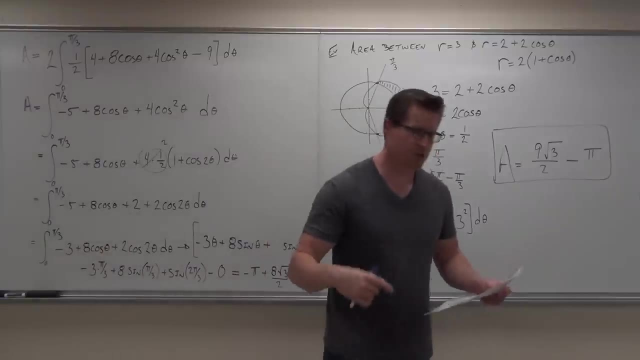 All right, Tell you what The last thing that we're going to do in here. I'm going to give you some formulas on how to find arc length, on how to find area of the surface of revolution. It's going to be really similar to the stuff that you've done before. 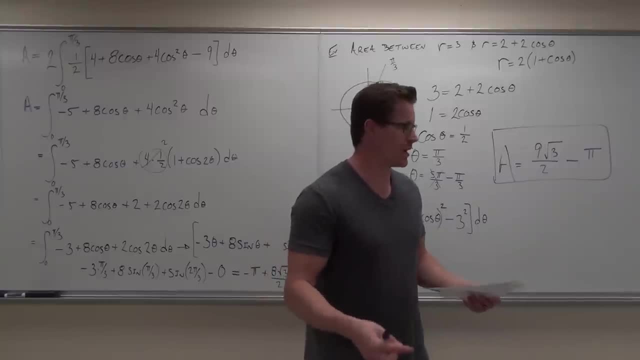 I'm not going to give you examples on that. There's formulas that you will know how to plug stuff in for. okay, You know how to do integrals, right. You know how to plug stuff in, right. So it's going to be just formulaic at this point. 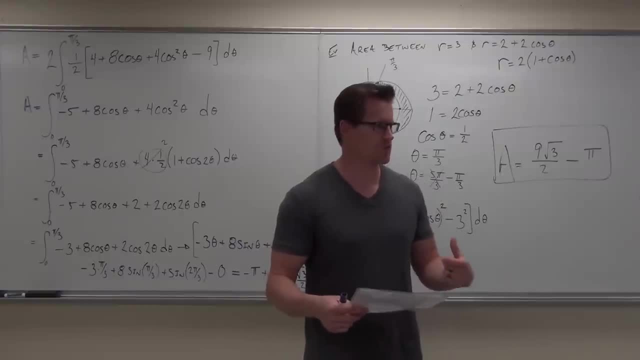 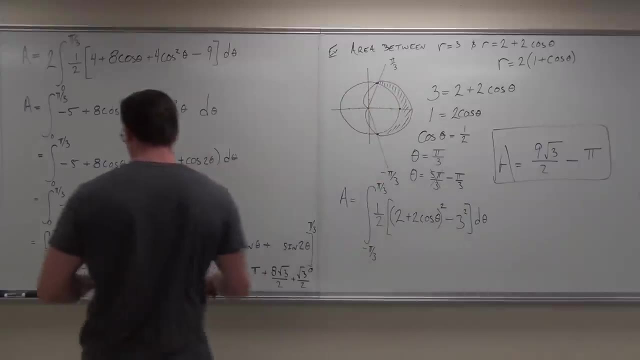 After that, I'll show you how to find the intersection between two polar curves, which is very useful like this sort of stuff, And we'll talk about some interesting things that can happen. So just a couple of formulas at first, but do you have any questions on this before we continue? 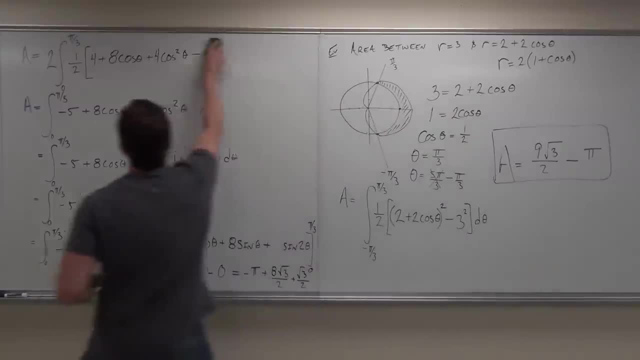 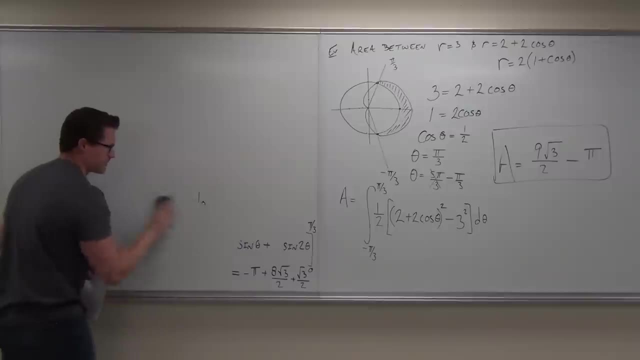 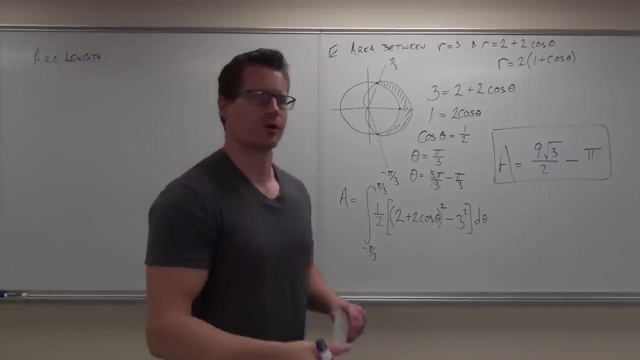 Have X-Line this one on for you guys to get it Okay. So a few other calculus concepts dealing with polar equations, And the first one is arc length. To find the length of a polar curve you can use this formula: Arc length is the integral. 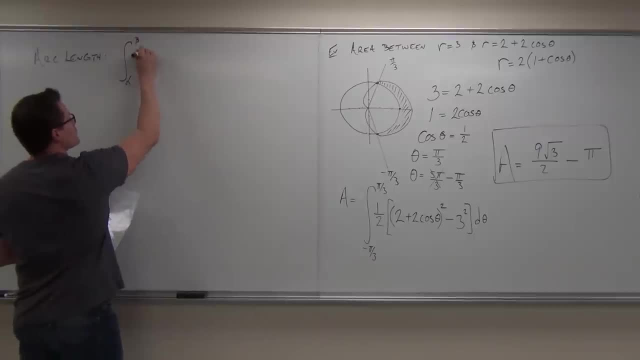 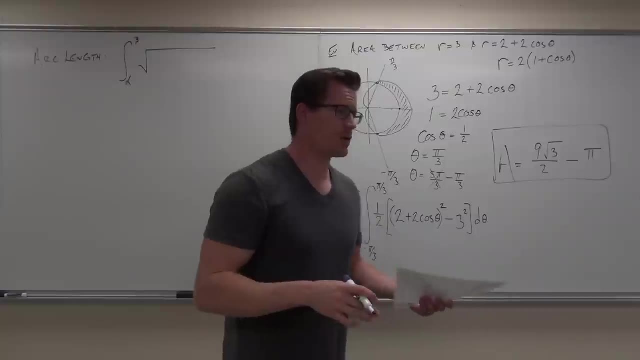 Alpha to beta. those are our angles. Square root- so far does that look familiar? the square root? Do you remember any time we've ever found the length of a curve, we've always had a square root. No, In calculus one it looks like this: 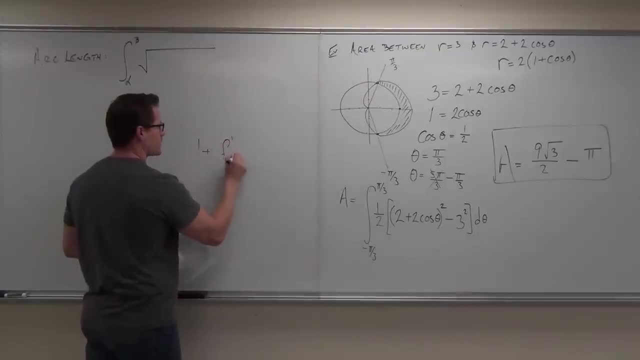 Okay, So we're going to find the length of a curve. We've always had a square root. In calculus one it looks like this: It's 1 plus f, prime of x, squared under that square root. Do you remember that? 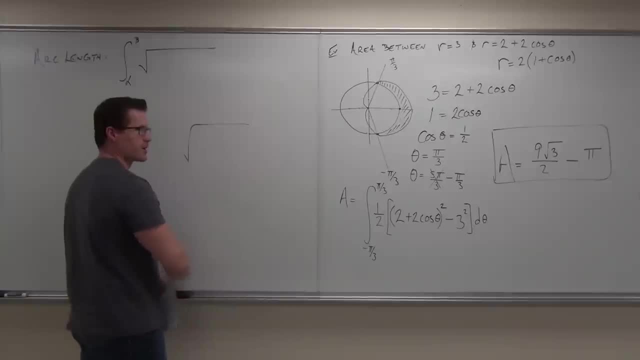 That's how it looks For parametric. it was dx dt squared plus dy dt squared. Remember that For us it's going to be similar to this one. What we do is we take a square root and we do dr d theta squared. 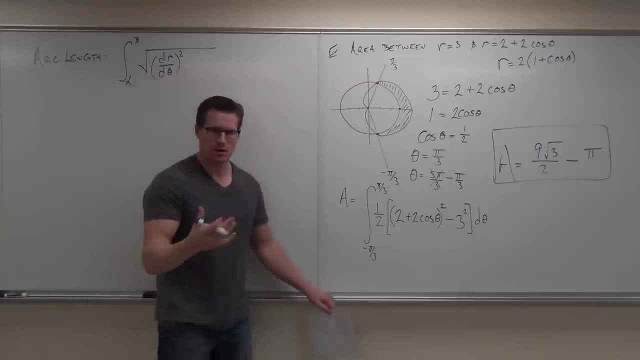 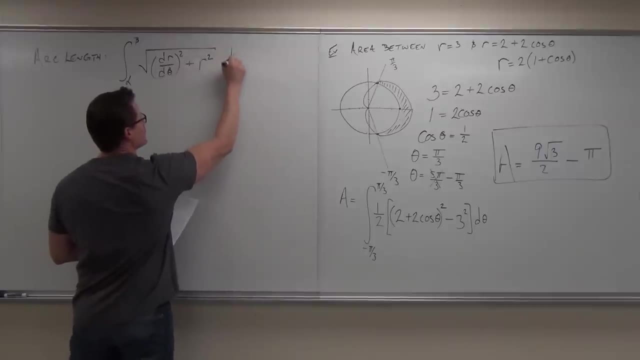 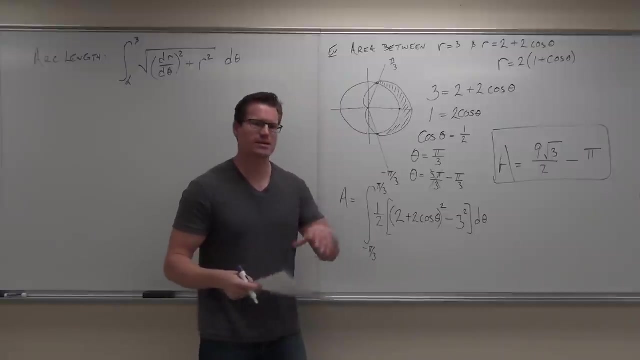 So far it looks very, very similar to: And then we do just r squared. That's where it changes just a little bit, Because our r is a function of theta. we have a little bit different of an idea than parametric, But that's the idea of arc length. 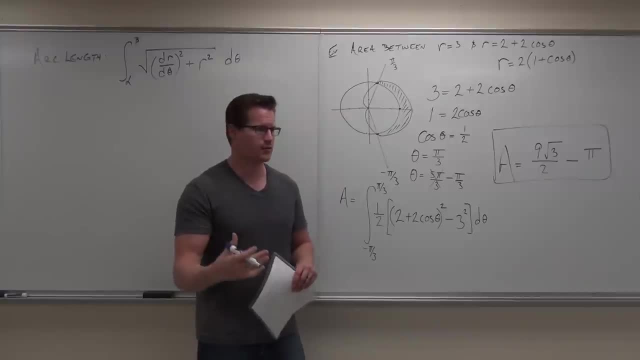 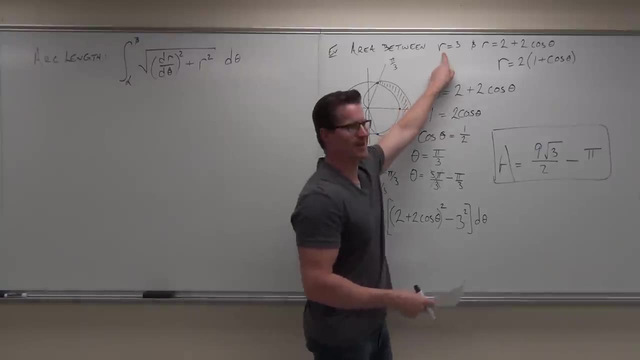 Could you, if I asked you, to find the length of a curve between two angles? Sure, What are you going to do? Well, the first thing you're going to do is take, like not that one. okay, that's pretty easy. 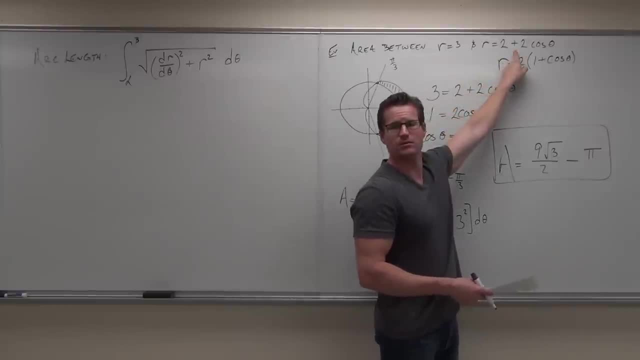 But Like that, one First thing you do is do what? Take a derivative with respect to theta, Then square it. Not a problem, That'd be pretty easy to do, wouldn't it? So take a derivative, square it Then. do you know how much r is? 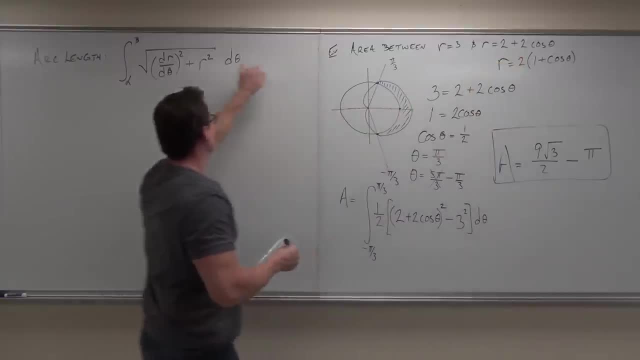 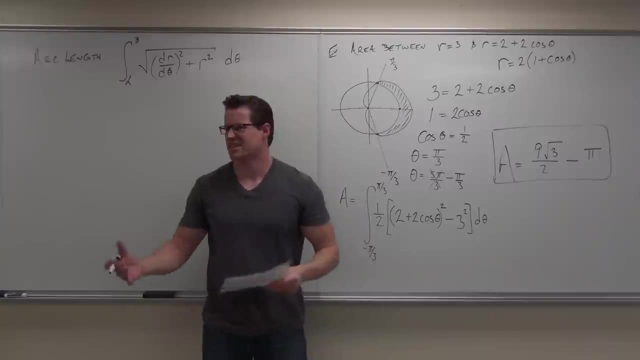 Yes, I'm sure you do. Take the r, plug it in square. it. Combine your like terms, figure out how to do the integral. It's under square root, so you might have to use some manipulation there, But that's the idea. 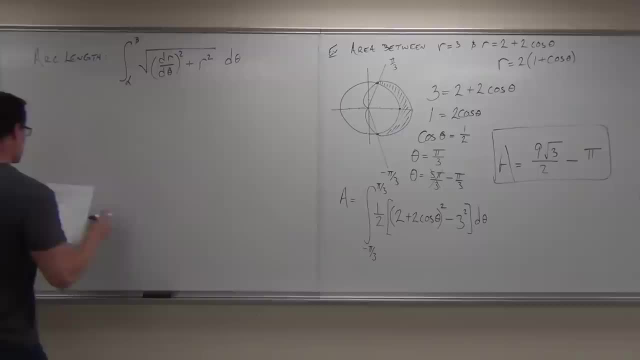 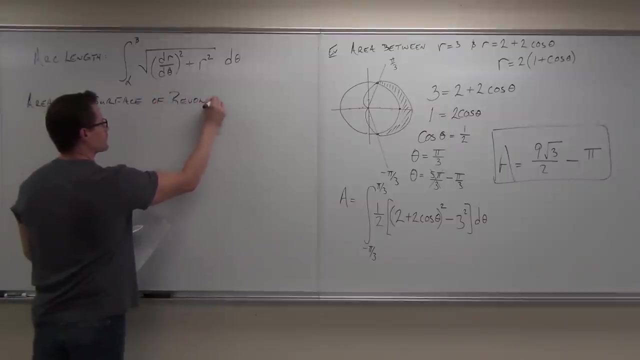 Feel okay with the idea, Not a problem, All right. So How about area of a surface of a rectangle, Revolution, Revolution. We'll talk about the polar axis. Polar axis And then about theta equals pi over 2 axis, or well, pi over 2y. 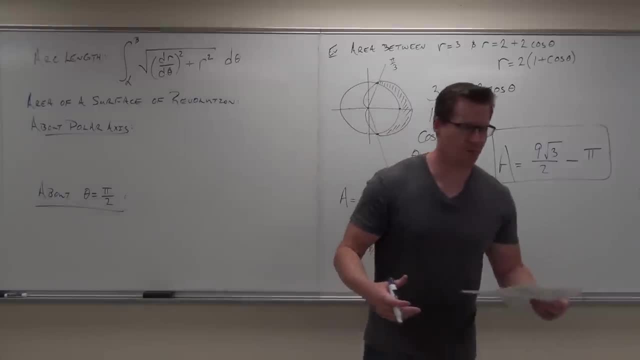 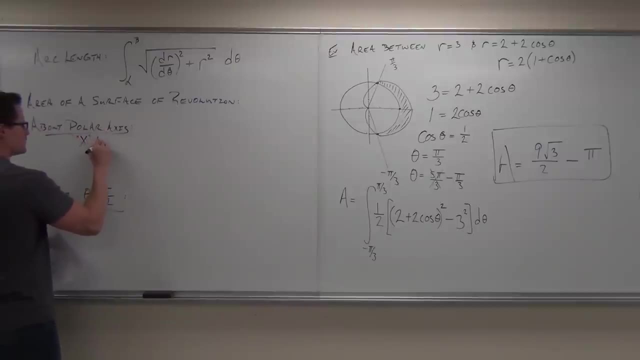 Which one do we usually call the polar axis? What is that? The x or the y X? Yeah, it's like the x axis And the pi over 2, that's like our y. Now, of course, we don't really have those in polar equations, but we can think of them. 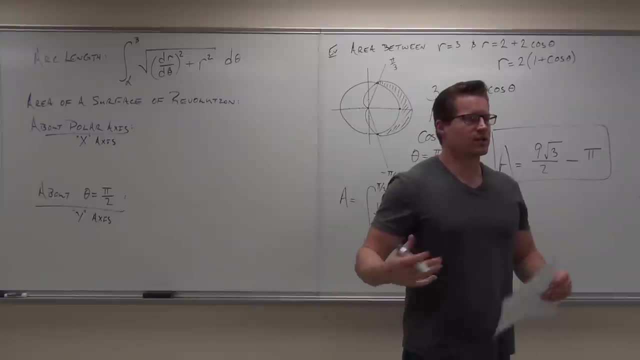 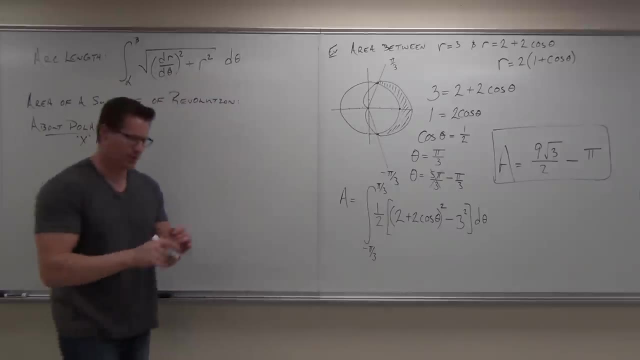 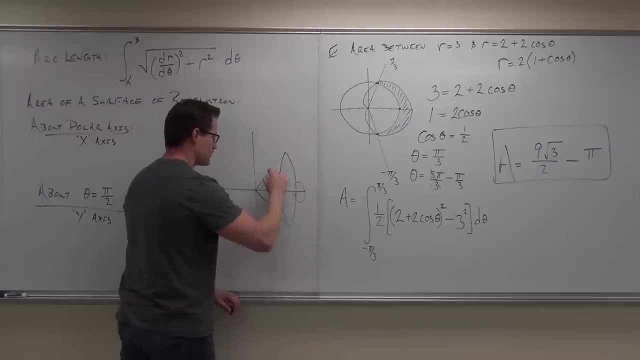 like that for this instance, because I want you to, I want you to really consider where we get these, Where we got all of our surface of revolutions, surface area of revolution. we got this. We said, okay, if I'm going about, if I'm going about the x axis of some curve, well, 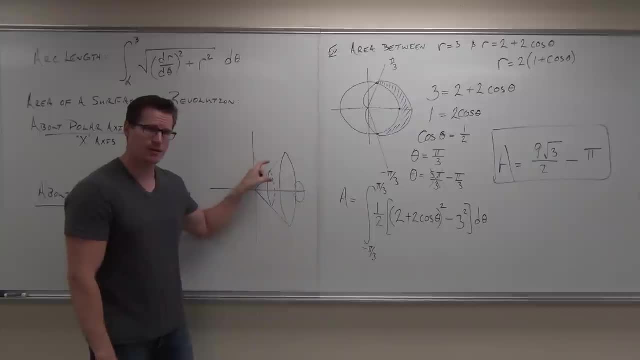 whatever my curve is, I'm going to need to know the height of it, Because what's happening here is, if you remember how this was and if you don't, you can watch Calculus 1,. I've explained how to do all of this at length and prove all of it. 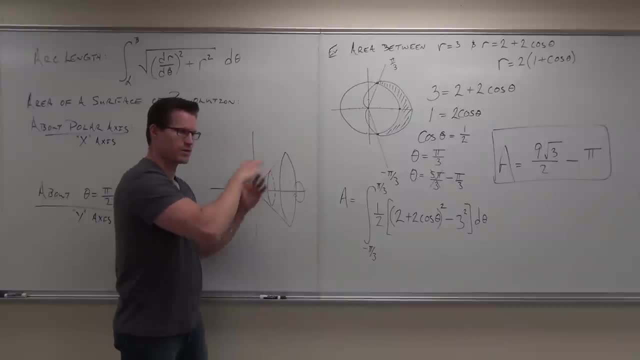 What happens is we take, we take little circles right and we find the circumference of each circle. And we find the circumference of each circle and integrate it about the length of the curve. So you say, hey, here, what's the circumference here? 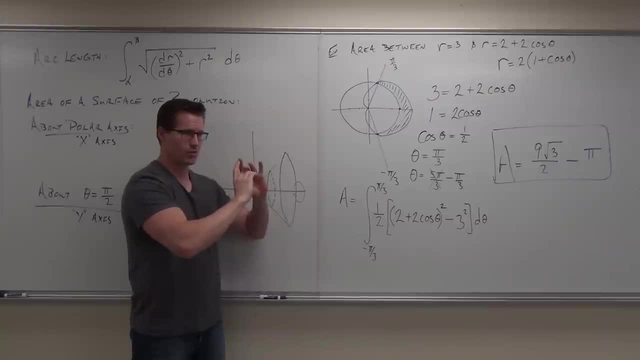 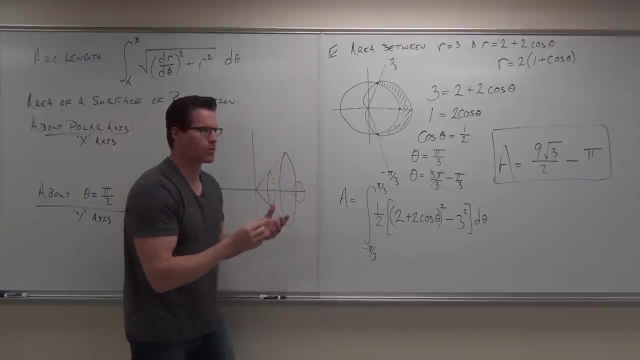 And the circumference is added together gives us our surface area. Now, of course, the circumference is multiplied by a little infinitesimal width, which is how we actually get to add them up. okay We go. that's our integration idea. it falls to the limit. 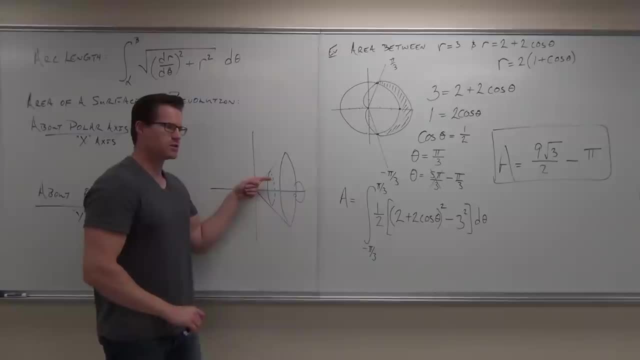 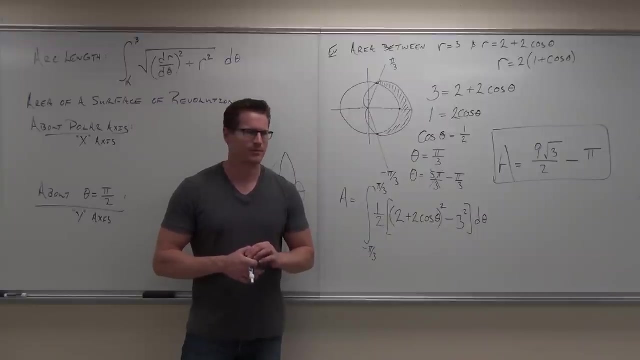 But this is the plan. The plan is: do circumference times length and then integrate. That's the whole idea. Circumference: what's the circumference of a circle? Oh good, what is it? 2r squared, 2r squared, yeah. 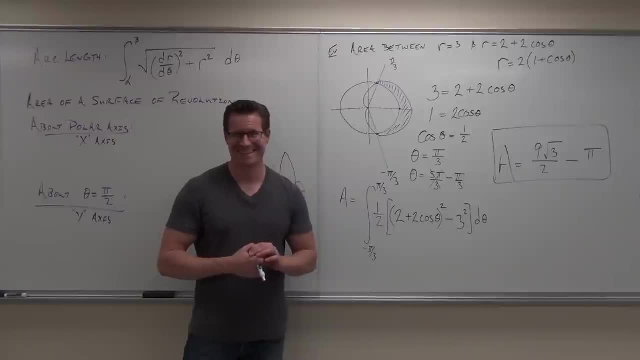 No, It involves a pi and an r. it's not squared. That would be, if you square a unit, do you understand you're going to get an area out of that. I'm looking for a circumference 2 pi r. 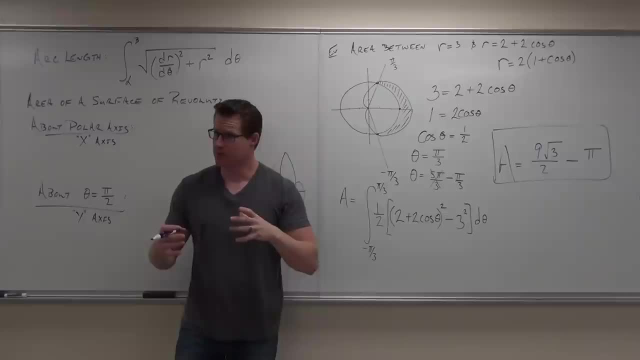 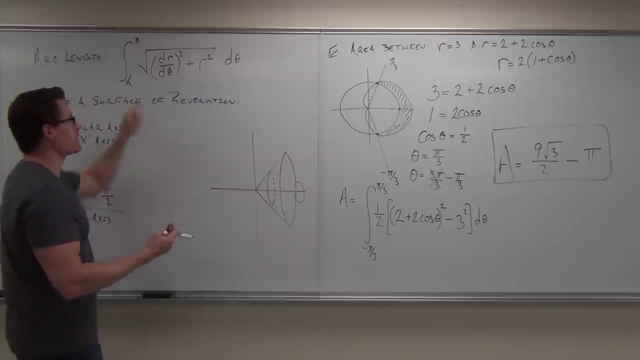 2 pi r. it's 2 pi r. So what I'm trying to do here is: take the circumference times the length. Listen, do we already have an expression for the length? Yes, Yes, that's the length. So all we're going to have to do about the x-axis is say: okay, well, here's alpha, here's beta. 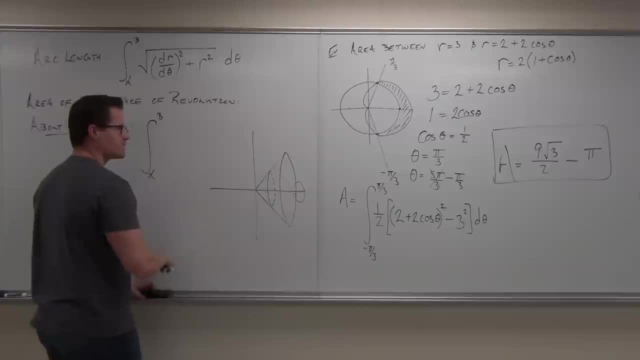 I'm going to do circumference times length. The length is going to be taken care of for us already. The length is this: It's dr d theta squared plus r squared, and then, of course, we're going to do d theta. 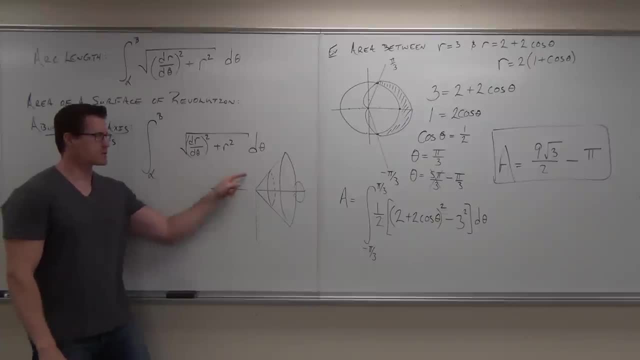 You guys all understand that's the length, right? Yes, Yes, So that's what we're talking about. So what I'm going to do is I'm going to do the circumference times length, because I'm just adding up all the little circumferences times, a little bit of width, giving us the 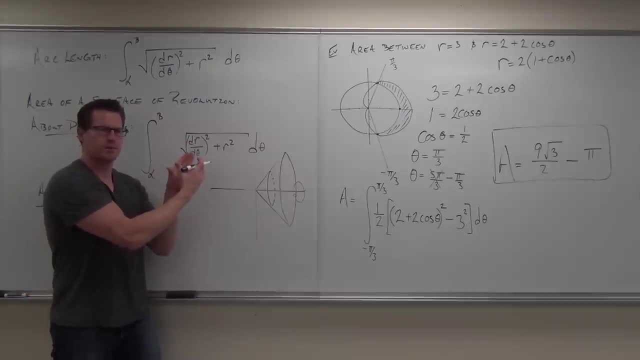 surface area of each little kind of. it's almost like a miniature cylinder and we allow that cylinder to change shapes. So it's 2 pi r. okay, wait a minute. 2 pi r, 2 pi. well, we don't really want r. 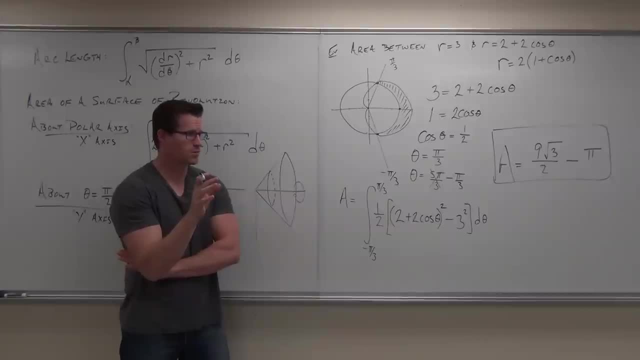 Let's not let our r's get confused here. r for polar equations, r for polar equations stands for this, this distance. here. what we want is the R, the radius of our little circles. what is this? if I have an xy axis, what's the radius of our circle? 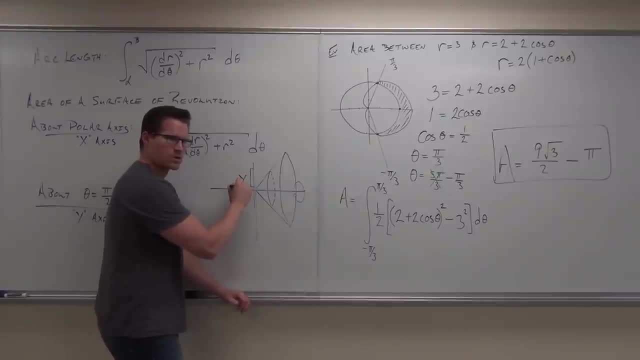 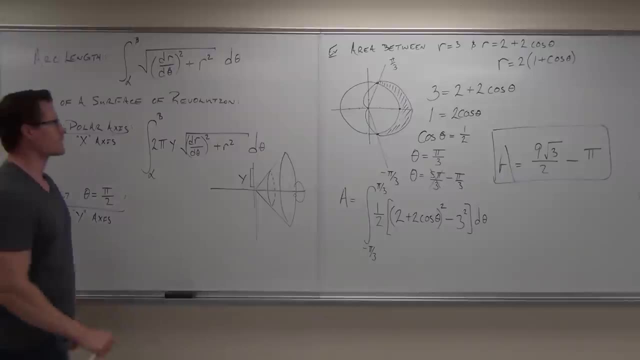 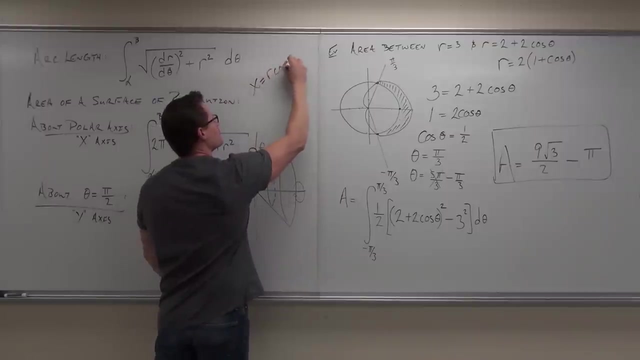 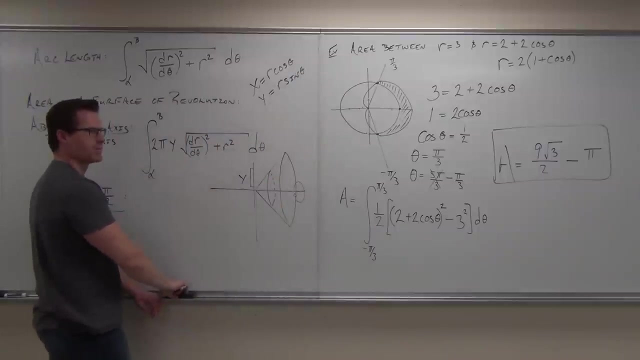 it's Y. it's Y only in terms of us. we're back at the very beginning of polar equations. we had two definitions. we said X was equal to R cosine theta and Y was equal to R sine theta. so, instead of Y, what am I going to put here? also, I'm going to move this 2 pi. 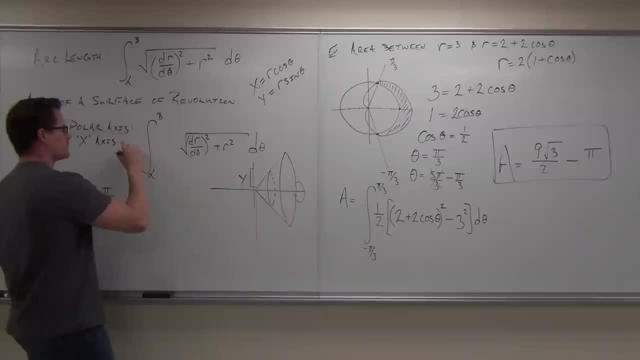 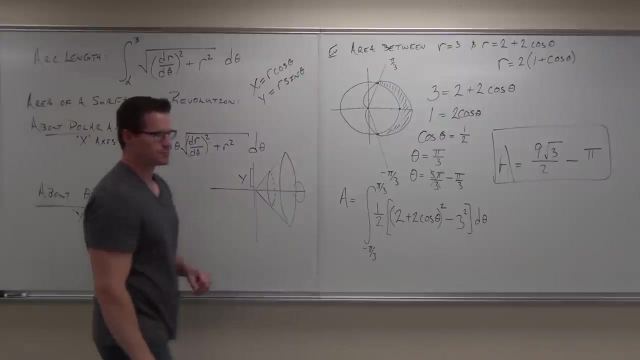 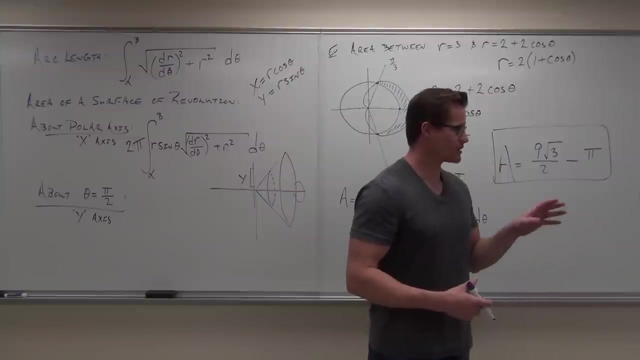 out front now I'm not going to give you an example of how to do this. I'm hoping that you can figure out that it's a formula. so let's look at this for a second. you already told me that you guys could find length right. so if I actually find the surface, 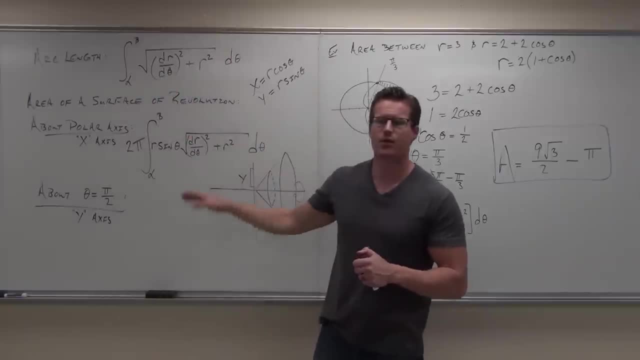 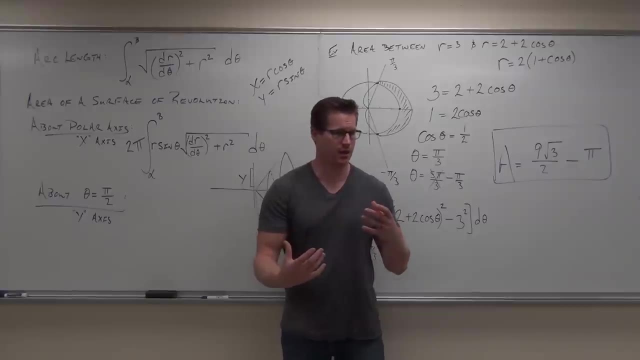 area, revolution about the polar axis, the x-axis. think about what this means. all I want to do is find the circumference times, the length. did you guys see that this is circumference times length here? look at this. here's 2 pi R. well, the R in that the R is. 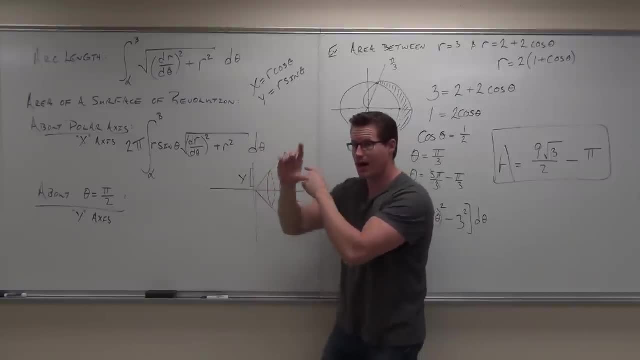 the Y height because I'm going around the x-axis, the height of my circle. the radius of my circle is just my Y. my Y component Y is R sine theta. so we have 2 pi radius. the radius is R sine theta because that is the height of my Y. quick. 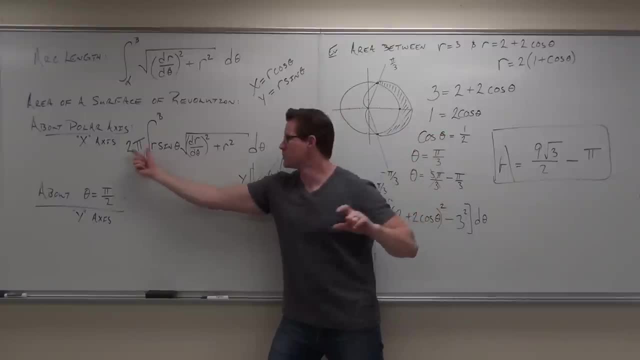 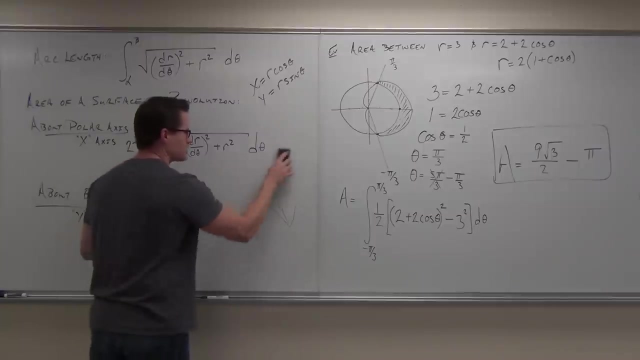 head, not, if you understand, that's the most tricky part here. do you guys get that part? so circumference 2 pi off, radius Y, times, length, hey, link, and then we integrate that. now can you tell me what the only difference is between, the only difference between this and this is going to be? what do you think? say what? 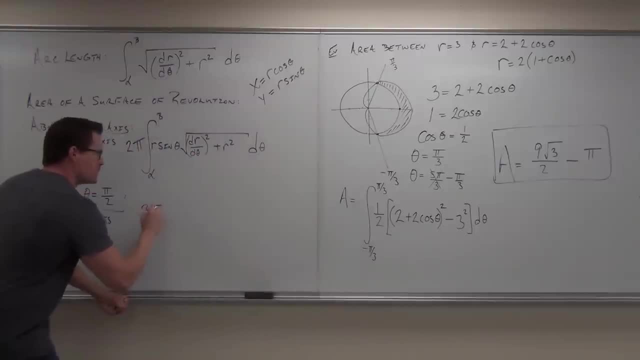 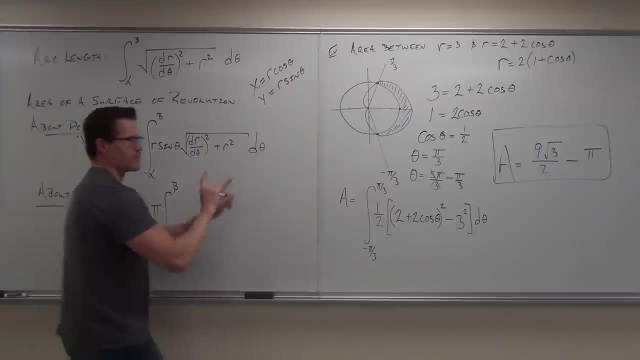 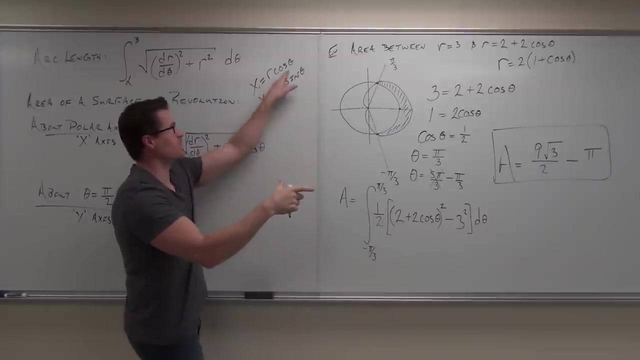 now that's right, why? I mean it's okay because why? that's confusing. but yeah, that's right. so if I was going around the y-axis this way, so around the y-axis, then my radius is going to be the X component, since X is R cosine theta we. 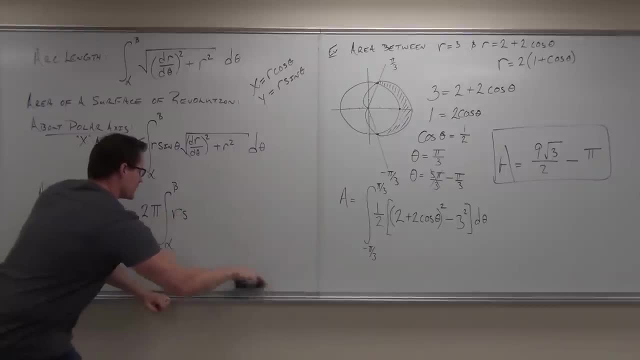 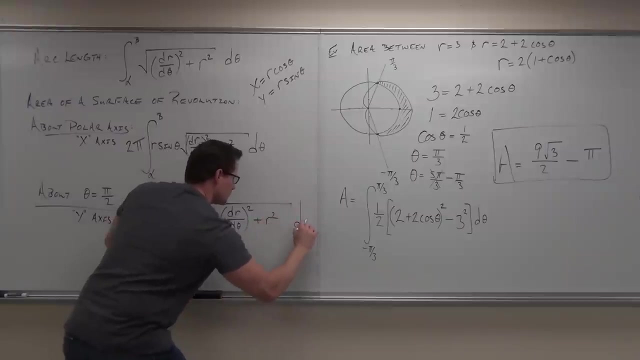 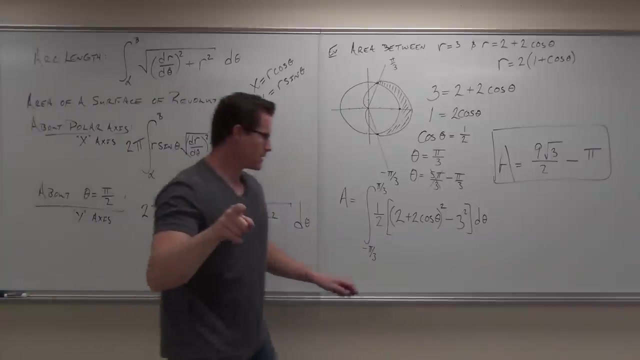 have 2 pi radius or X cosine, theta, and then we have, because it's polar, and X and Y don't assist in polar, right with it. still, you take your X component and your Y component and say, well, you know what, if I'm trying to figure out how, what my radius is, 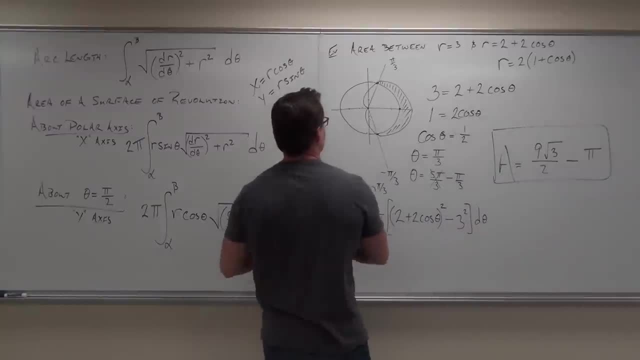 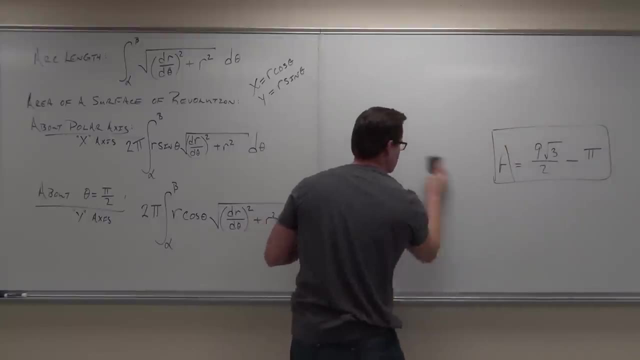 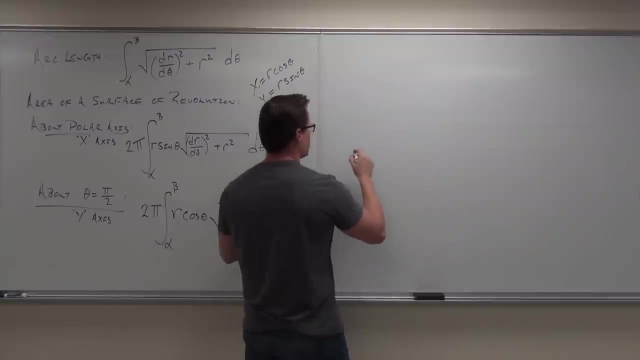 so a polar curve would look at. you know what polar curve. even if I have just like this, just an arc, if I want to revolve, that I need an X component, a Y component, and whether go to run X axis or Y axis. so if I said, all right, I want to involve that, 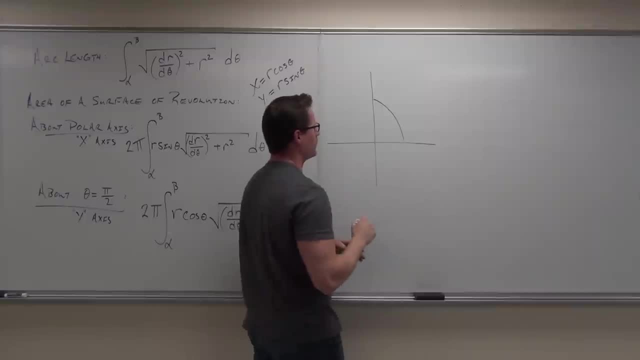 just something simple like that one. if I want to revolve that this way, I need to find out the radius of the circle it's going to make. so this is going to make some sort of a circle right where I want to find out my radius. the radius is just. 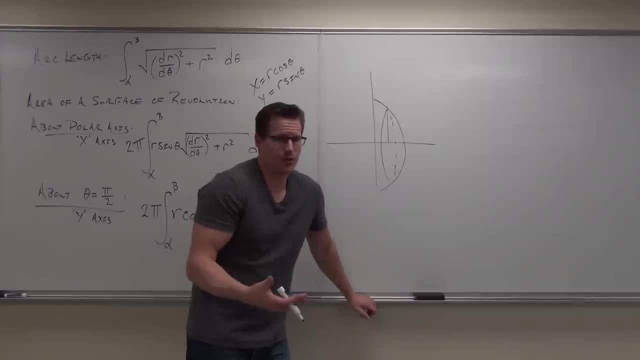 the Y component. so what we need to do is basically convert a polar equation into, Well, kind of think it through, Think instead of polar, let's think xy, because I'm going around kind of the x-axis, the polar axis. I just want my component, my y-component. 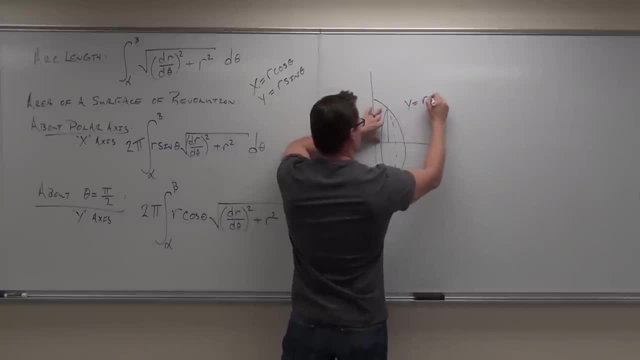 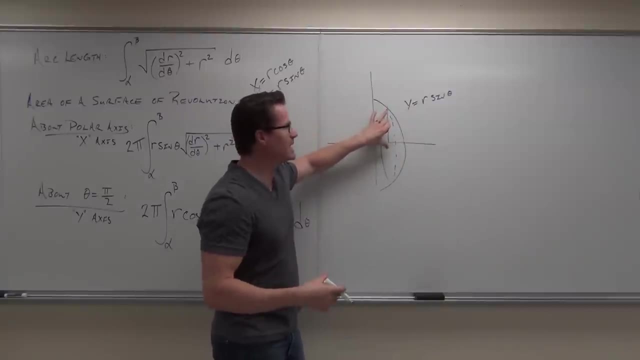 because my y-component is my height. So if my y equals r sine theta, then I have two pi. radius is two pi y. Y is my radius. but I need it also in the form of a polar equation. That's where I get our r sine theta from. 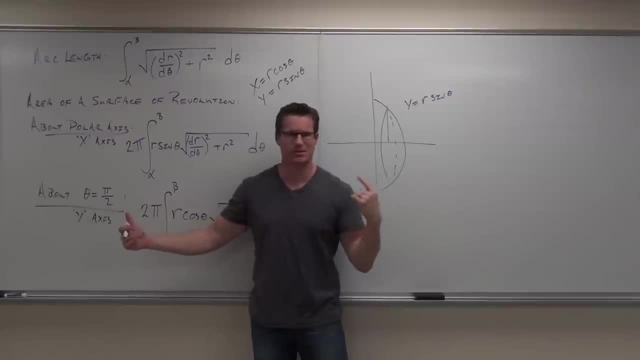 And in the x around the y-axis it's x instead of y, And so we get our r cosine theta. The length length is easy. Length is what we had before, So it's circumference times length. That's basically the idea in a nutshell. 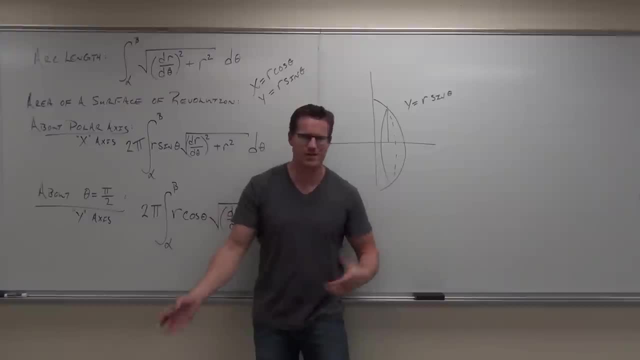 I mean, I would like to prove it but I obviously don't have time, and I've proved it before this idea before in calculus one, so you can always go back and watch that Show of hands if you understand the concept of this one. 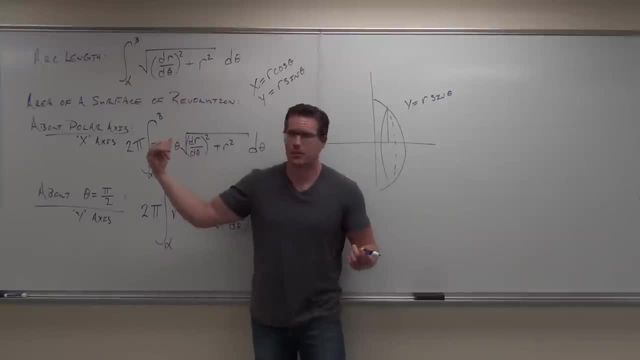 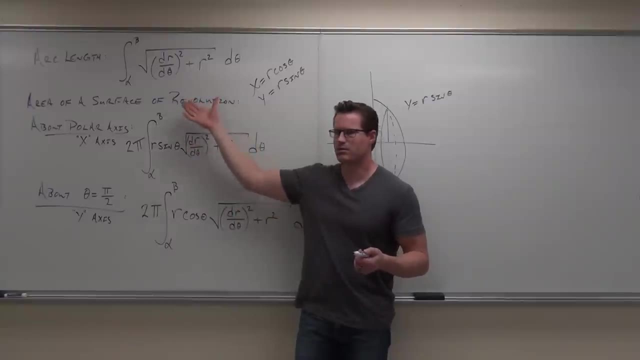 So if I had to do this, could you plug in the appropriate things? Yeah, we could find r, not a problem. Take your r multiplied by sine theta. Take dr d theta, no problem, it's just your length. So dr d theta, squared r squared. 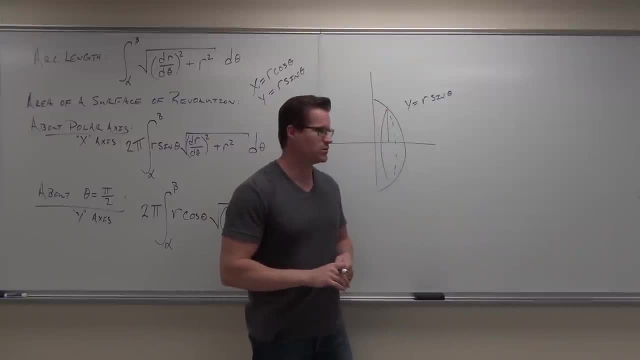 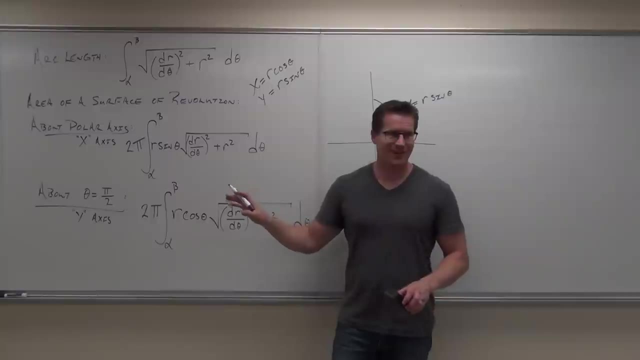 and then it might be nasty, but you do know how to do those things. Now I want to cover one last, unless there's any other questions any more at all with this, You sure? Okay, one more. I want to show you this example. 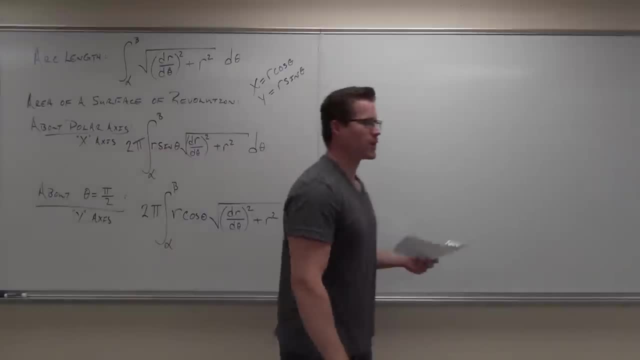 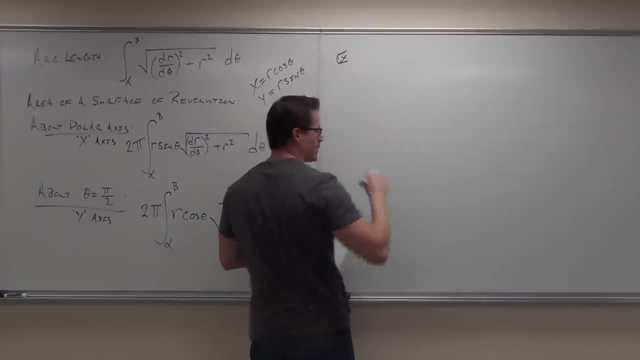 because interesting things happen when you try to find the intersection between two polar curves. I'll show you that right now. So what we're going to do is: we're going to find out without having to graph this. we're going to find out. 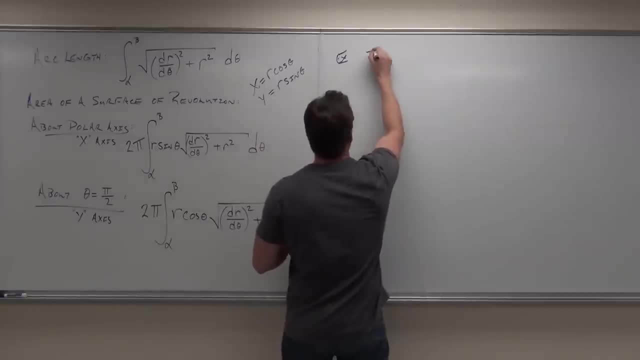 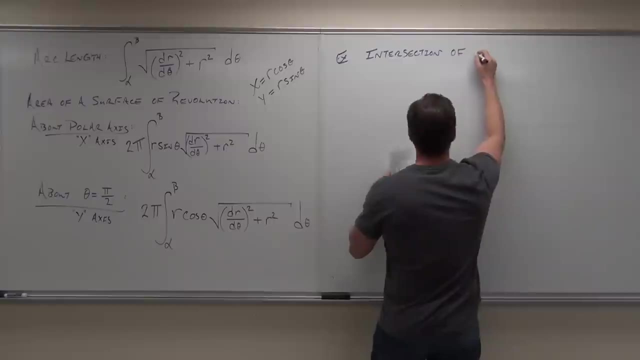 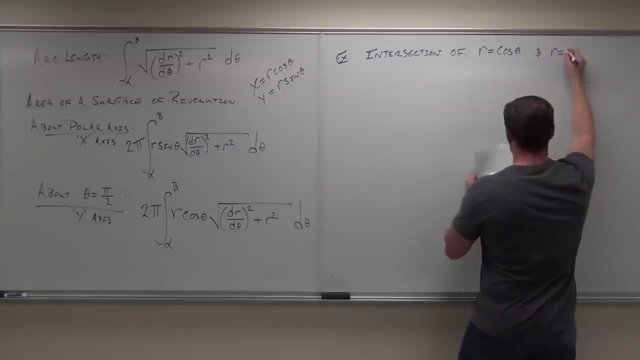 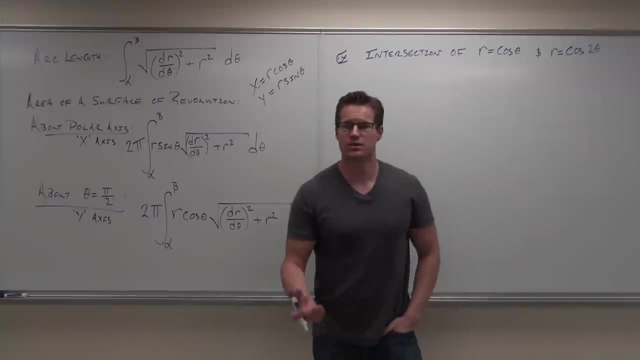 So what we're going to do is we're going to find out, without having to graph this, where these things intersect. So r equals cosine theta, r equals cosine two theta. where are these going to intersect? I don't know what these things look like. 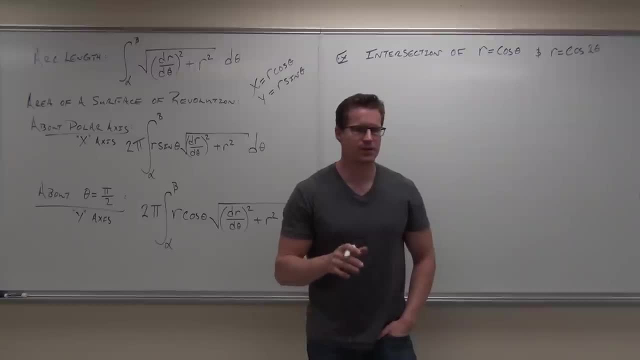 or at least let's pretend I don't know what these things look like. Let's try to find out the intersection Now. ladies and gentlemen, I asked you this already today: How do you find out where any two curves intersect, Provided they're solved for your variable? 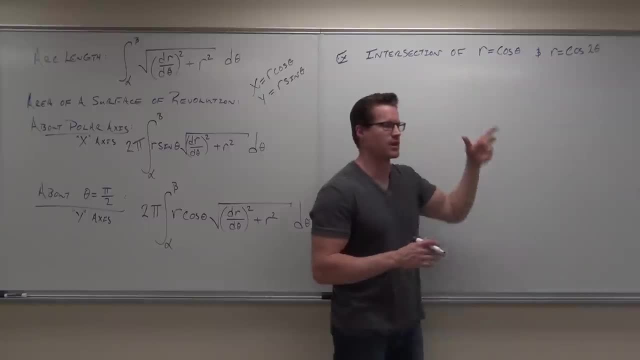 your dependent variable, r, provided it's not like an r squared or something. yes, just set them equal. So r equals cosine theta and r equals cosine two theta. if I want to find out where they intersect, I just set them equal and I try to solve for theta. 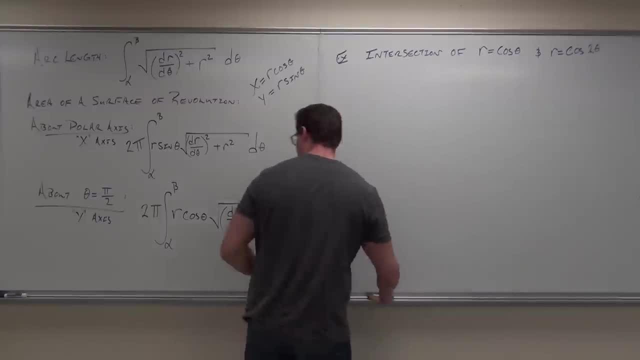 Are you listening? Are you listening still? Okay, so let's do that. Let's set them equal to try to find the intersection. Now, where in the world is cosine theta going to equal cosine two theta Without having to think a whole bunch of stuff here? 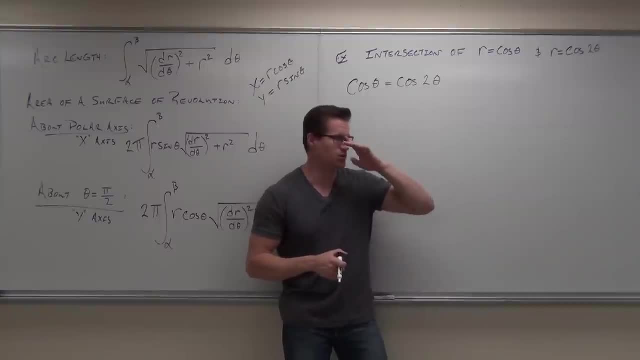 well- and we're going to come back to this in about three, four minutes too- Without having to do that, let's use some identities and maybe come up with an equation that we can use. The one thing I don't like. I don't like how that's. 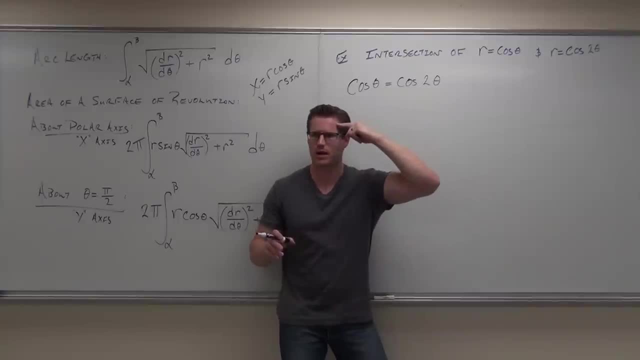 that's theta and that's two theta, because that's causing my brain some trouble right now. So let's change this one. So I'm going to do cosine theta and I'm going to use that formula that we often use in, but we're going to use it in reverse. 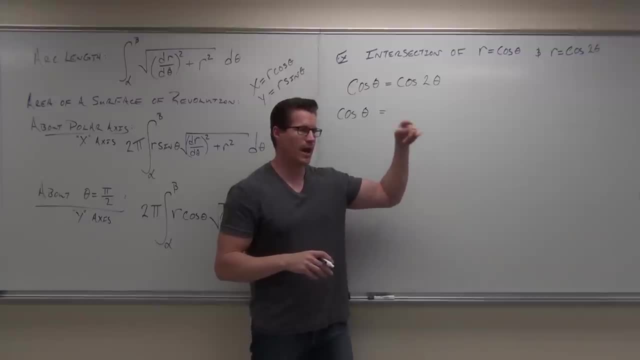 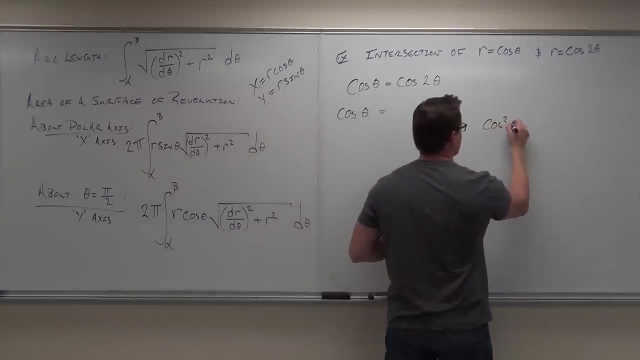 Remember how cosine squared theta equals one half one plus cosine two theta. Well, what that means is that we can do that in reverse. so let's see: cosine squared theta equals one half one plus cosine two theta. If we solve that for cosine two theta. 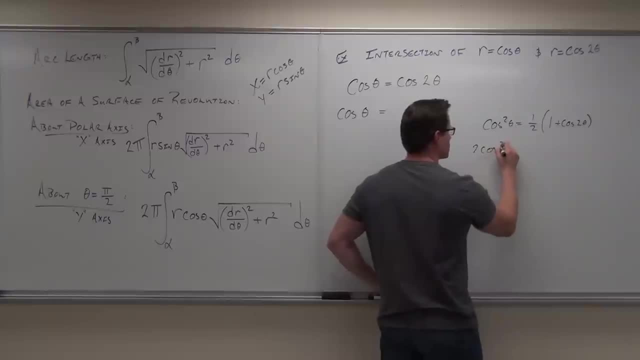 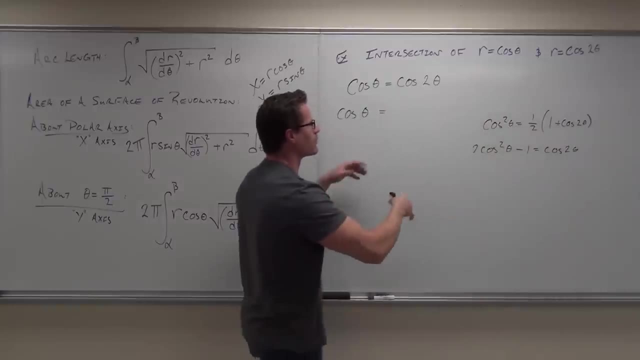 then we get two: cosine squared theta minus one equals cosine two theta. Does that make sense to you? We just solved that. we used that in reverse. So this therefore equals cosine two times cosine squared theta minus one. Now, if you don't see it, I don't blame you. 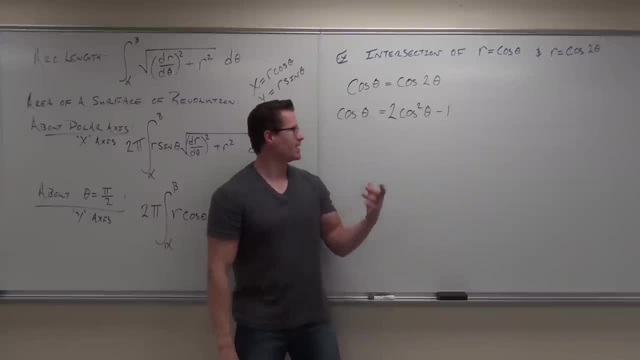 but do you see? do you see? this is kind of cool. This is actually a quadratic equation, do you see it? We get something squared. we get the same something not being squared. that's why we wanted to stay away from sines and stuff. we want to make them all cosines. 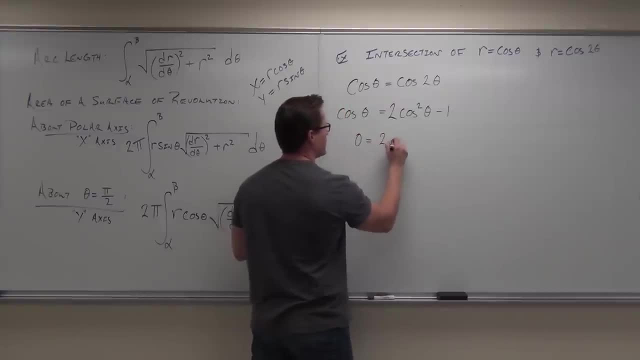 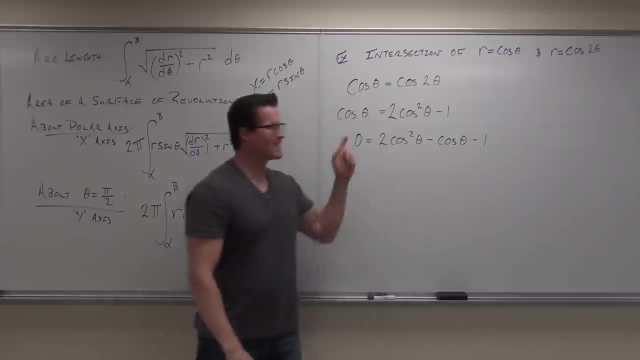 because right now, if I solve this for zero on one side, I can get that. Now what's interesting is this is still factorable, just like anything else. It'd be like doing: zero equals two x squared minus x minus one. 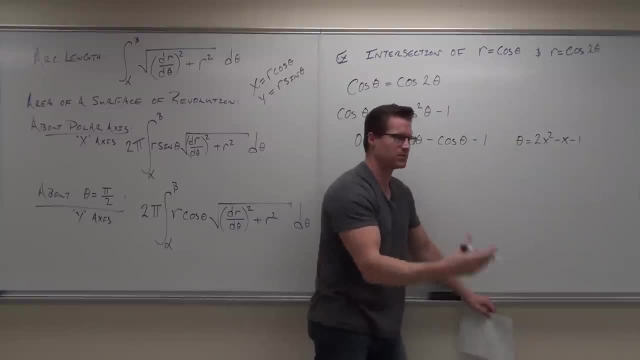 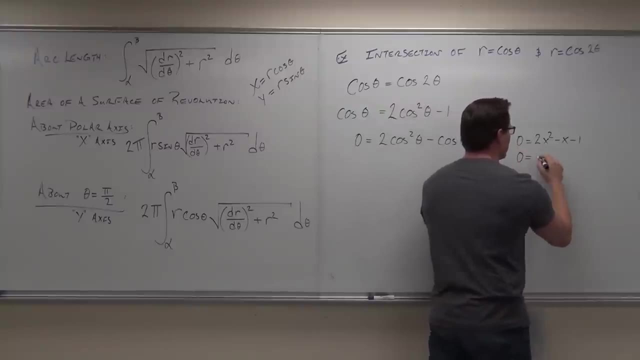 In fact you can do that. Just call that x for now. factor it, put your cosine back in. So if you factored it, not theta, sorry zero, Because I just got in the habit of it. Two x, what is it? 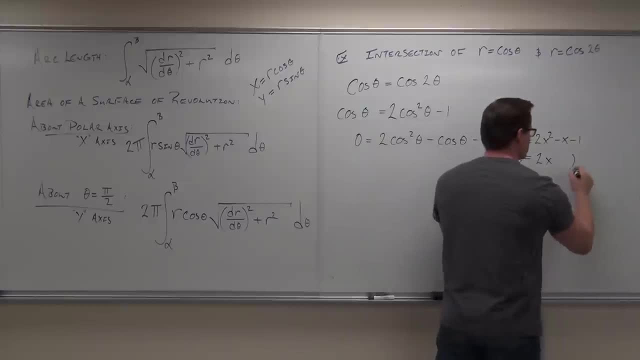 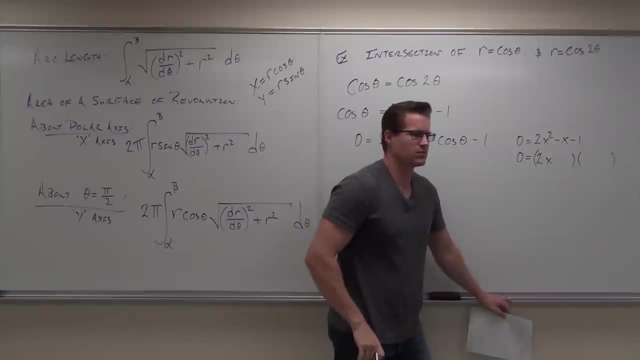 Two x. Do you know it? I'm pretty sure it's that, but you can double check. That would give us two x squared minus two x plus x. that's minus x and then minus one. Can you verify that? that's the correct one? 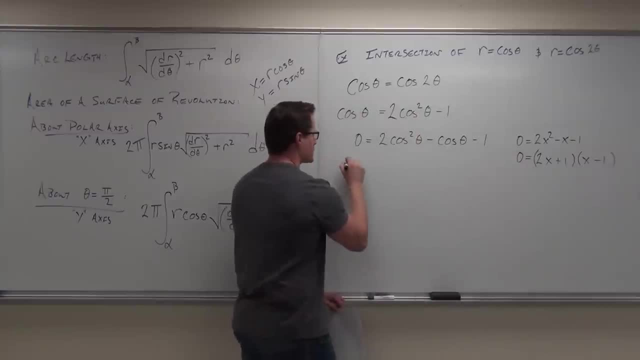 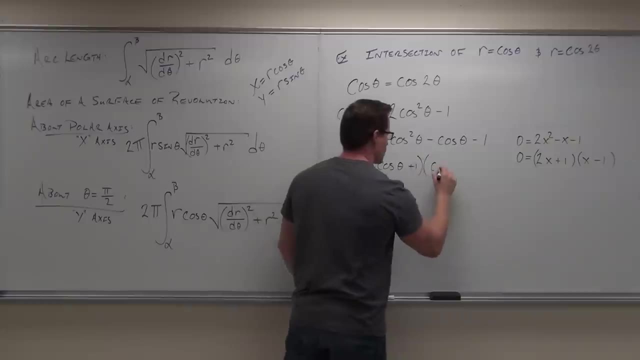 Okay. Well, now that we have cosines instead of x's, we get. zero equals two cosine theta plus one times cosine theta minus one, Just from our basic factoring. Now what's interesting is that the zero product property that always works for us. 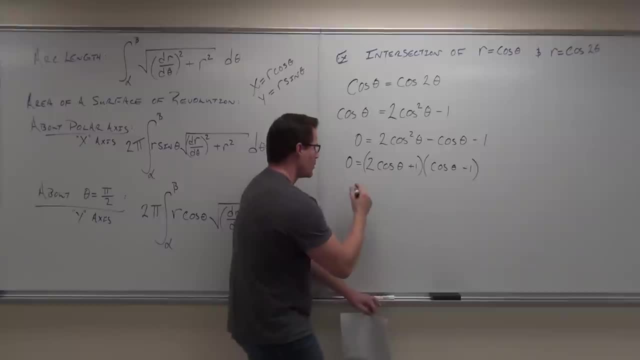 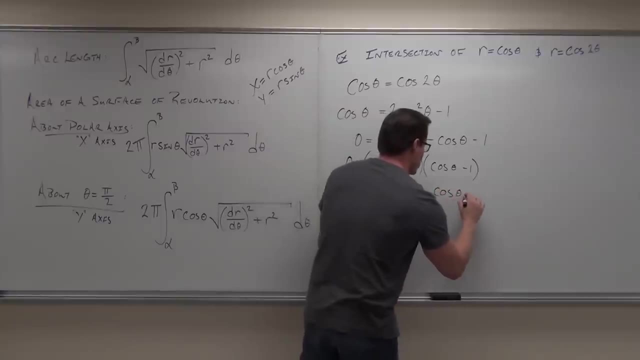 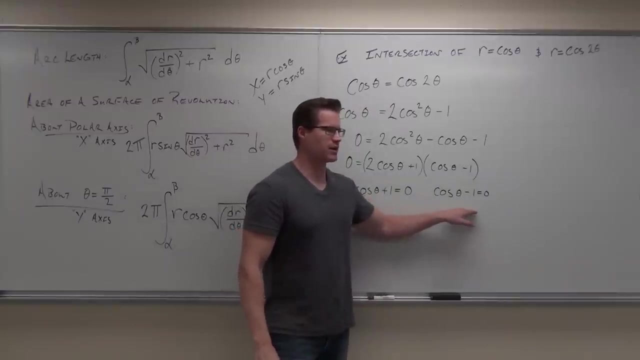 So if we have a product, and we have that product equal to zero, what that says is that each of those factors has to equal zero. Let's deal with this one first, because it's gonna be a little bit easier for us all, right. 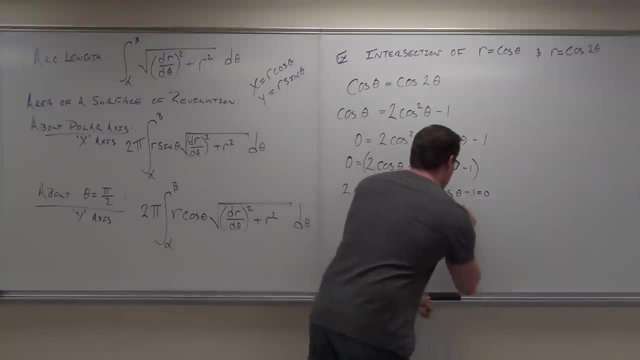 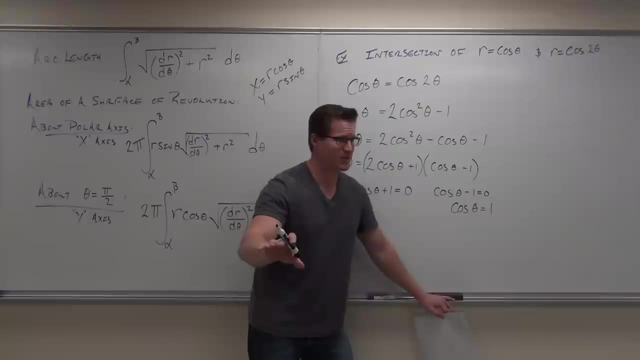 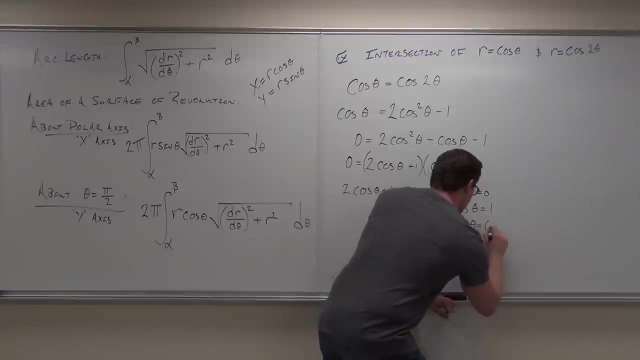 Let's solve that. How would I solve it? Cosine theta equals one. Now this one's easy. okay, Cosine theta equals one. You tell me right now, if cosine theta equals one, how much is theta Zero? 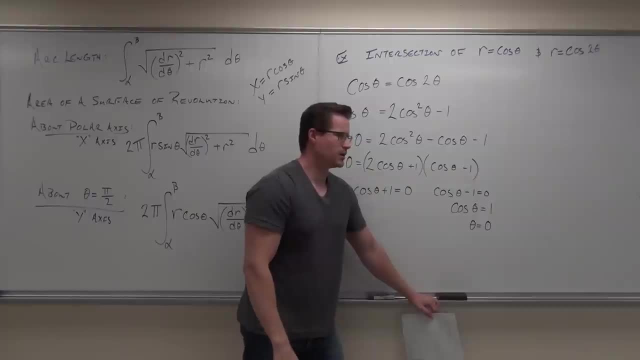 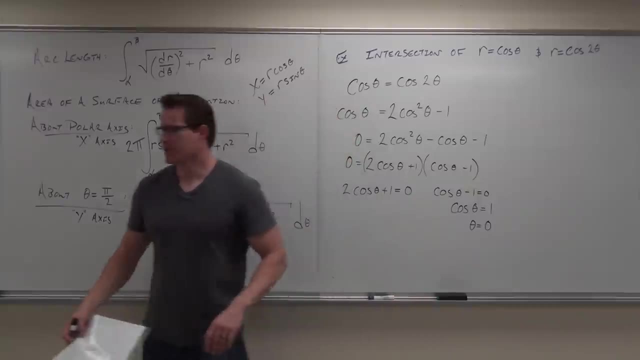 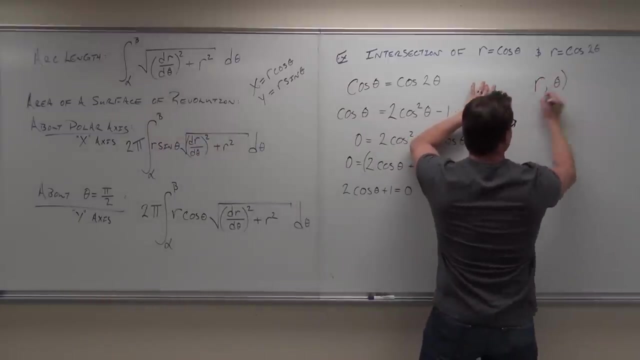 Very good, Zero, You with me? Okay, now think about this for two. Look back at our original equation. Do you remember? we want points, right, We want intersection points. Intersection points look like this. They look like R thetas. 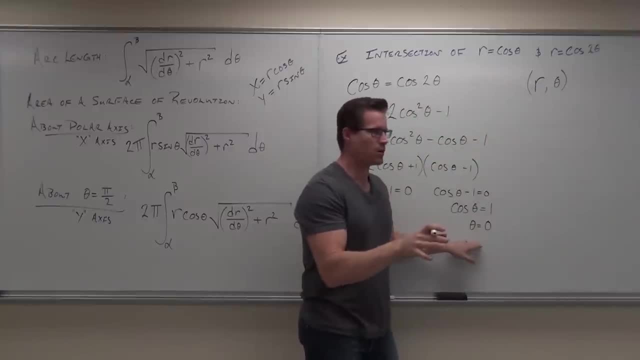 You get me. We now have a theta, We need an R. This is gonna be an easy one, but do you understand that we're not done right here, We just have? this is like saying, hey, find out where the lines intersect. 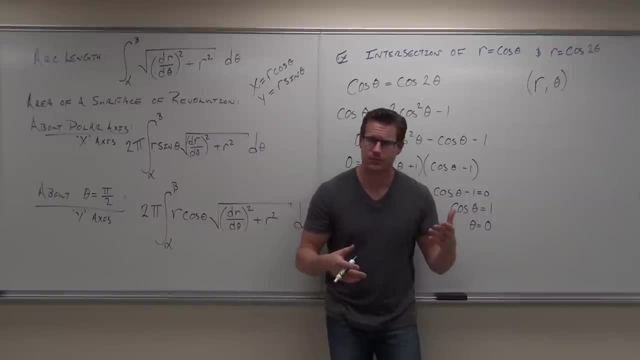 And you say they intersect at x equals three. Does that give me a point? No, it tells me somewhere in infinity, at x equals three, they're gonna intersect. I don't want that. I wanna know the angle and how far out to go. 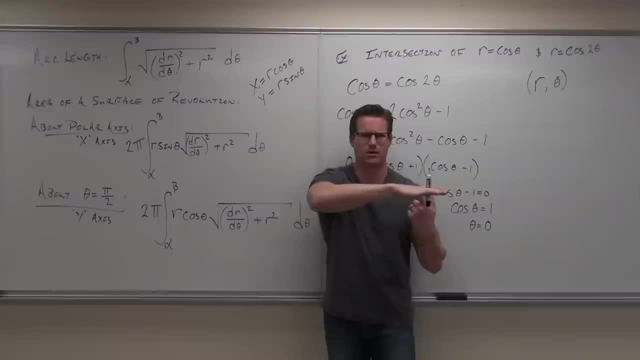 I don't want. hey, they intersect at theta equals zero, Cool. where That doesn't help me at all, I wanna know where I don't want a point. Do you get the point? Okay, so zero. Now look at this. 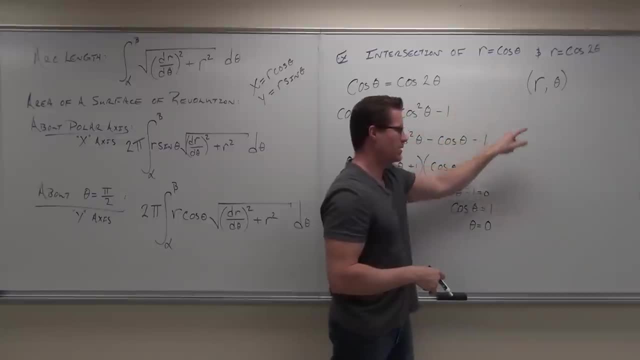 If R equals cosine theta, look down here: How much is cosine theta equal One, How much is R equal then One Cosine theta equals one. therefore, R equals one. So from here, R equals one. We now have a point. 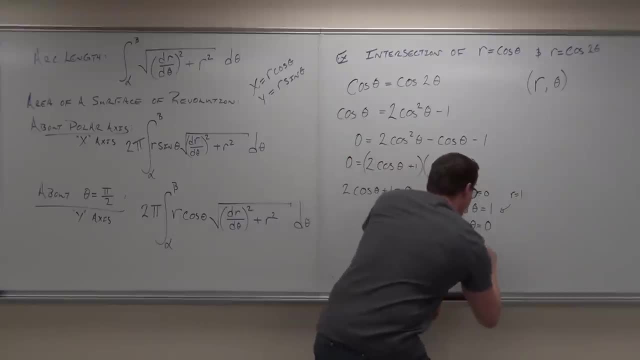 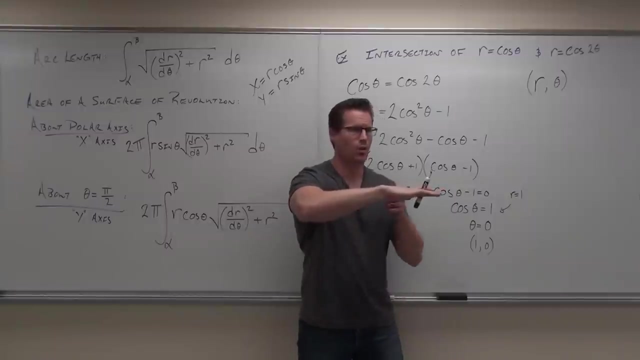 We have a point: Which one comes first, the R or the theta R, So one zero. These are gonna intersect at the polar coordinates, The coordinates of one and zero, R of one and angle of zero. So it says, hey, angle zero, go out one. 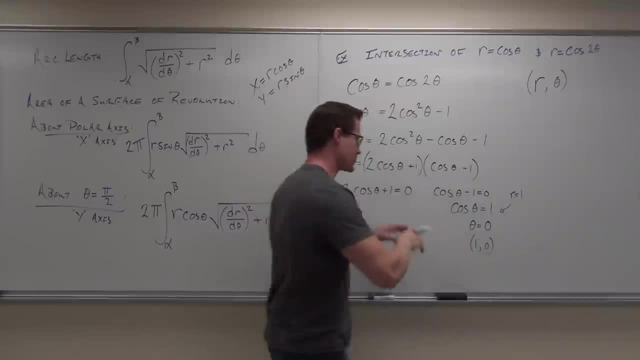 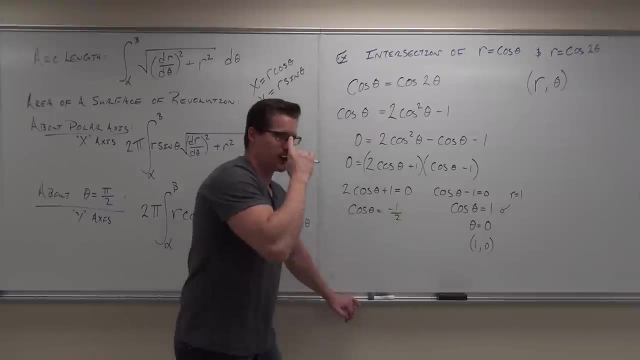 these things are gonna intersect right there. So it means we understand that one. Okay, now let's work on this one real quick. Do you understand that here we're gonna have cosine theta equals negative 1 half? yes, No, Okay, if cosine theta equals negative 1 half. 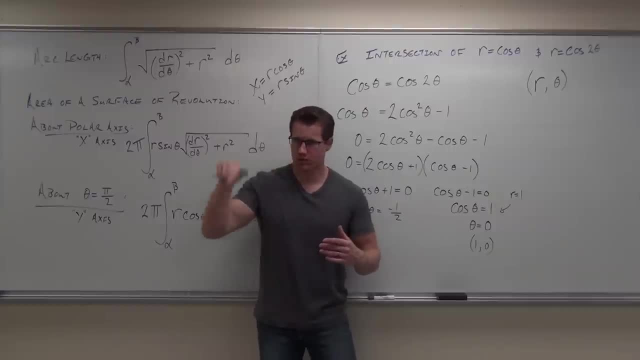 cosine is negative in quadrants Two and three. Two and three very good. So cosine's 1 half where Right here Pi over 3, so if it's a pi over 3 for 1 half, it's going to be 2 pi over 3 for negative 1 half and 4 pi over 3 for negative 1 half. 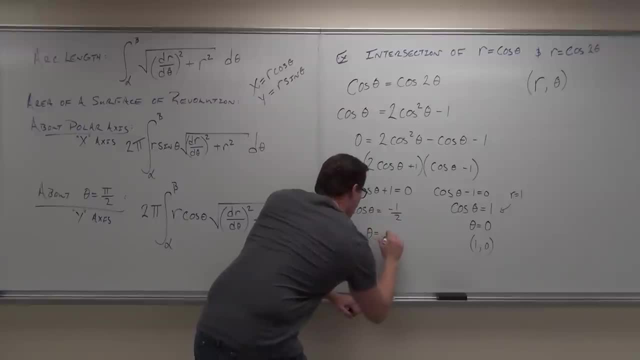 So these thetas are 2 pi over 3, you can check your unit circle if you want- and 4 pi over 3.. So can't you feel okay with that one, Are you sure? Now is my r going to be 1 for these points as well? What's my r? 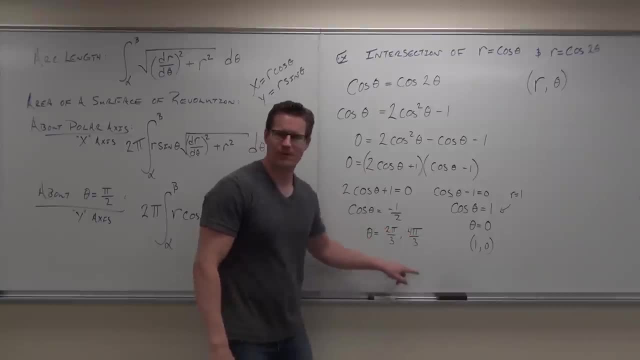 Look up here what's my r. You got it. Cosine theta equals r. yeah, So if cosine theta equals negative 1 half, that means r equals negative 1 half, And so we get two points here, but they're both going to have the same r. 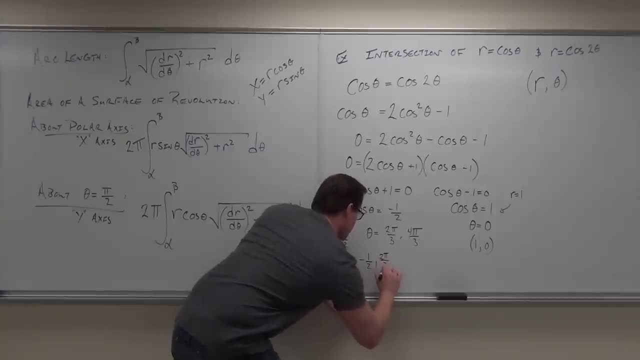 We get negative 1 half of 2 pi over 3.. And we get negative 1 half 4 pi over 3.. What I want to know is: does that make sense to you? Show of hands. if it does, you're like, okay, that makes sense. 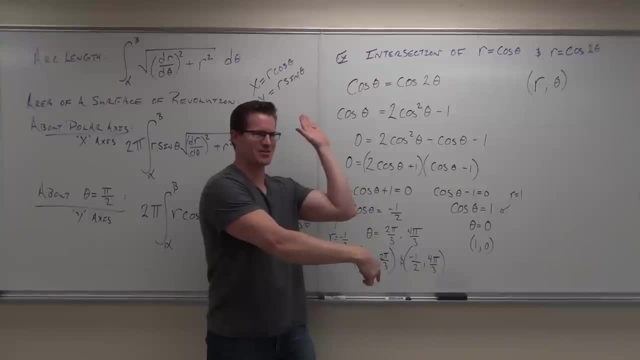 These are weird. yeah, because you have to go 2 pi over 3, but then go negative 1 half, alright, so it's in quadrant 4.. And this one says you go 4 pi over 3, you can't even do that. 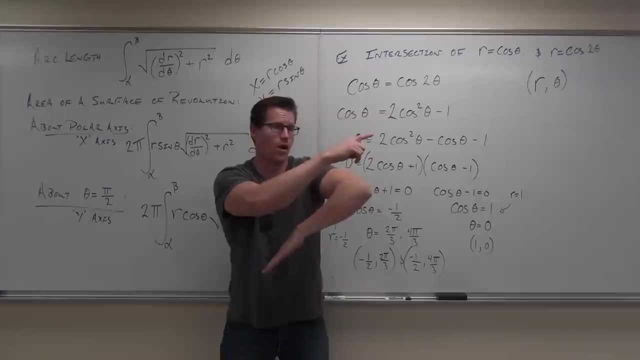 And that's negative. so it's in quadrant 1, actually, But that's what those intersections are. This is right on the polar axis. Do you guys feel okay with that one? So, use an identity, find an equation, solve it. then just don't forget that you need to find your r. 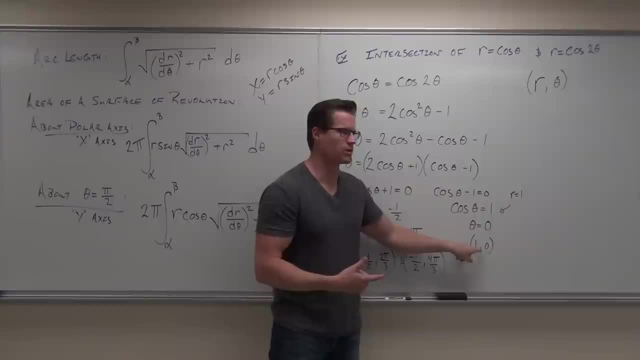 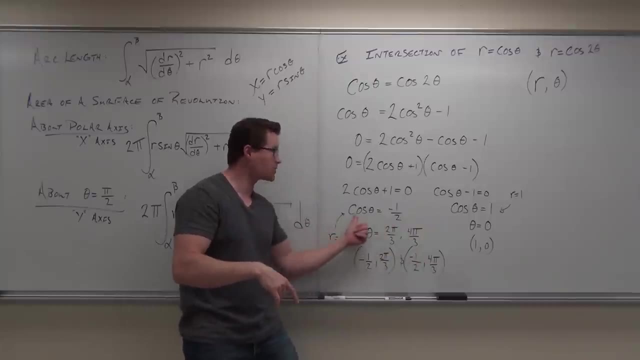 You don't just give me thetas here. Theta is 0,, sure, but r is 1,, so 1, 0.. Theta is 2 pi over 3 and 4 pi over 3, but that also, they both work with the r cosine. theta is r of negative 1 half. 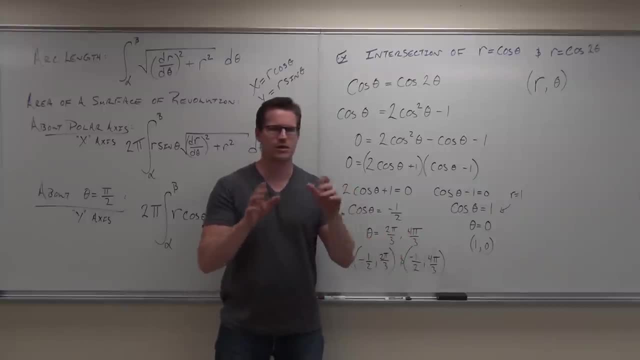 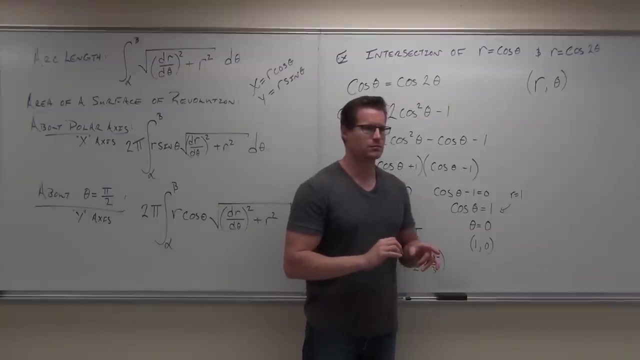 So we have negative 1 half 2 pi over 3 and negative 1 half 4 pi over 3.. Now the last bit. this was not that interesting. This is what makes it interesting. You ready? Plug in cosine of pi over 2.. 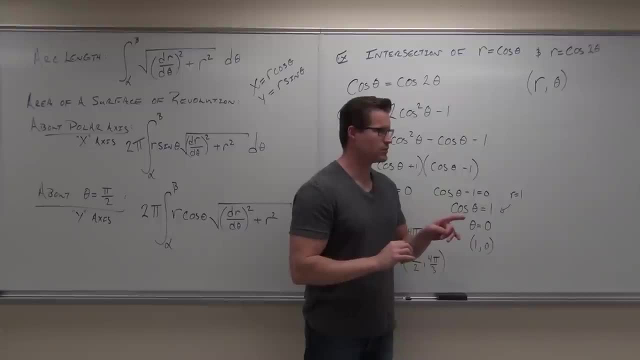 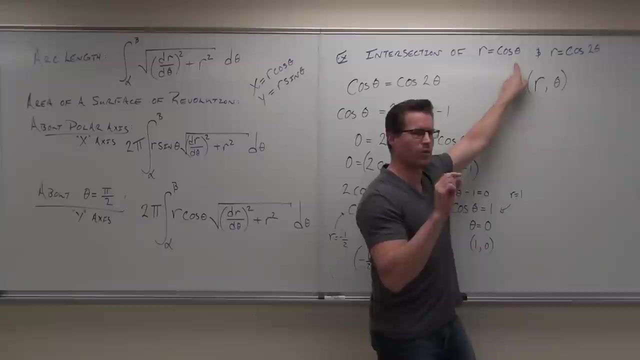 What's cosine of pi over 2? 0.. What's cosine of 3 pi over 2?? Good, now I'm supposed to sleep for a little bit. Do pi over 4.. So that was for this one. Do you understand that you are going to have an r of 0.. Do you get that point? 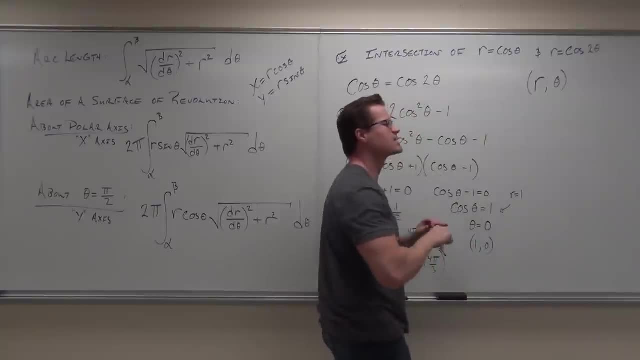 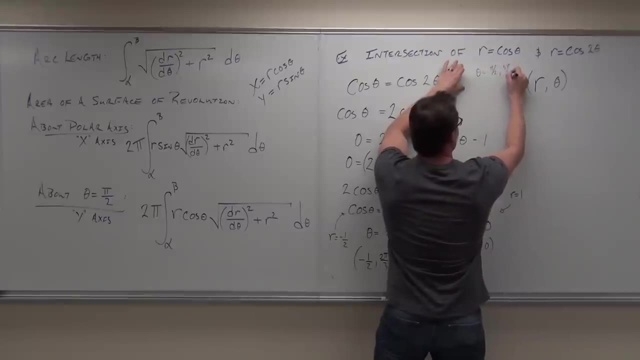 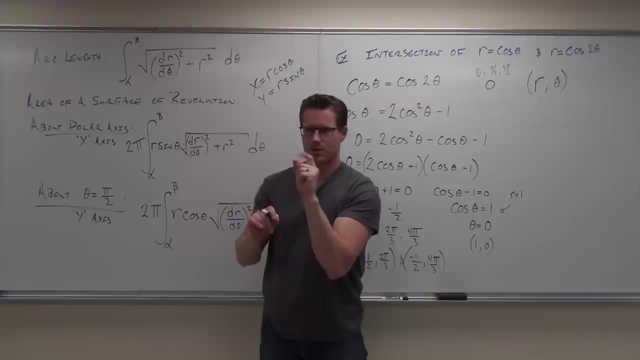 So if I plug in, so this is kind of a, this is the interesting part. So if I do theta equals pi over 2 or 3 pi over 2, I get 0. That means I'm going through the pole, I'm going through the origin You follow. 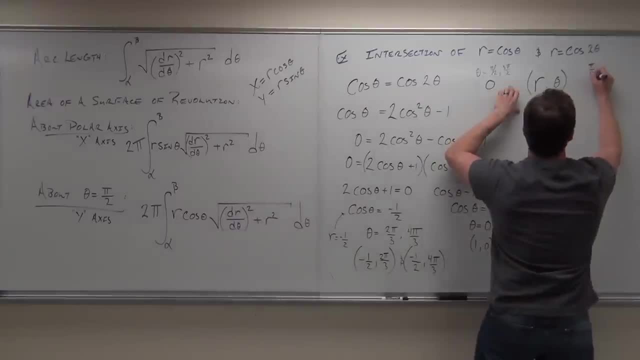 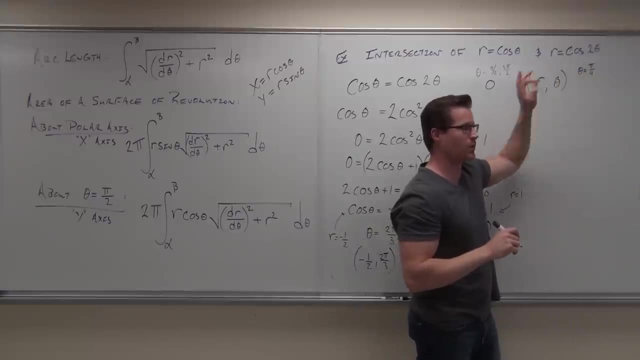 Do this: Plug in pi over 4. here It's 2 times pi over 4.. What's our r Weird? okay, Plug in 3 pi over 4.. 3 pi over 4 times 2 is 3 pi over 2.. 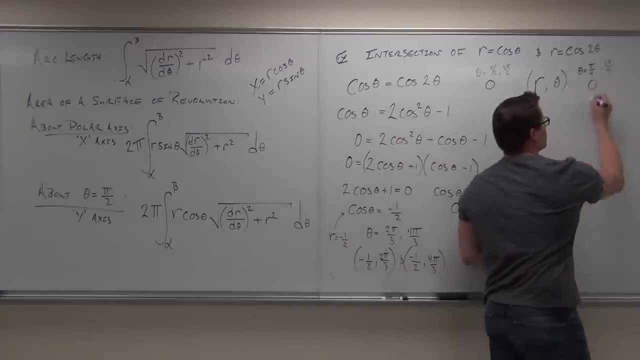 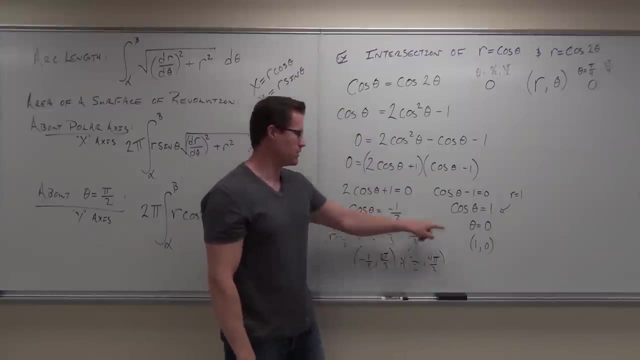 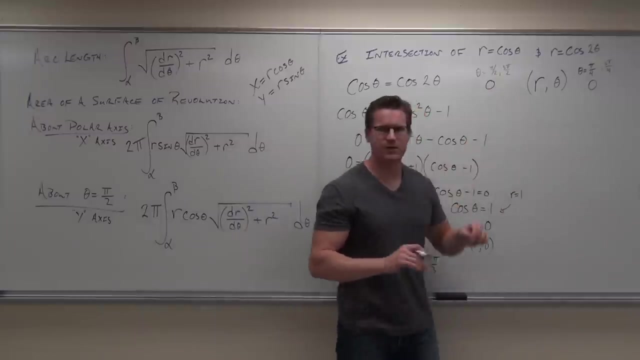 What's cosine of 3 pi over 2? I get 0 here. Did we have an intersection of r equals 0 anywhere up here? No, This said r equals 1.. This said r equals negative 1 half. Yet we know for sure that both of these curves are going to go through the origin at some point. 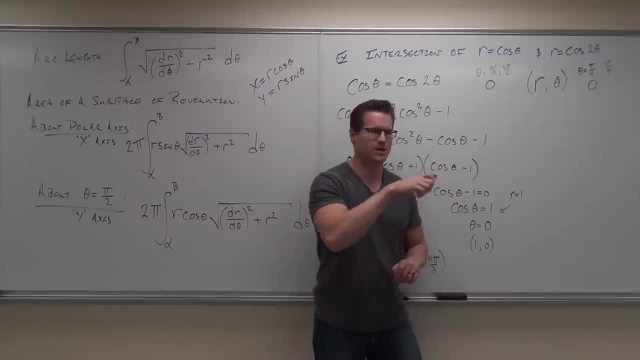 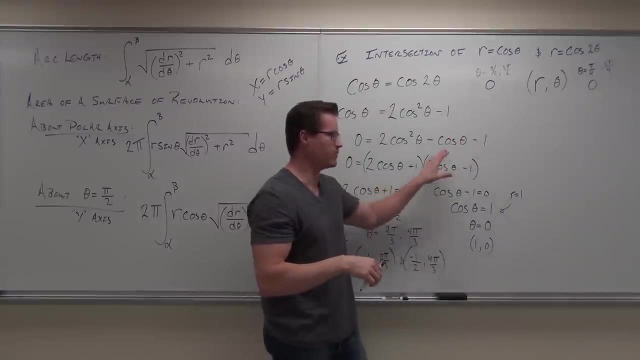 Do you get that? Why it doesn't show up is because they go through the origin at different times. So what's weird about these polar curves is that even if you solve it all the way down- we don't make any mistakes here- you can still go through the same point, but at different times. 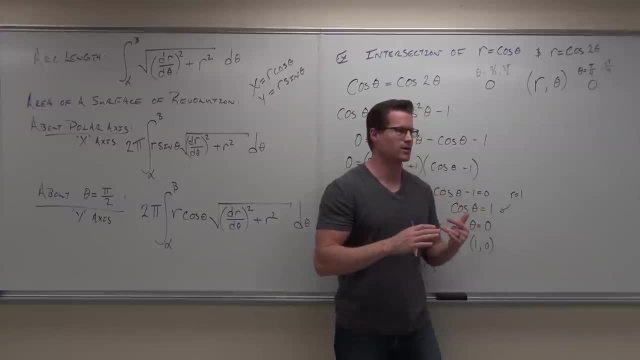 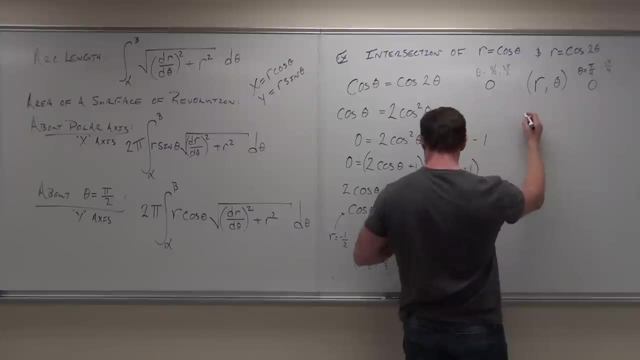 So the angles aren't the same when they hit that point, Because here we're multiplying those angles times 2.. That's what's weird. So we do have another intersection. So one more intersection. Intersection happens at negative 1, half 2 pi over 3.. 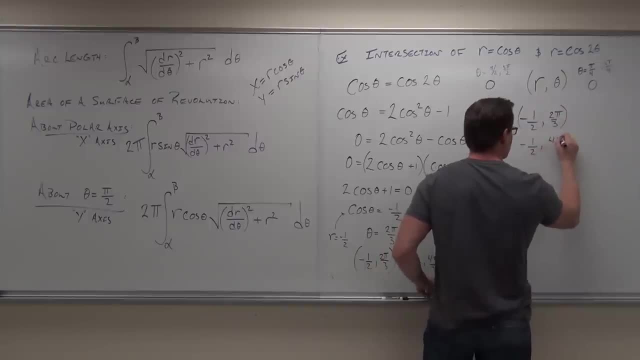 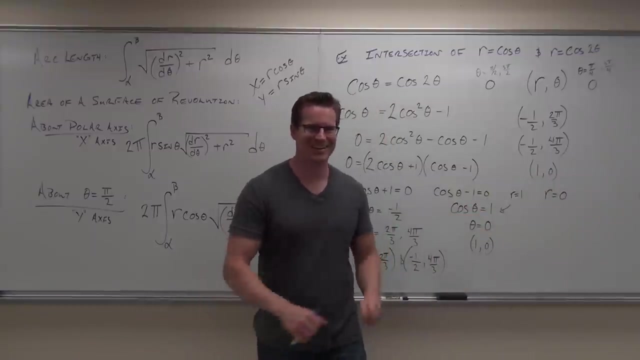 Intersection happens at negative: 1 half 4 pi over 3.. Intersection happens at 1, 0.. Intersection also happens at r equals 0. Because they're both going through the origin, right there? Isn't that interesting. That's kind of cool, right Weird. just different times.